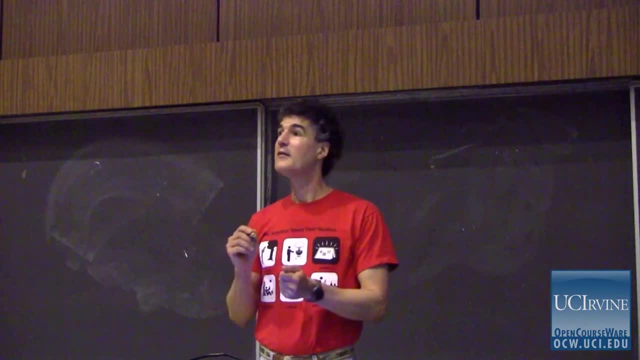 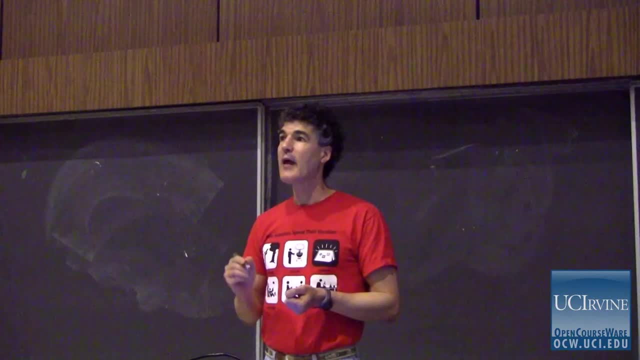 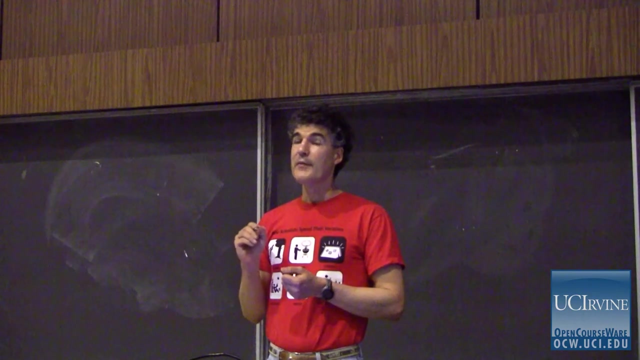 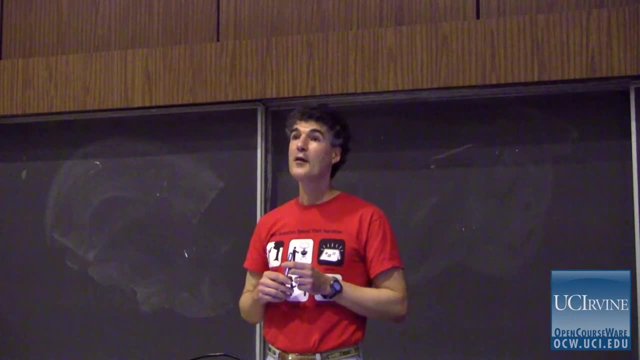 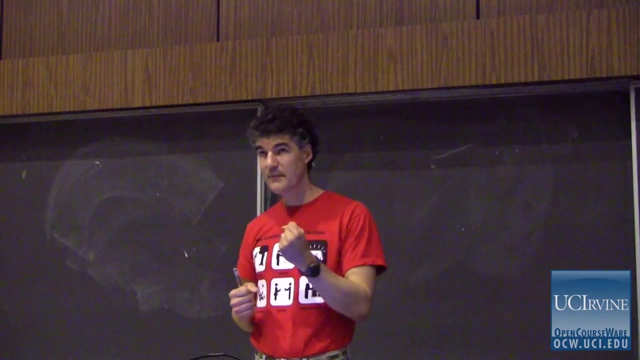 That's the only cure for that. Learning is a chemical reaction. You have to drive it with your force of will or it doesn't happen. You don't get stronger for no reason, or by lifting a feather or, in fact, by doing anything. 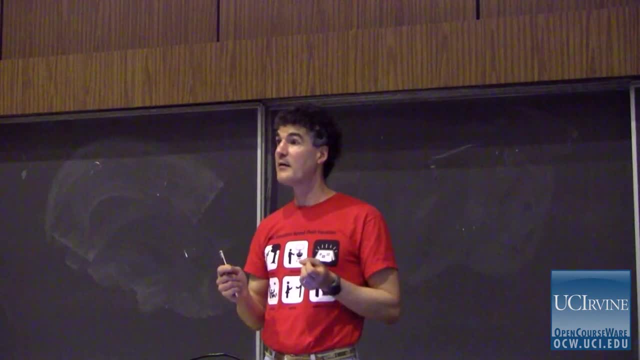 you can do easily And you don't get smarter or more proficient by just looking at the answer and never actually working it out. It's just a reaction. It's a reaction. It's easy when you see somebody else do it, to think, yeah, I could do that if I wanted. 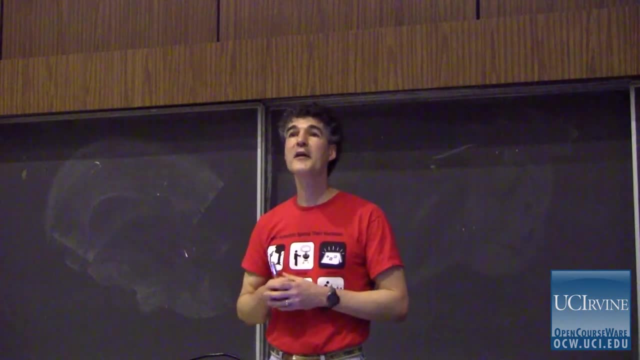 to. But you know I've got a lot of things to do today and that's not one of them, so I'll do that tomorrow. That's a problem for some people. You're paying a ton of money to come here. at least from my perspective, it's a ton of. 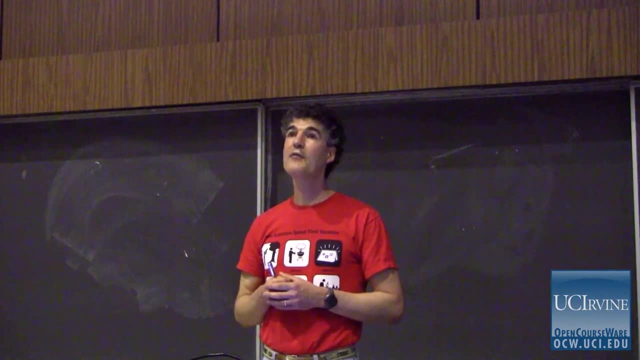 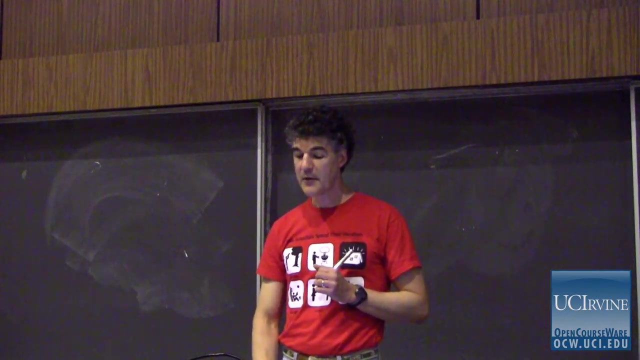 money and you have to make sure that you get every dollar's worth. I'm trying to give you good value, but I'm only half of the equation. The other half is how hard you work. Some of you worked extremely hard but, honestly, if you got a ten, you really need to look. 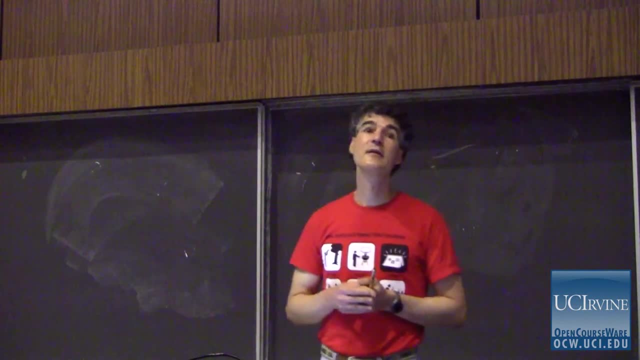 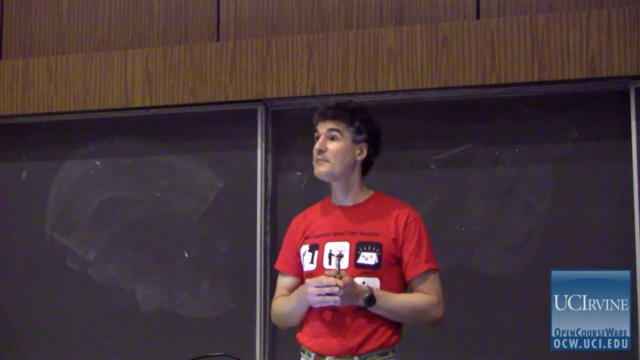 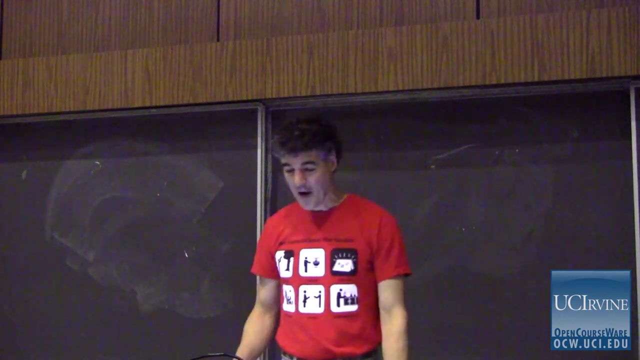 at what you're doing and you need to change it quickly because you won't pass the course with that kind of performance. All right, you get five for the exam form. all right, enough, said. I'm going to pick out the problems that I was particularly worried that the percentage. 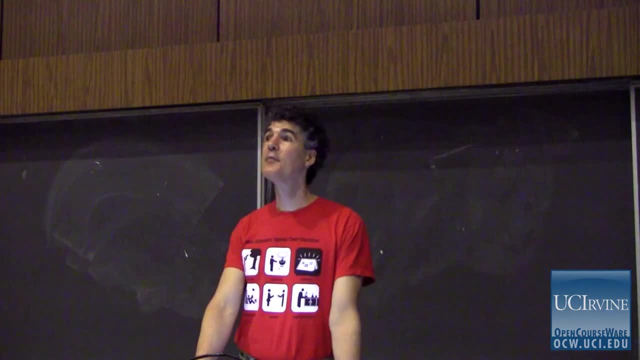 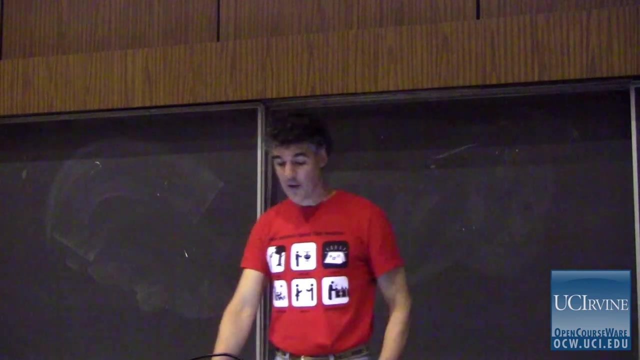 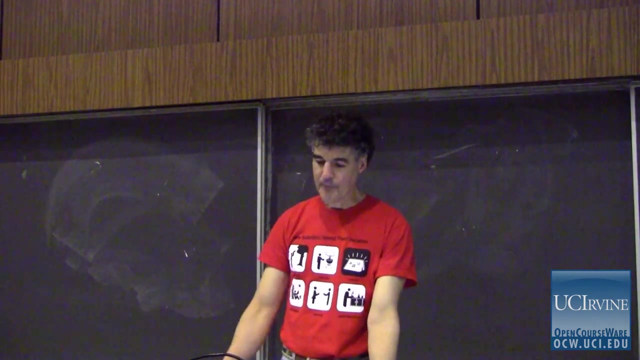 of wrong answers was high, and those problems are going to make an encore appearance on another exam. So study, Study this exam and make sure that you can do all these problems. That's the best way to learn. Okay, let's continue on with Chapter 12.. 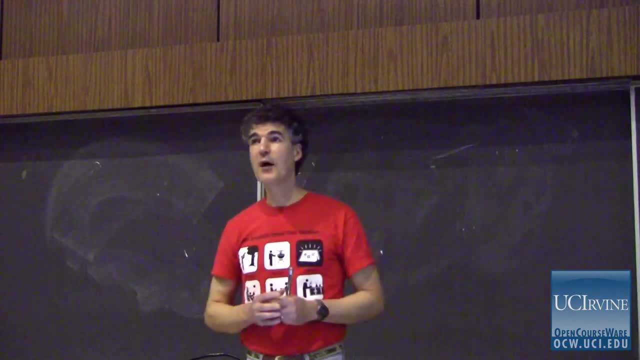 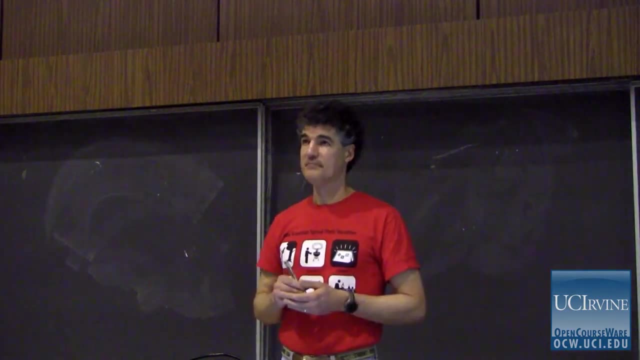 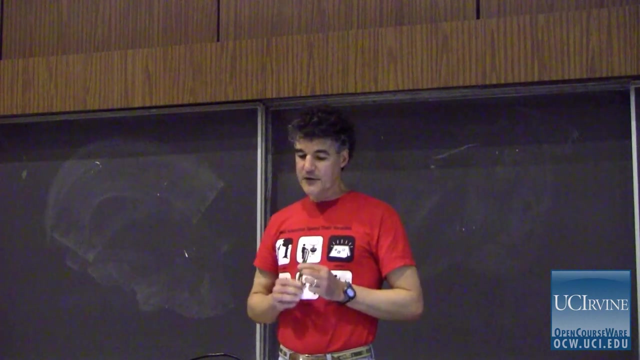 Solutions and Colligative Properties. Colligative properties are properties that depend on the number of particles in solution, but not on the details of the kinds of particles, at least not so much There are. first of all, let's talk about concentrations. 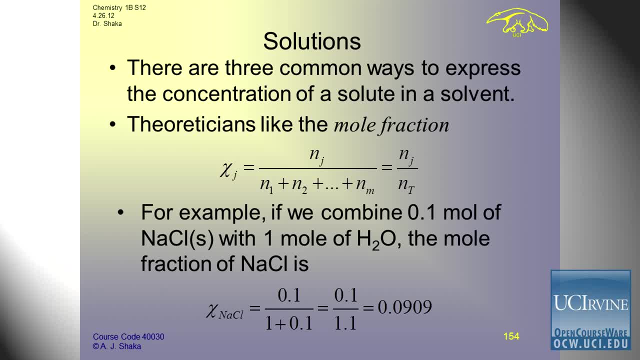 There are three common ways to express concentrations of a solute and a solvent. Theoreticians like mole fractions, because theoreticians don't have to actually measure anything, and so they don't have to actually make the same measurements. Okay, solutions up. 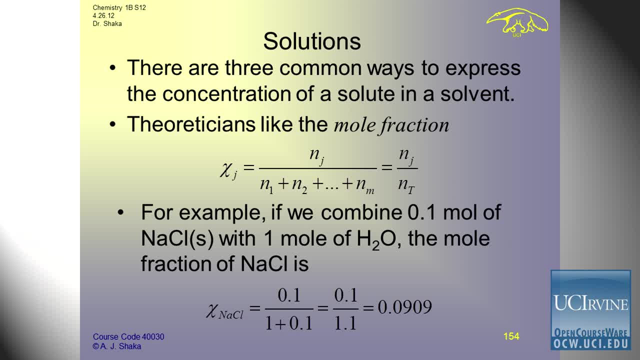 But they have very nice theories where the natural concentration is the mole fraction. That's just the natural thing to use. it drops out of the equations, it makes everything so simple. they love it. But an experimentalist doesn't like mole fractions, because then you have to. 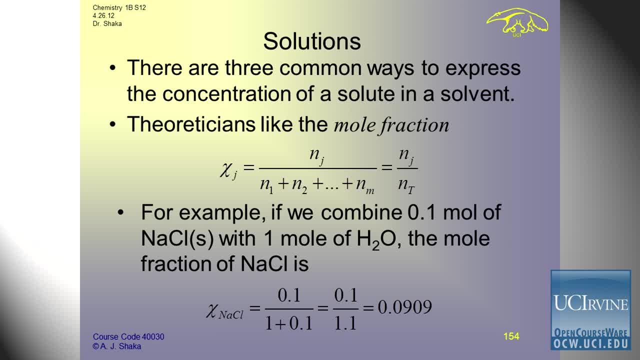 work out the moles of everything And it can be tedious. But the mole fraction is just the number of moles of whatever you've got divided by the total number of moles, And it's given this symbol, chi, Fancy looking X. 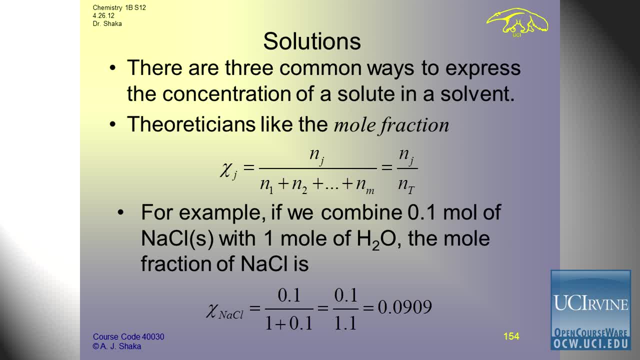 I may have told you, we use Greek letters to keep out the riff-raff in science. Greek letters intimidate people, and then you find out who's not easily intimidated. So, for example, if we take a tenth of a mole of sodium chloride and we have one mole of water, 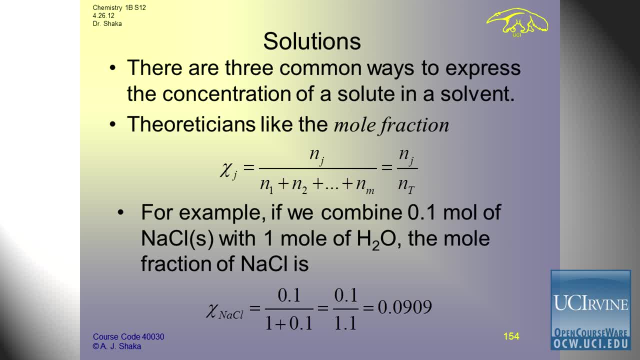 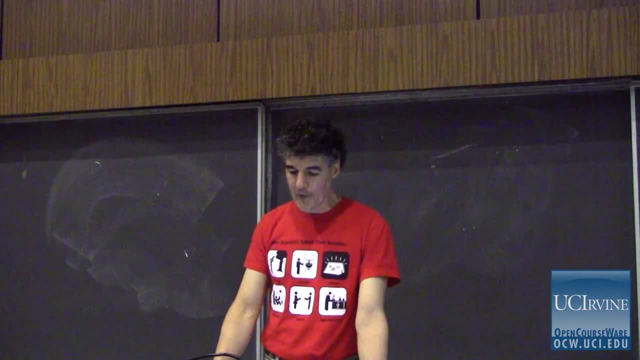 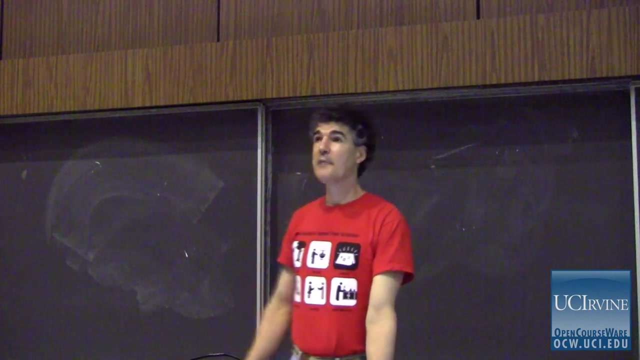 then the mole fraction of sodium chloride is just point one over one plus point one, or point oh nine, As I say. theoreticians like it, but it's not much used in the lab. Chemists want to make up solutions quickly and they want to make them up reproducibly. 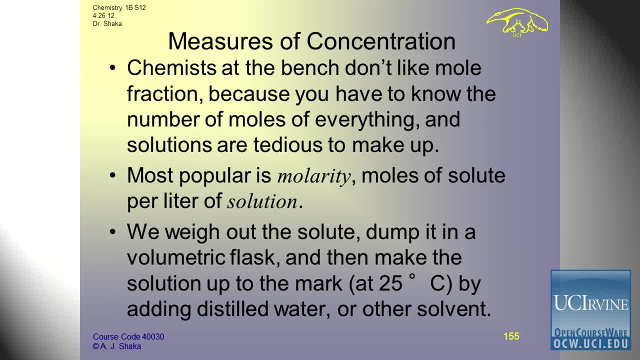 And so the fewer things they have to measure or fiddle around with, the better it is. You have to weigh out usually you have to weigh out what you're going to dissolve in the solution, Or if it's a gas. you have to know the solution. 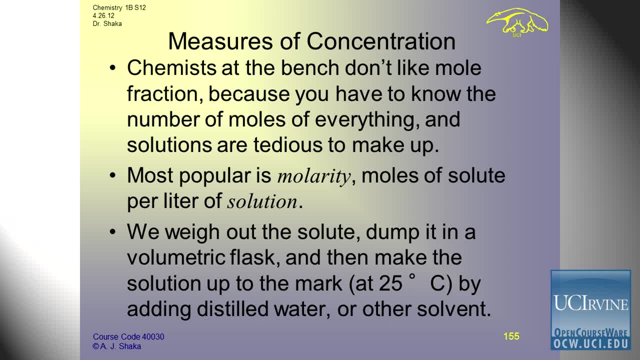 You have to know the pressure of gas you're putting in. That's not such a big deal because those things are usually easily measured and solids don't slosh around and it's not too bad. But when it comes to the liquid, there's an easy dodge. 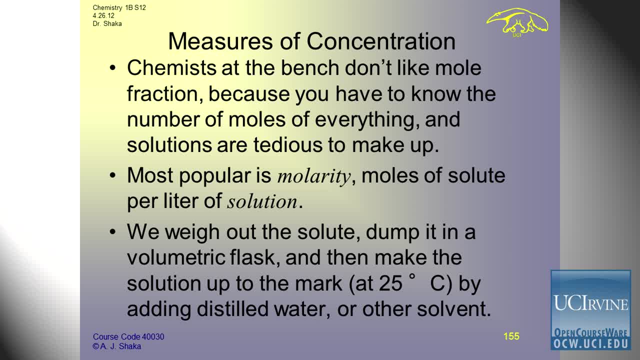 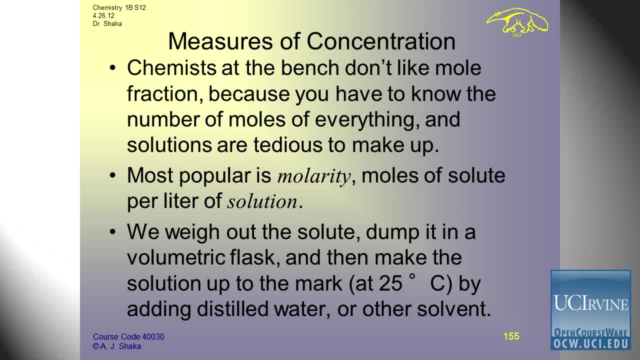 And the most common way to do that is to use a liquid. And the most common way to do that is to use a liquid, And the most common measurement, then, is molarity with an R, And that's the moles of solute per liter of solution. 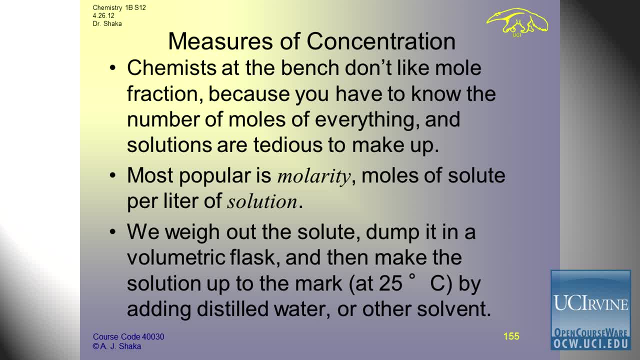 Again, chemists like to know how many moles are in there, because that has to do with how many atoms are in there and that has to do with how many little chemical reactions can occur If I just know how many grams of something are in there. 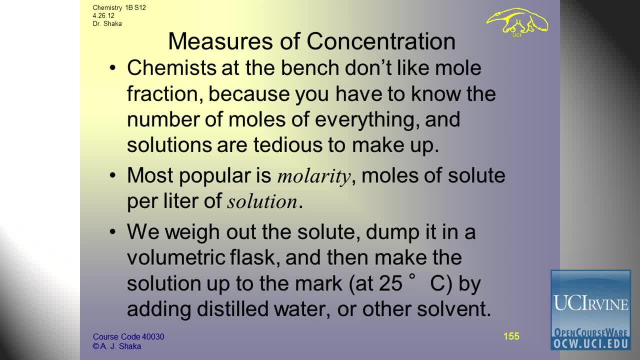 I don't really have a clear idea of what's going on. So we weigh out the solute and then we just dump it in, and then we make up the solution to a mark on a calibrated volumetric flask at the right temperature, which is usually 25 Celsius. 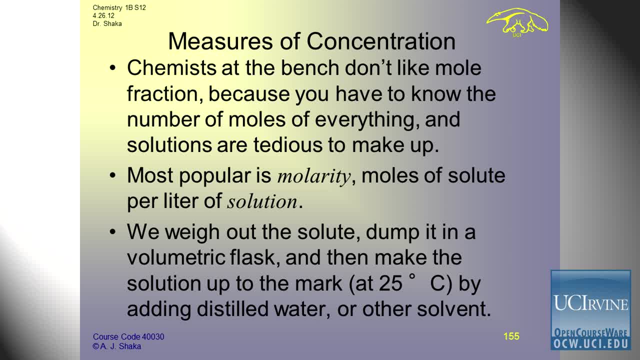 and we're done. And that's easy to do because you don't have to weigh out the water and the solute. So we weigh out the solute and then we just dump it in, And that's easy to do because you don't have to weigh out the solute. 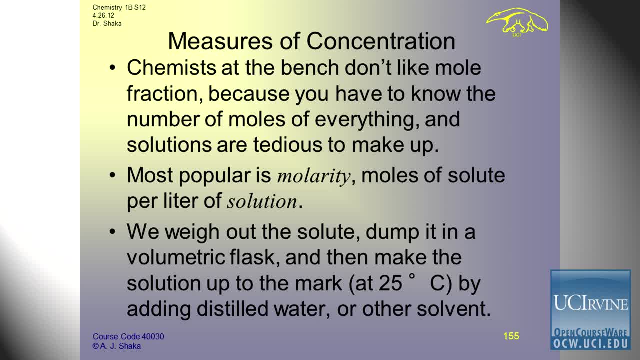 and then we just dump it in Or put in a certain number, especially if you have to put in a certain amount of volume of water. it's a nightmare, because the water sticks to the container that you use to pour it in and there's some left behind. 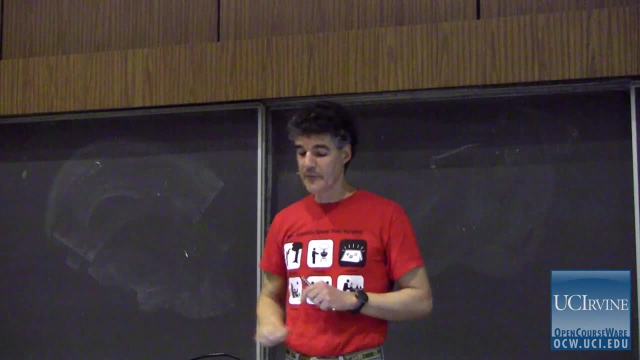 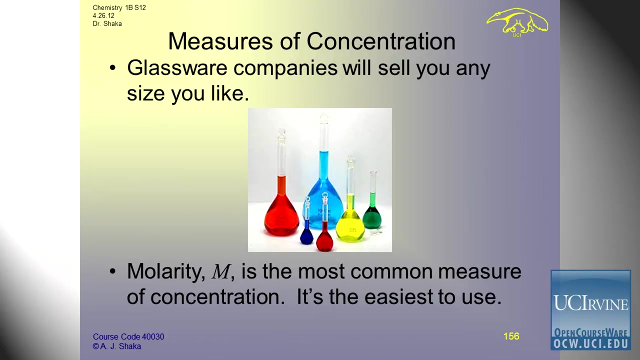 So that's a big problem. So to get rid of that, we define molarity to be moles of solute per liter of solution, And we don't want to have to measure the volume of the solvent. And Glassware company companies will sell you any size you like. 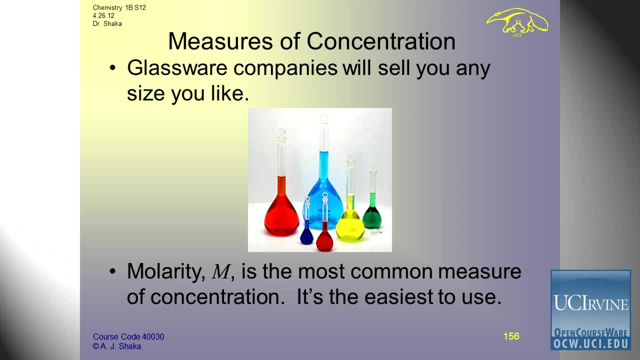 These are common things to find in the lab, And these are probably just food coloring, who knows. But in any case, you throw in the solid and you make it up to the mark. First, you add distilled water quickly and swirl it around, and that's why it has that shape. 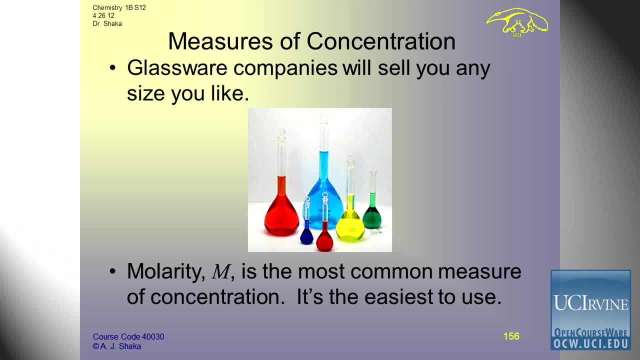 so you can mix it easily, not drop it on the floor. And then it narrows here so that you can get good accuracy on the scored mark. You don't want a big wide thing there. A little height is a lot of volume. 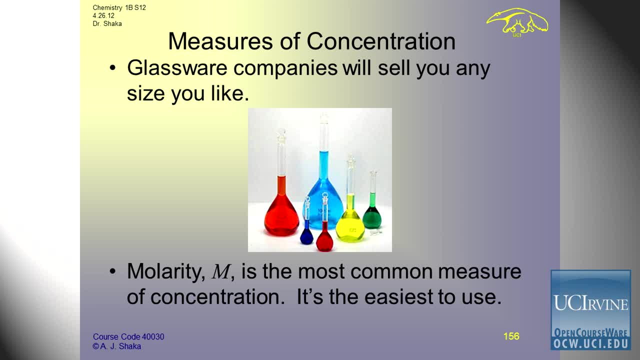 Yeah, I'm just curious, maybe a little off topic, but does that have anything to do with the like-as-loves, like kind of theory, Like if, for instance, if we used ethanol alcohol, would it do something with it? pretty much, 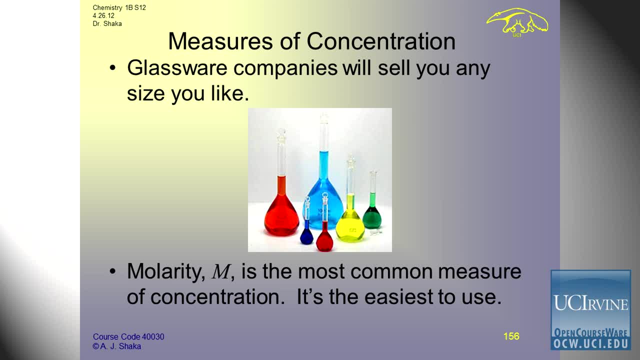 Would it be like that? Yes, If you try to make too concentrated a solution, let's say you don't know and you try to make 10 molar of something, so you pour in 10 moles of this stuff and then you throw in the water. 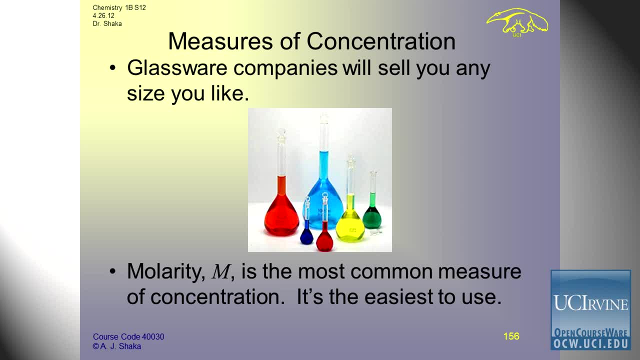 and it doesn't all dissolve, then you've got to start over, okay, And if you pour in a liquid and another liquid and they form two layers, that's it That you aren't making a solution, You're just making two layers like salad dressing. 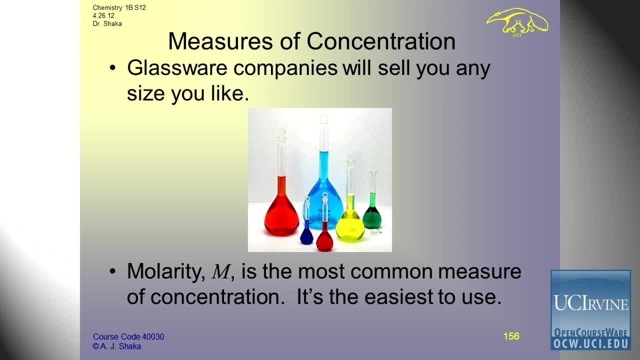 Ethanol would be a special case, Because ethanol is volatile. So when I pour in the ethanol I have to worry about some of it actually evaporating if I go away and that type of thing. So I have to be a little bit more careful with that. 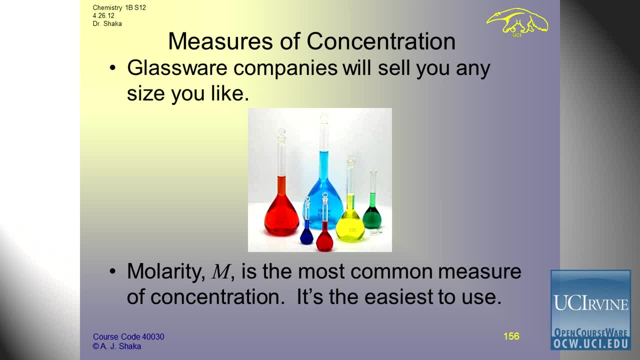 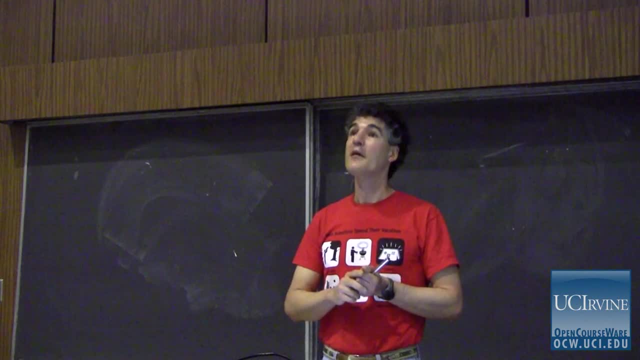 if I'm using a volatile thing. But ethanol and water will mix in all proportions. But, as I'll show you, they don't make an ideal solution. They make a solution, but they don't make a solution. but it's not what's called an ideal solution. 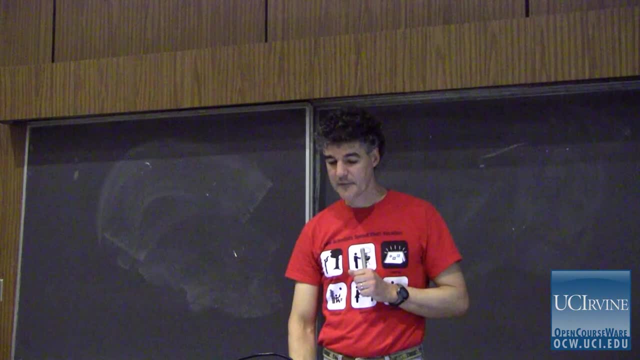 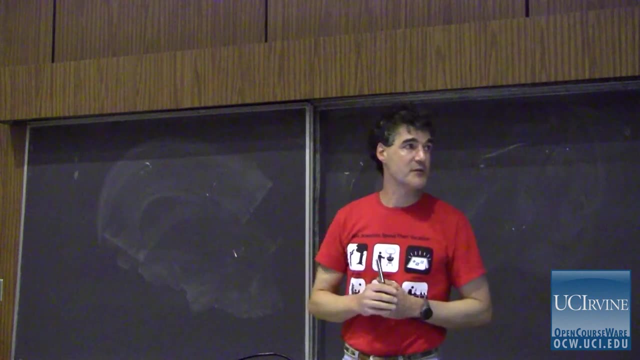 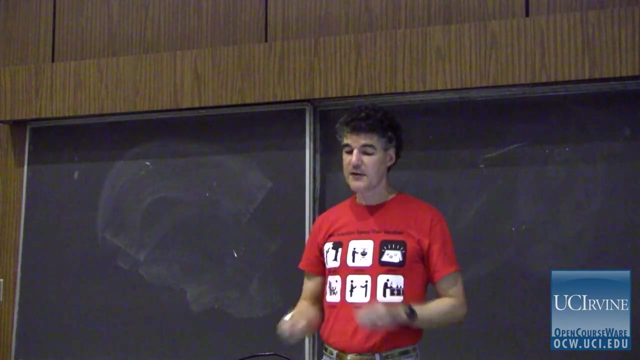 That's a special term, like ideal gas. This is the most common thing you're going to run into and it's the easiest to use, No question about it. And then, courtesy of some very important experiments, it turns out the final case instead of big M for molarity. 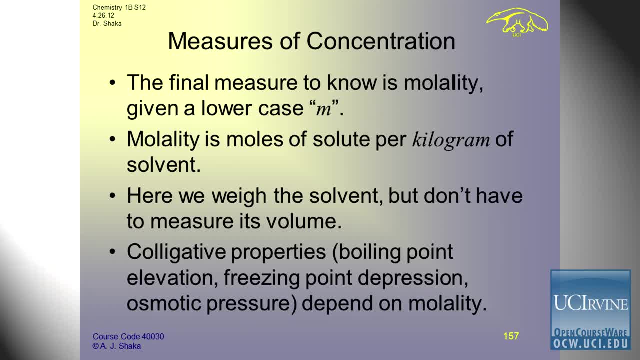 is little m for molality, And that's what I'm going to do. And again, I told you you don't want to have to measure the volume of solvent, But you don't mind weighing the solvent Because I can sit there with the volumetric flask. 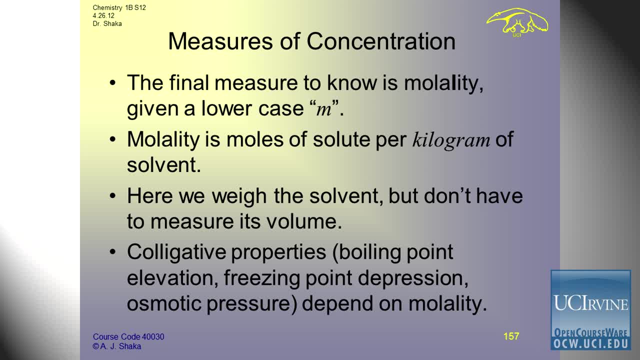 and I can pour in solvent while it's on a balance, And if I tear the balance I can add a kilogram of solvent, No problem. Again, that's pretty easy to do because I can add drops at the end and watch the balance. 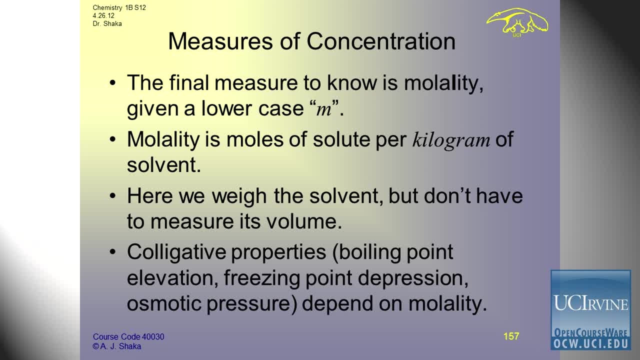 So that's OK, And this turns out to be important in certain kinds of experiments that I'll talk about, And so that's also a very useful thing to be able to do in an analytical chemistry lab, And the key is: we weigh the solvent. 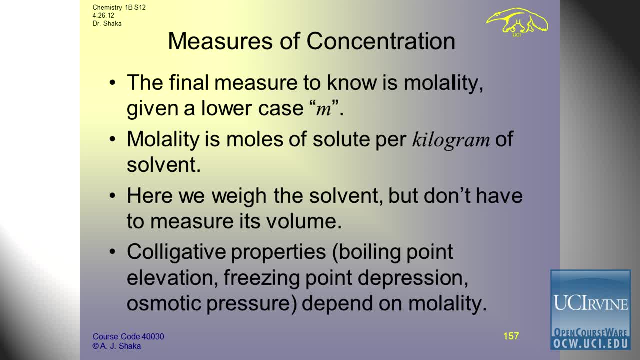 but we don't have to measure its volume. These colligative properties, There are a bunch of them: Boiling point, elevation, freezing point, depression, osmotic pressure and so forth. They all depend on the molality. That's what drops out of the theory. 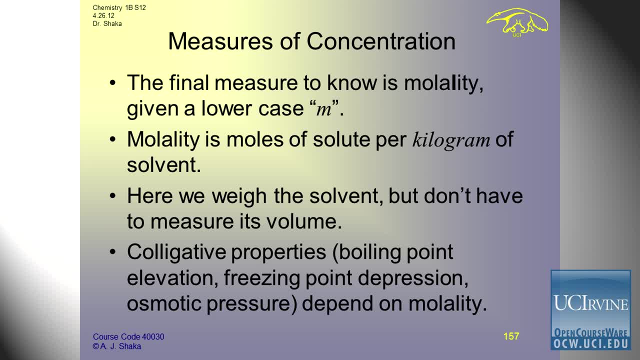 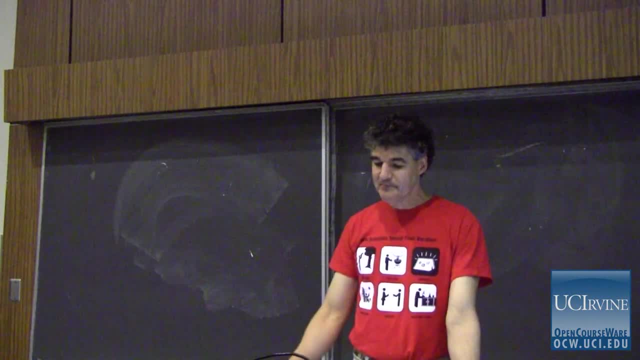 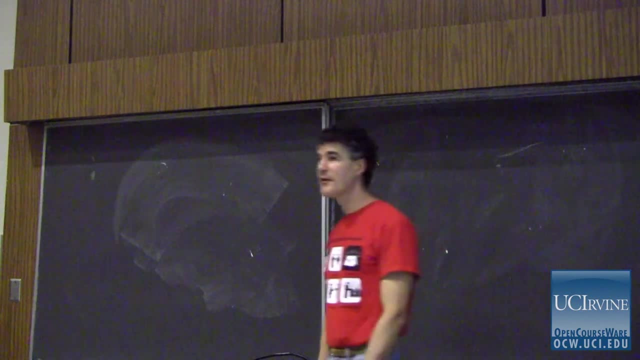 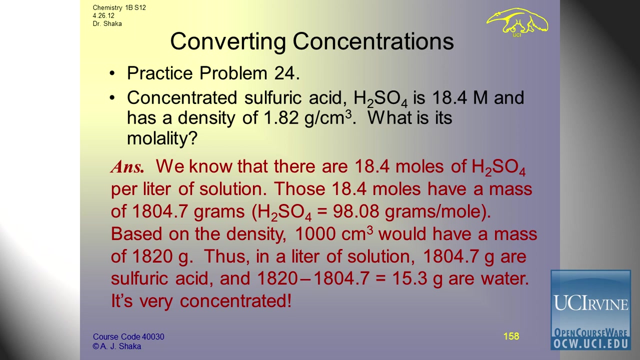 that you'll do in physical chemistry. Let's practice converting concentrations. These numbers are not exact, but let's just use them. OK, They aren't. I don't think they're quite right, because the molality comes out too high. as to what I recall, 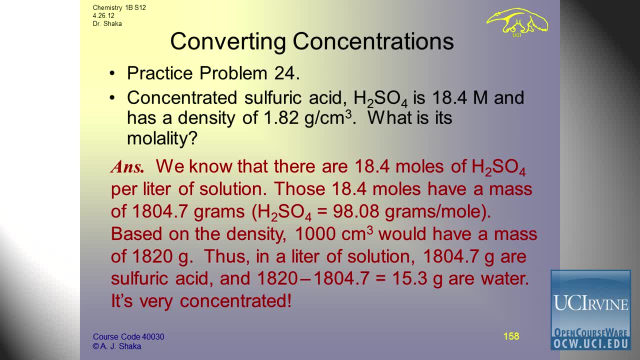 But let's try it. Let's assume that sulfuric acid is 18.4 molar and has a density of 1.82 grams per cubic centimeter. What is its molality? Molality- I need to think what I'm going to do. 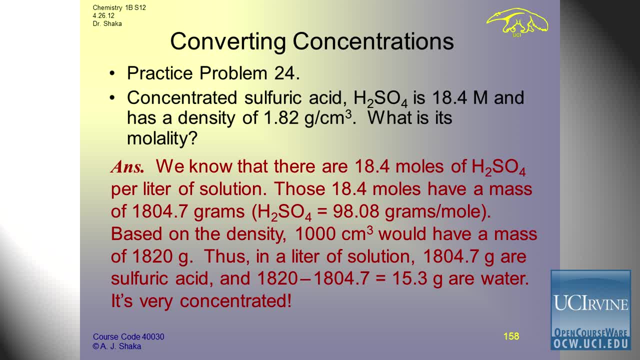 First of all, I know if I have a liter of solution. I know how many grams that weighs, because I know how many grams a cubic centimeter weighs And I know how many moles of sulfuric acid are in there. So if I look up the molar mass of sulfuric acid then I 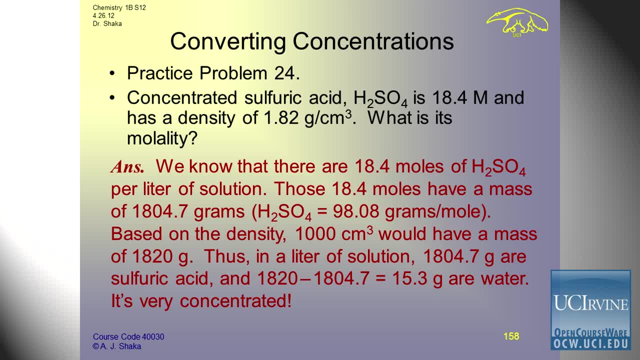 can tell How many grams of sulfuric acid is there. The rest of it is water, Because while volumes do not add, masses do. That's why we like to stick to calculating masses. If you mix two liquids together or you put a solid in a liquid, 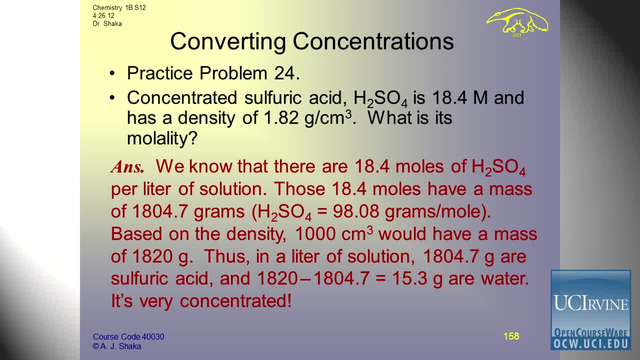 the volume won't add up. In fact it can sometimes actually get a little smaller, even though I add something, Because something I add can break up the structure. that's kind of pushing the thing apart and actually make it shrink, And that's very confusing then to try to measure things. 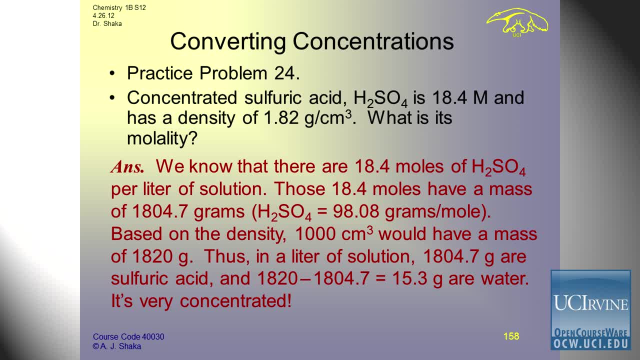 by adding up volume. So we never, ever, do that in chemistry. OK, let's have a look. There are 18.4 moles of sulfuric acid per liter of solution. Those 18.4 moles will have a mass. 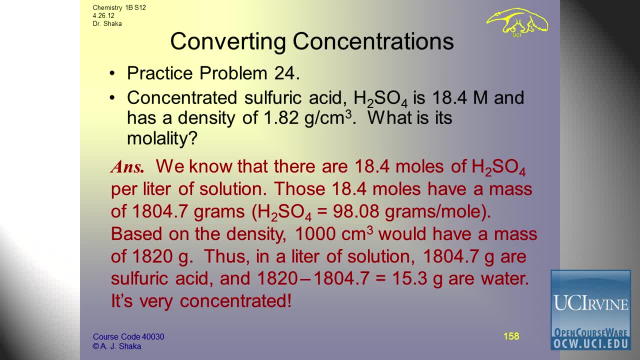 A mass of 1,804.7 grams, based on the density of 1.82.. And here I'd like to have some more digits, But let's take 1.82.. 1,000 cubic centimeters or one liter of solution. 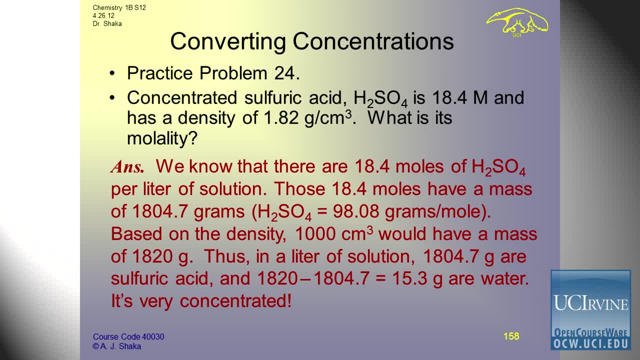 would have a mass of 1,820 grams Out of the 1,820.. Almost all of it is sulfuric acid. There's hardly any water, So this is really, really concentrated solution. We can do that because sulfuric acid itself is a liquid. 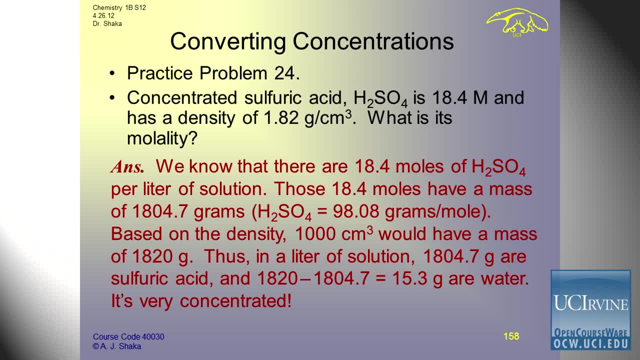 It's a very, very viscous liquid itself. It's not going to solidify on us and come out of solution. Well, out of this, 1,820, 1,804.7 are H2SO4 molecules And that means the other 15.3 are water. 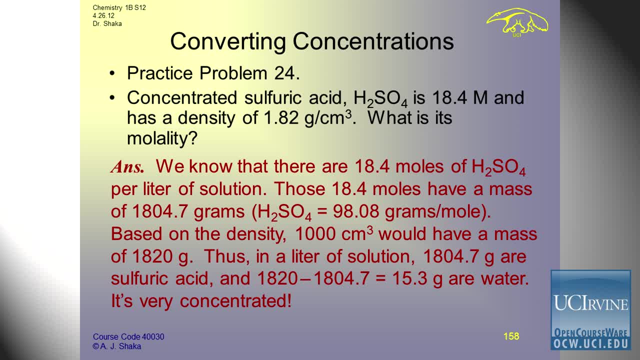 And now for molality. I have to figure out how many moles I would have in a kilogram of solvent. But a kilogram of solvent is a lot more than 15.3 grams, So the molality is going to be quite a bit higher. 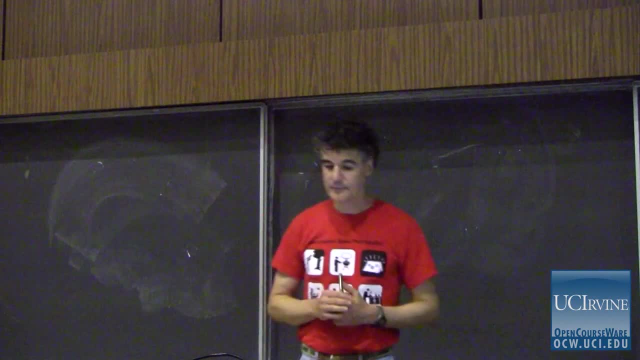 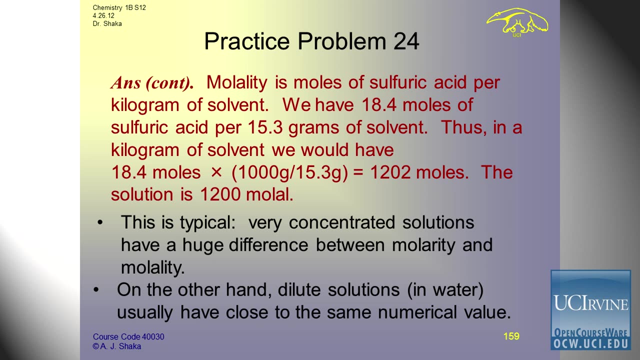 So let's have a look. The molality is moles of sulfuric acid per kilogram. We have 18.4 moles of sulfuric acid for every 15.3 grams. So in a kilogram we have 18.4 moles times the ratio. 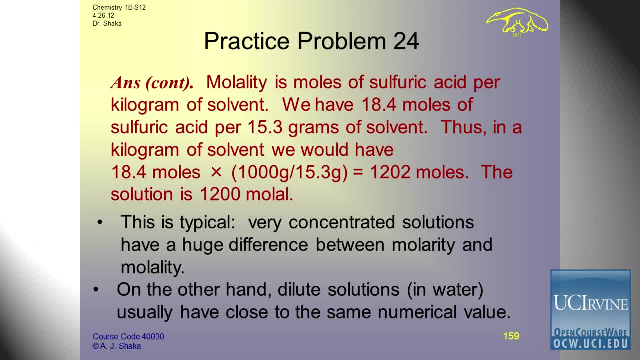 a kilogram, 1,000 grams, over 15.3 grams, And we cancel out the units And we have 1,215.2.. 1,215.2.. and two moles and therefore the solution is 1,200 molal. 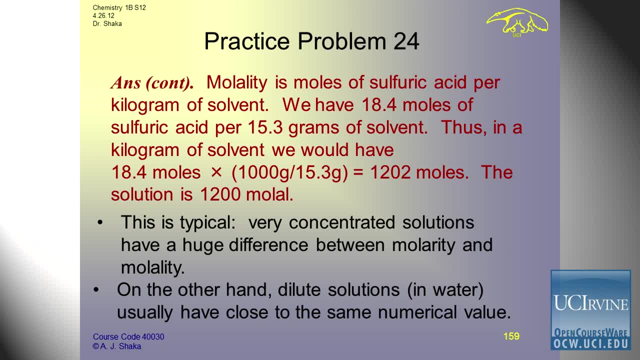 I think that number is in fact quite a bit too high. I think if you look up the literature you'll find it's more like 500 molal, And I think that's down to me calling it 18.4 molar. 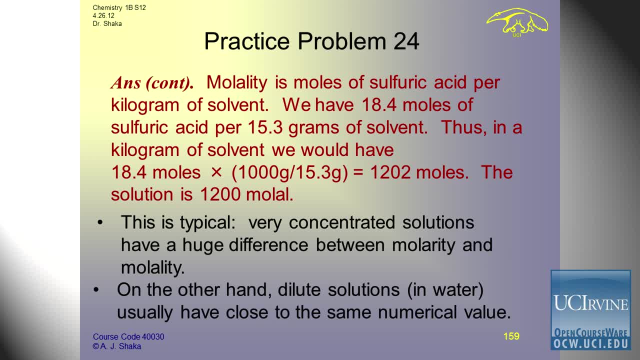 and the exact density that I used, But in any case it's got a lot higher molality than molarity, And that's always true. if you have a concentrated solution, The molarity is much lower than the molality. On the other hand, if you have a dilute solution, something, 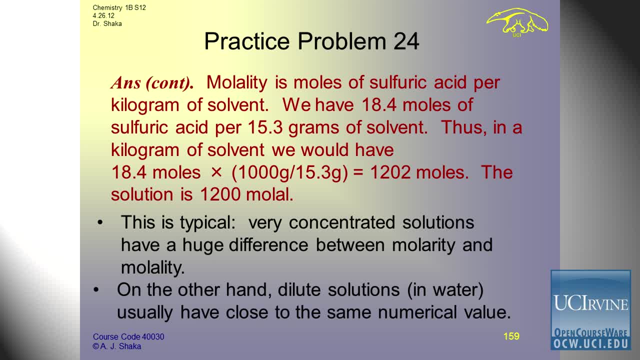 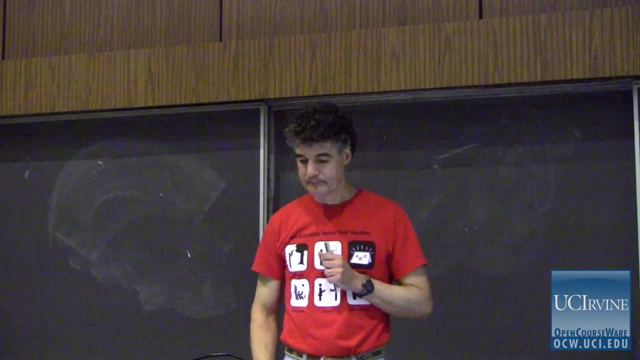 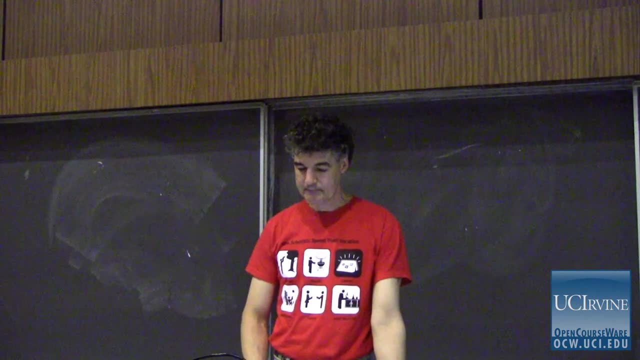 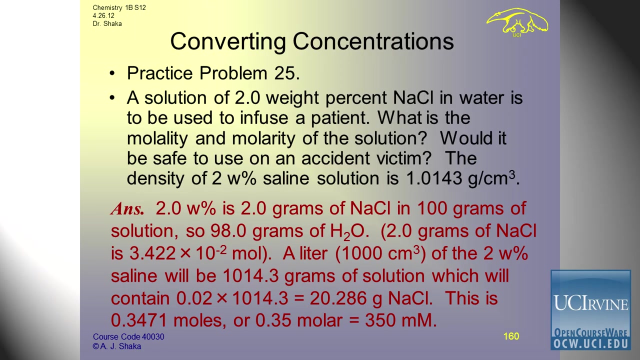 let's say, in water. usually they have close to the same numerical value. So let's convert concentrations again And let's do something that we might find at a hospital. People have made very bad mistakes at hospitals by administering infant 1 molar heparin instead. 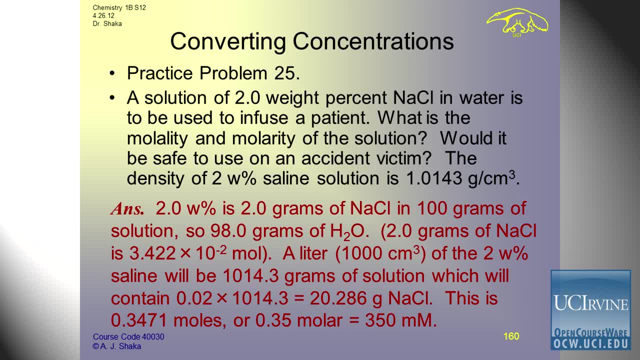 of 1 millimolar heparin, which led to a lawsuit that you may have made And you may have heard about. You're supposed to dilute it. You forget or you don't know what the units mean. You blast this little kid with weight 1,000 times too much. 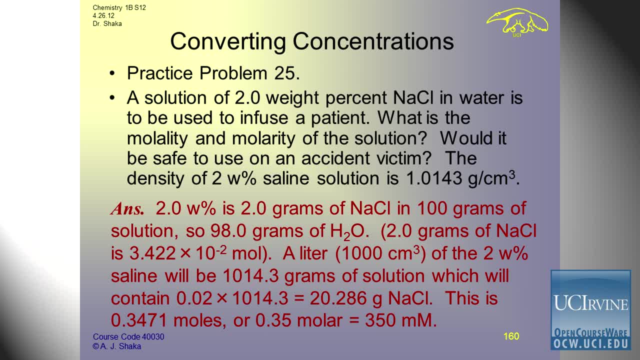 of something, And even if something's a medicine, 1,000 times too much is usually not a good idea for anything And you can have an adverse reaction. And then, if you fail to understand why you're getting an adverse reaction, and deal with it. 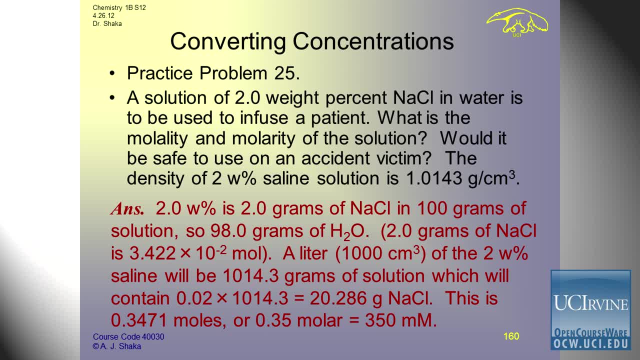 you can have a death on your hands, And you did it by being careless. So let's take a 2 weight percent. Chemists don't like this 2 weight percent sodium chloride in water And I'm going to use that to infuse a patient patients. 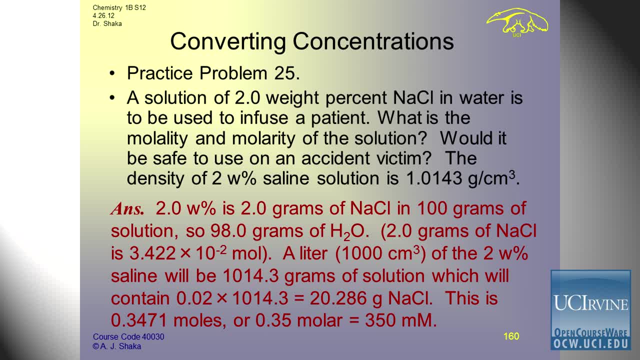 in distress, I'm going to puncture a vein. I'm going to string up this bag, like you've seen on TV, and drip in some extra fluid so that they don't go into shock. Question is: what's the molality and molarity of this solution? 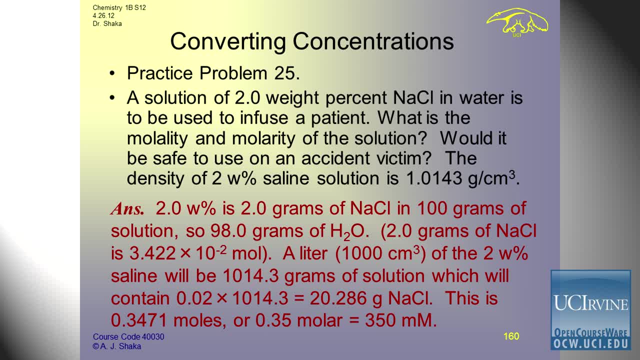 And would it be safe to use on an accident victim? And I found out that the density of 2 weight percent saline is 1.0143. Grams per cubic centimeter, So it's pretty close to the density of water. Usually that means if it's dilute like this. 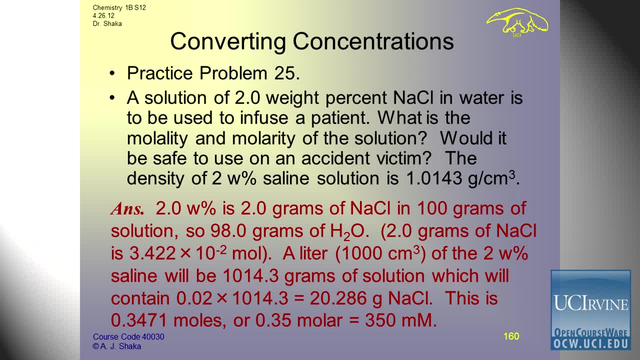 that the molarity and the molality will be similar. So let's have a look And let's see what they are. So 2 weight percent means 2 grams of sodium chloride in 100 grams, 2 grams of the whole thing put together. 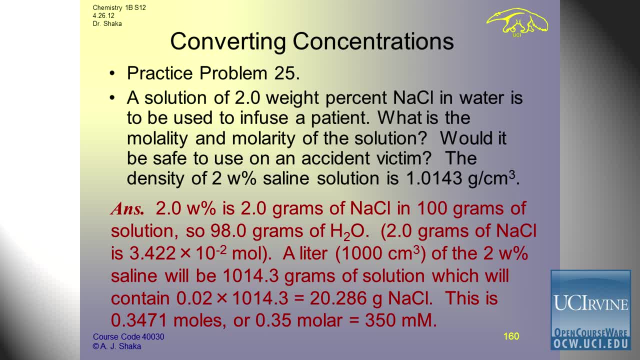 100 grams of solution, Total amount of material, And that means that it's got 98 grams of water, 2 grams of sodium chloride at 58.44 grams per mole gives this number of moles a tiny number of moles. 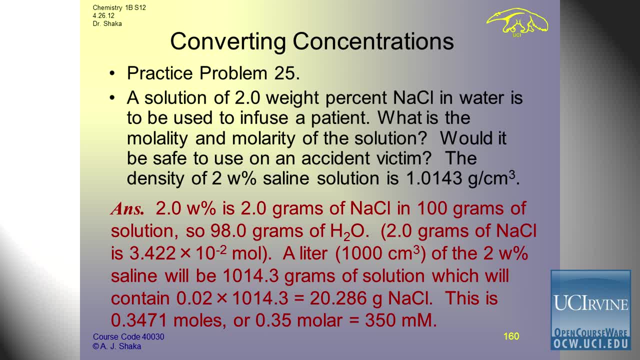 A liter of this solution, Based on the density, is going to be 1,014.3 grams of solution, And that's going to contain 0.02 times 1,014.3, because this is the weight percent- or 20.286 grams of sodium chloride. 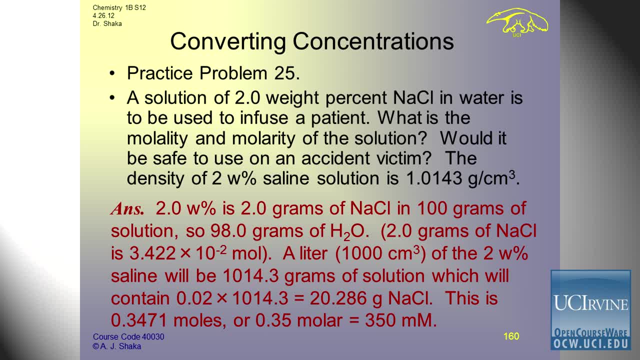 I don't believe 5 digits here. I'm not sure I'm not saying. I believe that You can't measure usually things to 5 digits, except voltage if you're lucky. But this is an intermediate result in the calculation. 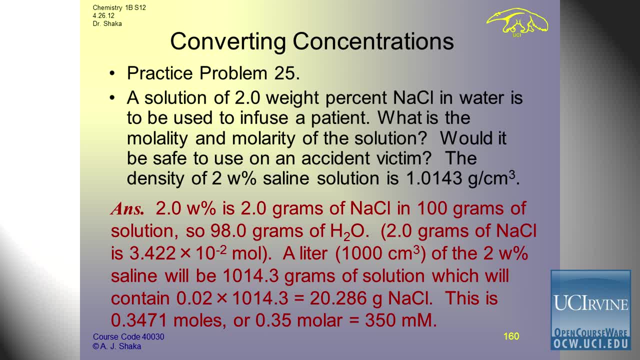 So I'm just keeping all the digits And I'm going to round it off at the end when I'm done. This amount of grams of sodium chloride is 0.3471 moles, or about 0.35 molar. 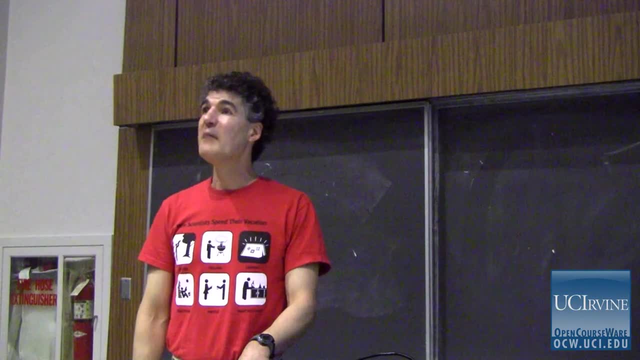 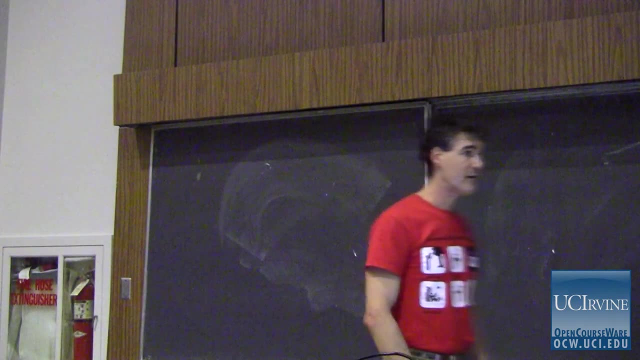 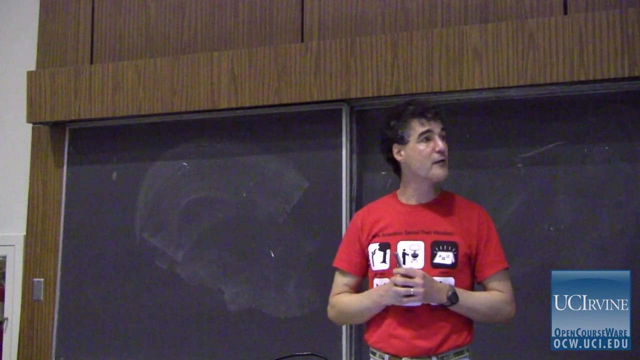 Usually we would call this 350 millimolar because we just like to use numbers that are bigger than 1, are kind of easier for us to understand as long as they aren't too big. So it's 350. millimolar is the concentration and molarity. 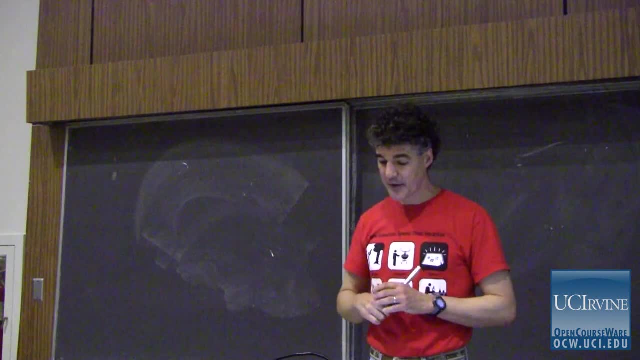 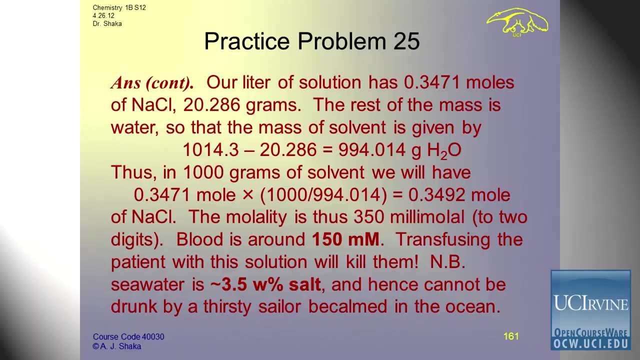 of sodium chloride in that 2 weight percent solution. The rest now to figure out the molality. I want to figure out how many grams of water is in the liter of solution And I've got 20.286 grams of sodium chloride. 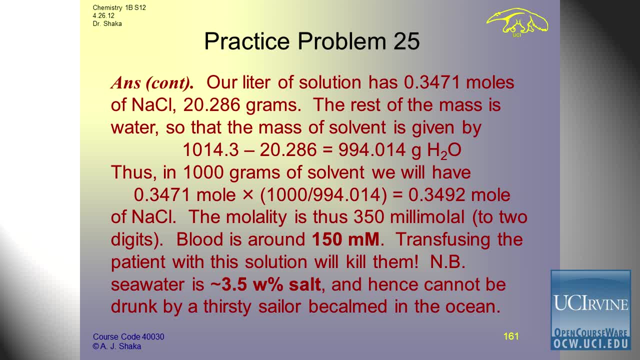 And I know how much the liter of solution, what mass it has: 1014.3.. So I just subtract them And therefore in that I've got 994., 014 grams of water, And therefore in 1,000 grams of solvent. 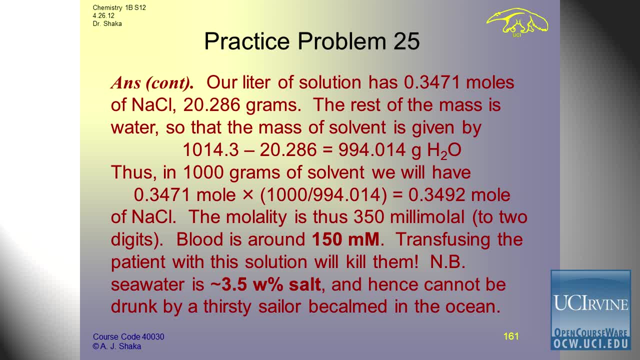 we have this number of moles per 994.014 grams times 1,000.. And I should have put the grams in here, but it didn't fit across. But I mentally put the grams in and then I mentally canceled them out. 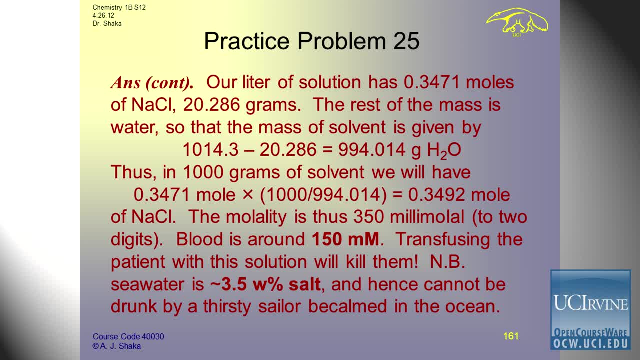 And I end up with 0.3492.. So that's the number of moles. The molality is 350 millimolar to 2 digits. So the molarity is 350 millimolar and the molality is 350 millimolar. 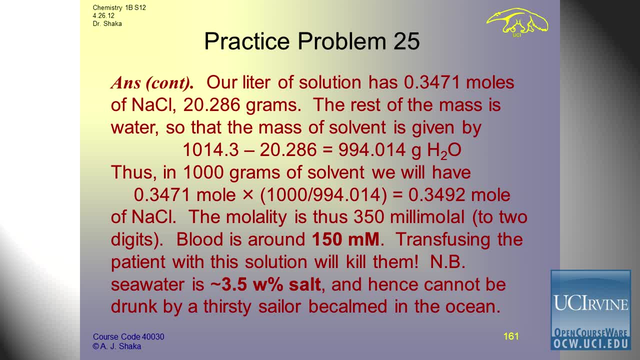 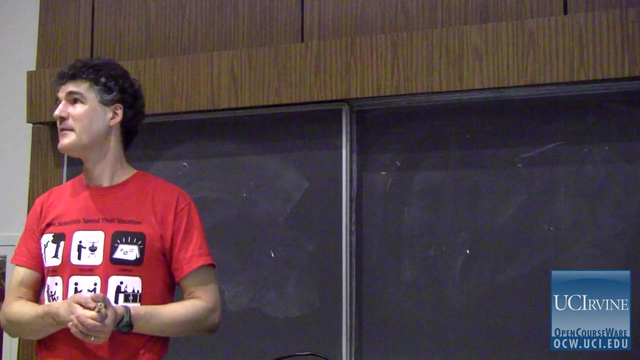 OK, Close enough. Blood is around 150 millimolar salt. That's why it tastes salty. Also tastes bad, I guess, unless you're a vampire, If you transfuse the patient with this solution, you will kill them. You'll finish the job. 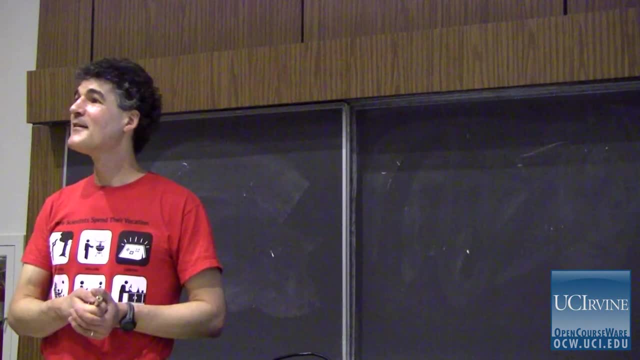 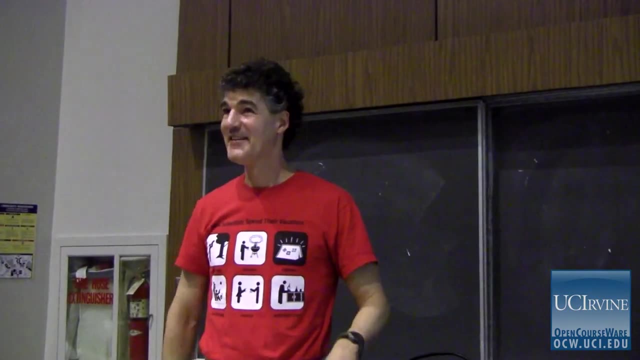 They got in a car wreck. They're on their last legs. Fear not, I'll save you. Wait a second. What's in the bag? Ah, forget it, It's saline. There are different concentrations of saline and they're used for different things. So if you grab the wrong one, that's it. You just finished the job on that guy. Seawater is 3.5 weight percent salt, And that's why, if you try to drink seawater because you're thirsty, you die. You actually get more and more dehydrated as you go And you expire, But the urge to drink something liquid that's cold if you're thirsty, can be overwhelming. I don't know how thirsty you've ever been, but I've been extremely thirsty. 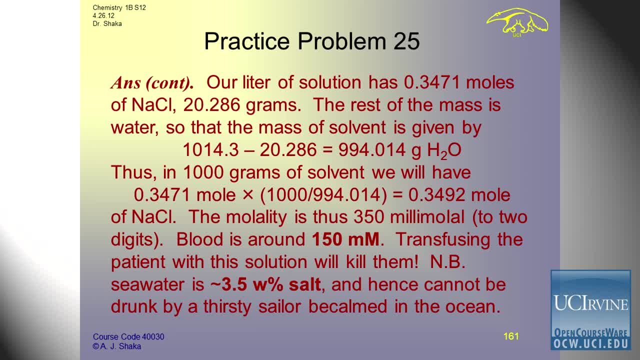 And I can tell you that some dirty puddle of water starts looking pretty good. under those conditions, You would never ever drink it normally. But if you really think that you're going to die and your tongue is a dry lizard hiding out in a cave, 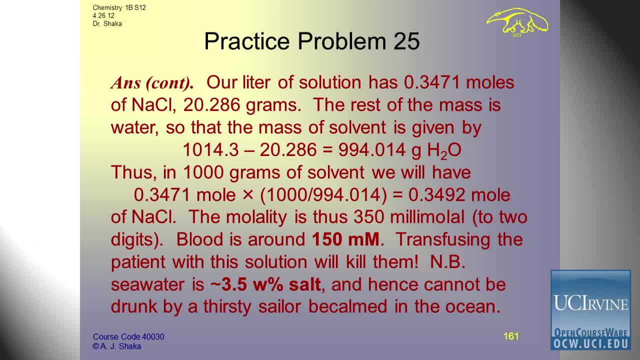 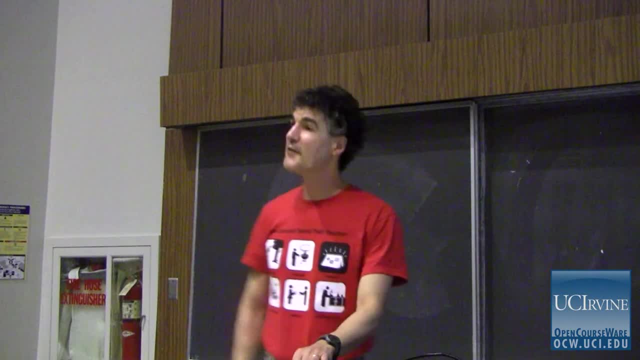 and turning colors and you're getting hot and cold and you've stopped sweating three hours ago. that water looks pretty good, And so if you get marooned on a sailboat in the ocean, sometimes sailors would succumb to the urge to start drinking. 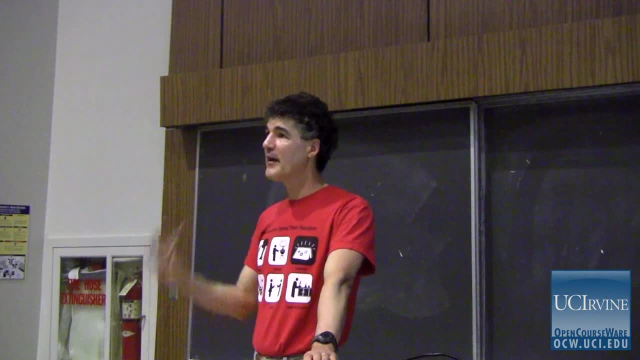 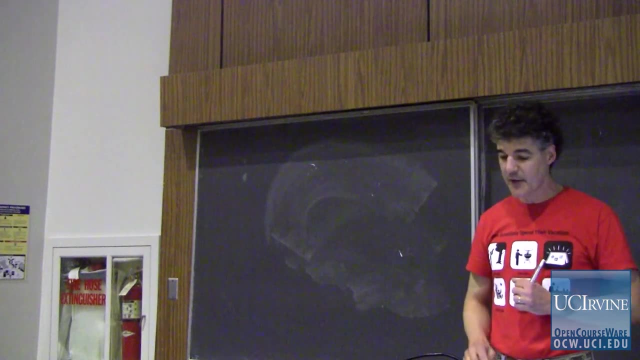 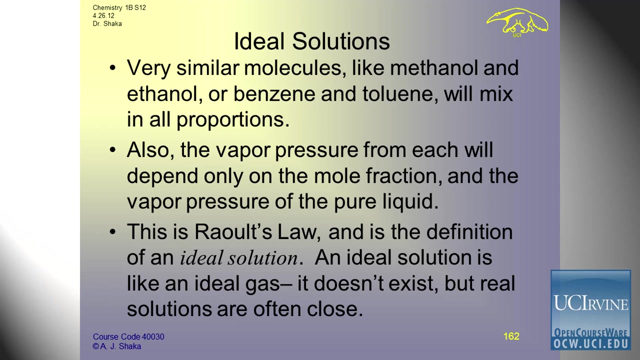 And then it's kind of like a siphon: Once you start drinking something, you tend to keep drinking it and they would die often. Okay, let's talk about this term ideal solution. We had an ideal gas. An ideal gas was one that followed the ideal gas law. 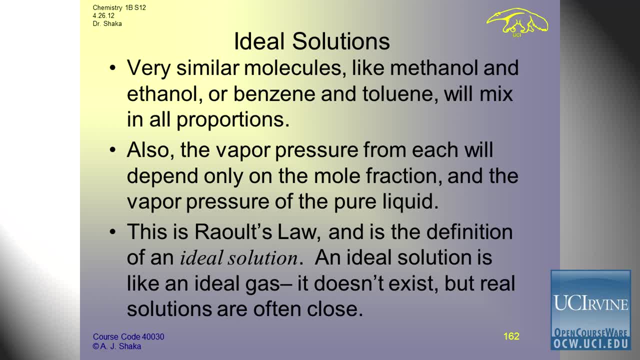 and real gases were sort of closed, And if we have very similar molecules like two alcohols, methanol and ethanol, and we mix them together, they'll mix in all proportion and they'll make quite a good solution. that will approximate an ideal solution. 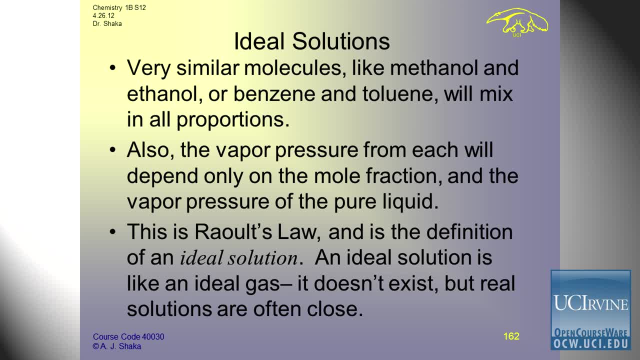 And likewise, if we mix toluene and benzene, that will also be quite an ideal solution. What does it mean that it'll be an ideal solution? Well, first it has to mix in all proportions From 1% of this. 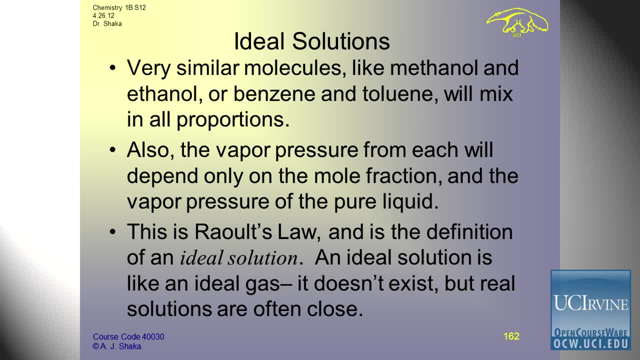 to 99% of this. if I've got two things, They always mix entirely. I never get anything sitting on the bottom. I never get two layers. Second of all, when I measure the vapor pressure of each thing, they follow exactly what the mole fraction. 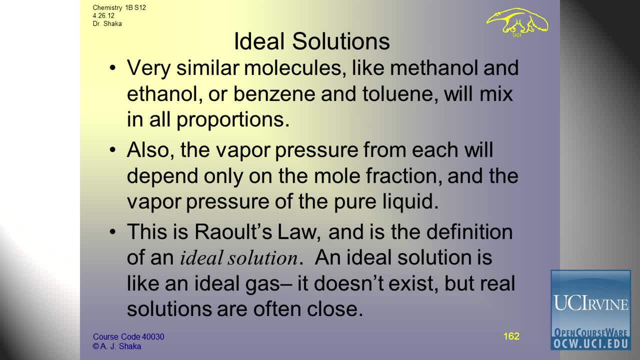 so this is why the theoreticians like this: The vapor pressure of each thing in the solution follows exactly the mole fraction of the stuff in the solution times the vapor pressure of the pure liquid. If I measure the vapor pressure of pure water at some temperature, 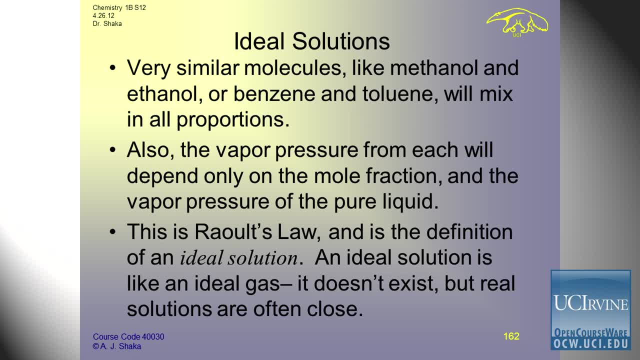 to be 400 torr, and I have an ideal solution and the water has a mole fraction of 0.9,, then the vapor pressure of water will be 360 torr. right on, And it'll follow If it's 0.8, it'll be 320, and so forth. 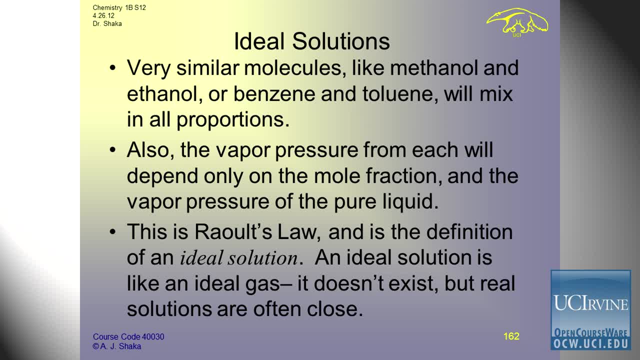 All the way down to 0.. And this proportionality between the mole fraction and the vapor pressure is called Raoult's Law. And Raoult's Law if all the components, all the chemicals in a solution follow Raoult's Law. 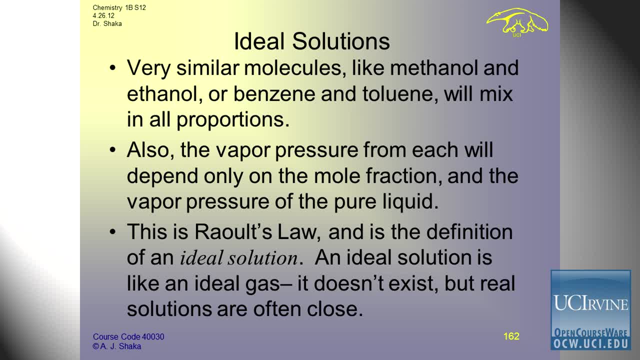 the solution is called ideal. That doesn't happen that often, but it does happen from time to time. If you pour something into a solvent and the temperature changes, it either gets colder or hotter. no way is it going to be an ideal solution. 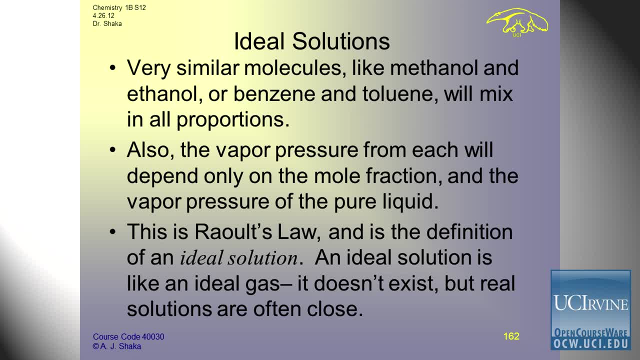 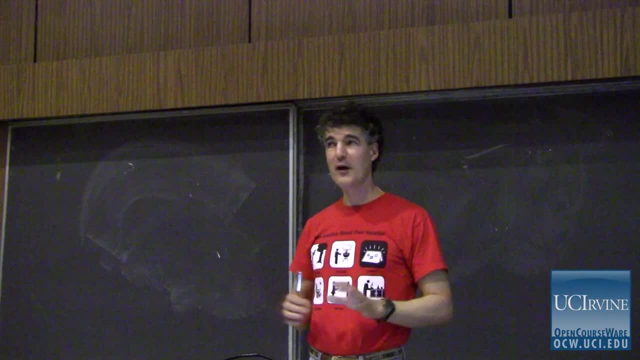 It's going to be way off, But that's one clue. If you pour something in and it gets really hot, a lot's going on, They're interacting, and so they aren't going to follow Raoult's Law. Of course, if you pour in two beakers. 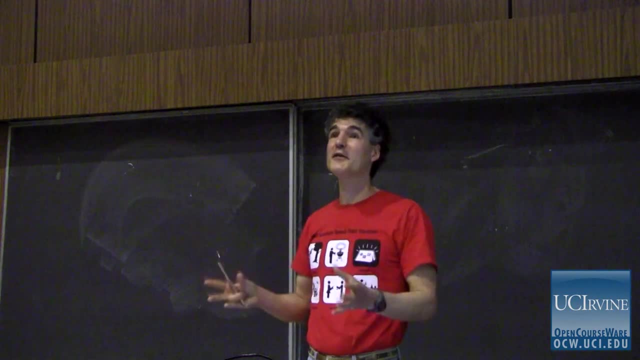 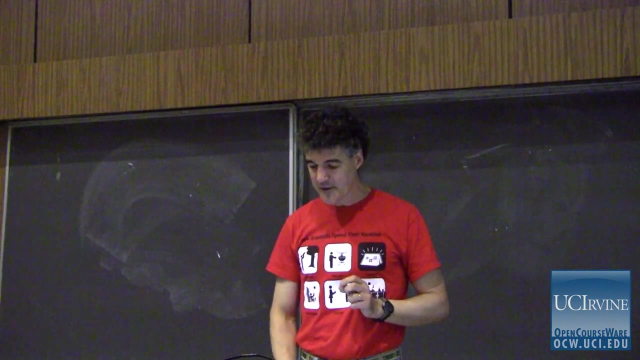 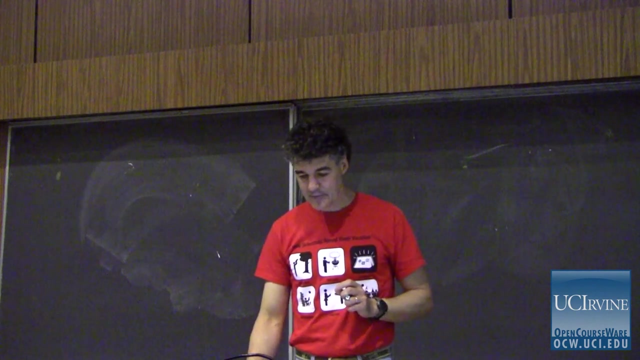 and they're in fact the same thing. that's an ideal solution, because it follows it perfectly. And they don't really exist. but real solutions are sometimes pretty close. Sometimes they're far off, but sometimes they can be pretty close. So let's have a look then. 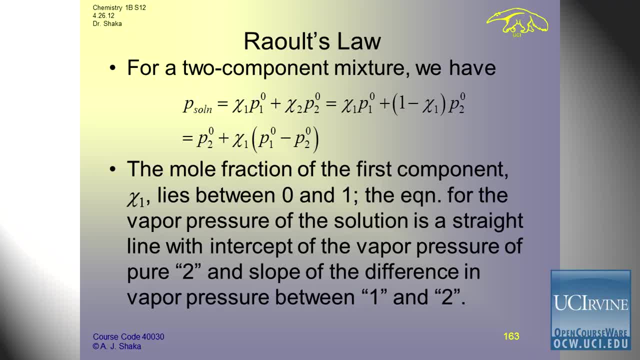 at these ideal solutions. So again, we use chi for the mole fraction, The pressure of the solution. the vapor pressure, and this is at a given temperature, is equal to just the mole fraction of whatever the first thing is times, whatever the vapor pressure. 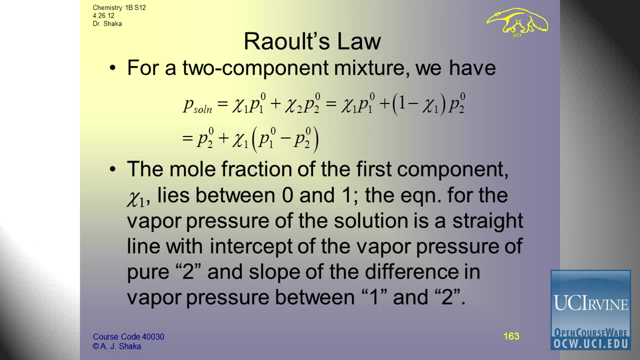 of that pure thing is Things have different vapor pressure And then the mole fraction of the second one times the vapor pressure of the second one, And if I only have two things, then the mole fractions have to add up to one so I can substitute. 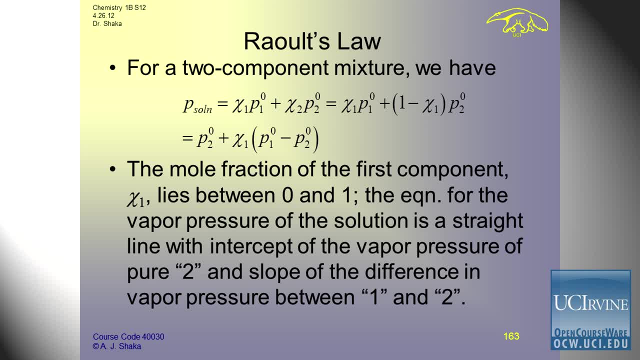 for the mole fraction of the second one, one minus the mole fraction of the first one. And if I rearrange that, I see that the vapor pressure of the solution is the vapor pressure of one of them plus the mole fraction of the other, times the difference. 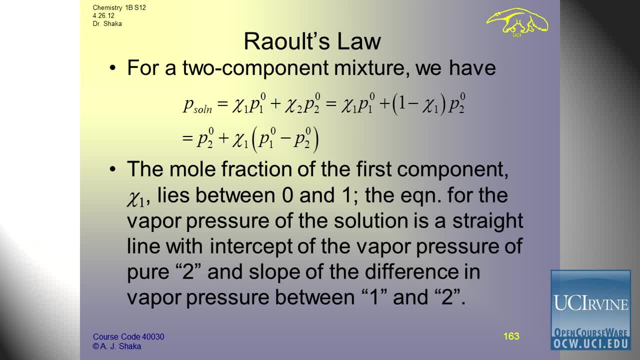 And I like that because I understand that if chi is varying between 0 and 1, which it does because it's mole fraction. so now I can make a plot. I start with: chi equals 0, and it's the vapor pressure of the other stuff. 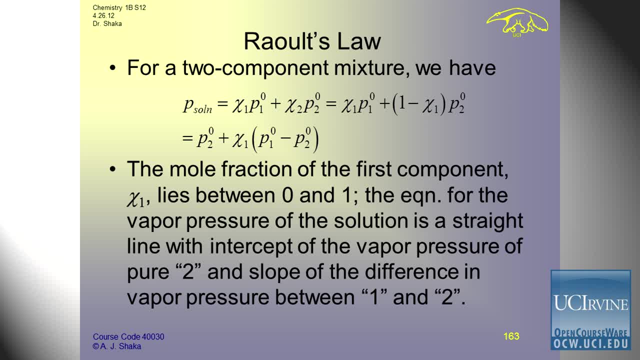 because it's 100% the other stuff. And then, as I increase the amount, the percentage of component one, the vapor pressure heads. Finally, when it's one, the vapor pressure is p1 of the pure stuff, And this is a straight line. 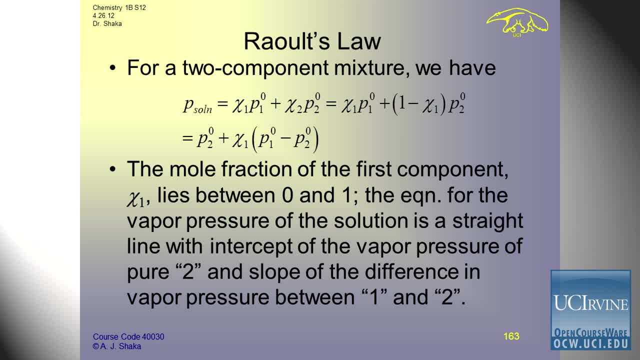 And therefore if I plot it and I look at the vapor pressure and it's always a straight line like that, then I know it's following Raoult's law. If it curves, then it's deviating from Raoult's law. 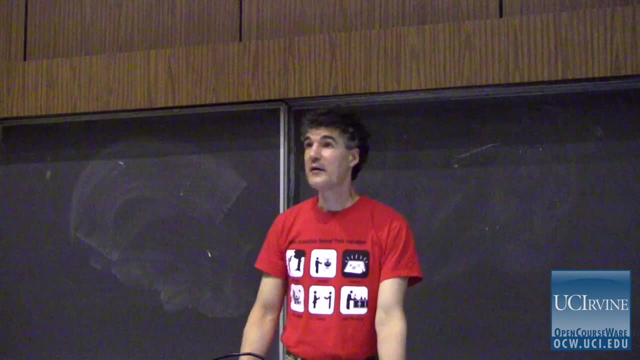 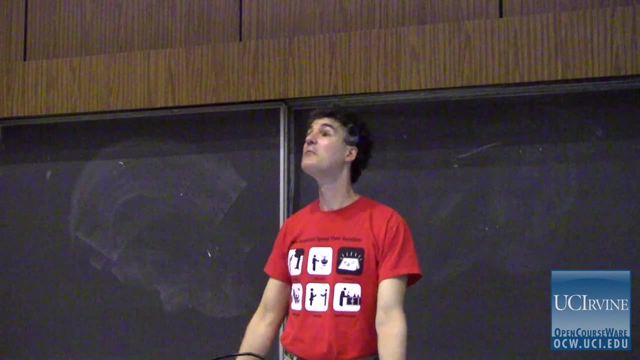 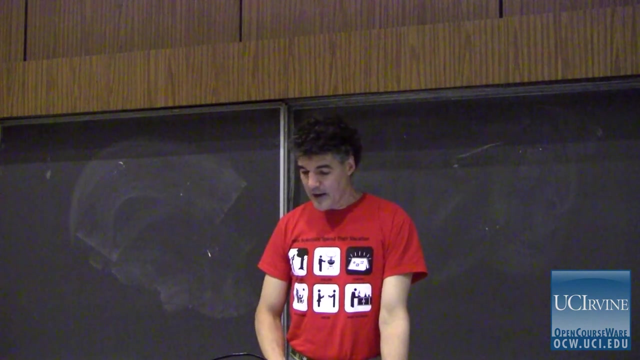 and that's just the same as with gases. When we keep doubling the pressure, the volume can't keep halving all the way down, because the volume can't go to 0. And so it starts curving. Same thing here. Alrighty, well, let's have a look. 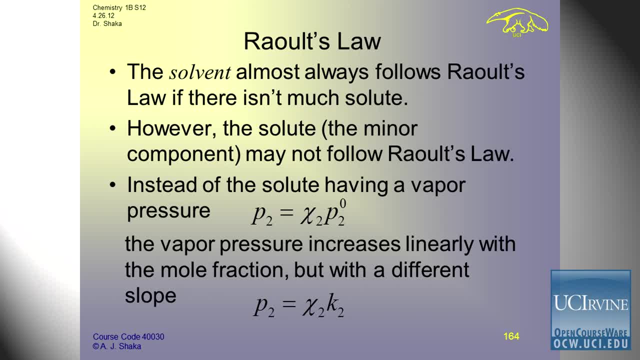 The solvent. if you've got a ton of solvent and hardly any solute, then the solvent usually follows Raoult's law. That's the normal assumption. You just say: look, the solvent doesn't even have much of this other junk in it. 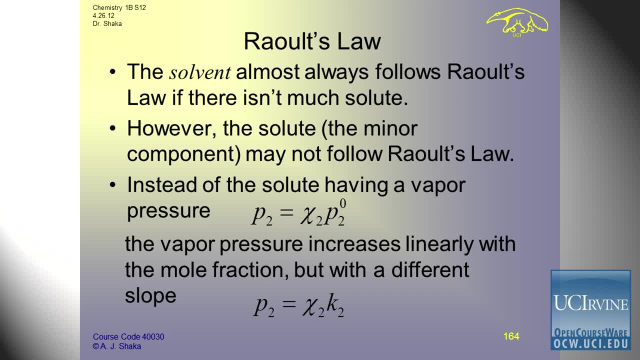 It's probably going to be pretty close to the pure solvent And it's just less of it, and so it's going to have less of a vapor pressure of itself. And that's because when you have hardly any of the solute, most of the solvent molecules- 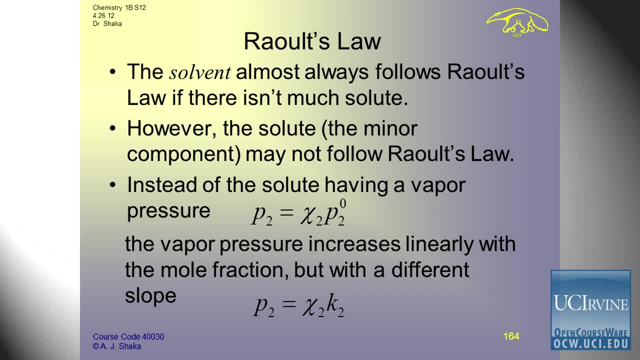 are just seeing themselves. If I have one micromolar of something and I'm there as a solvent molecule, I look around. I can't even see the solute. He's way over there, I'm surrounded by just my same old buddies. 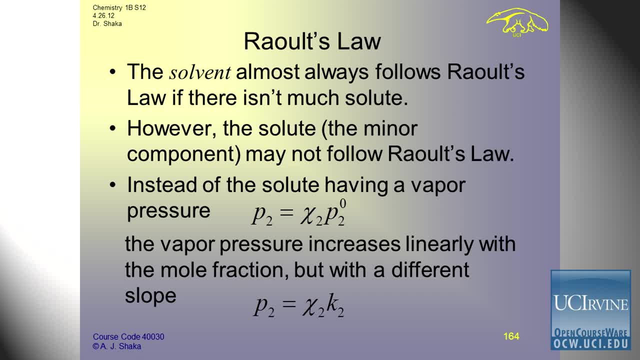 the solvent. and so I behave the same. If I'm going to go up, I go up. If I'm not going to go up, I don't go up. But the solute looks around: It is the black sheep in a herd of white sheep. 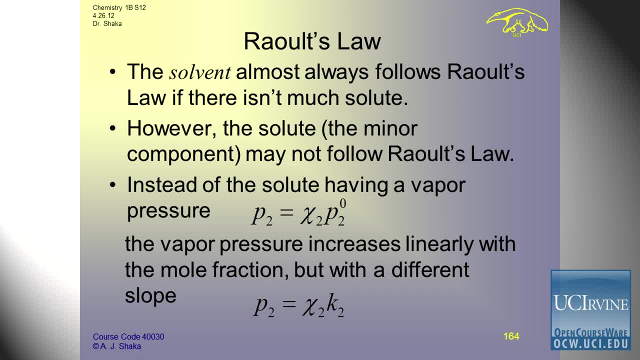 He's looking around and saying: hey, this environment is totally different than if all these molecules were solute. So oftentimes the solute doesn't follow Raoult's Law even remotely. So I've said that here. The solute, whatever the minor component, is. 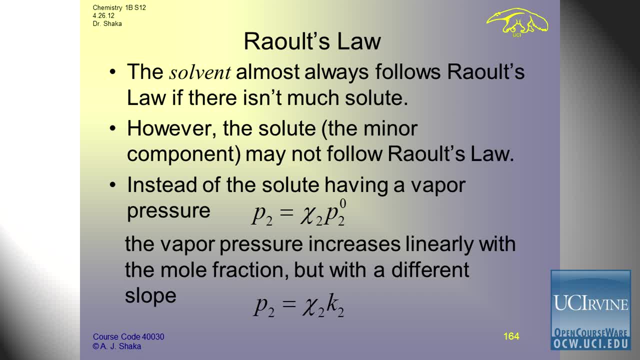 you have to be careful, because if you have two liquids, it's hard to decide who's the solvent and solute. But if it's dilute, the dilute one's the solute, even if it's another liquid. That's the convention. 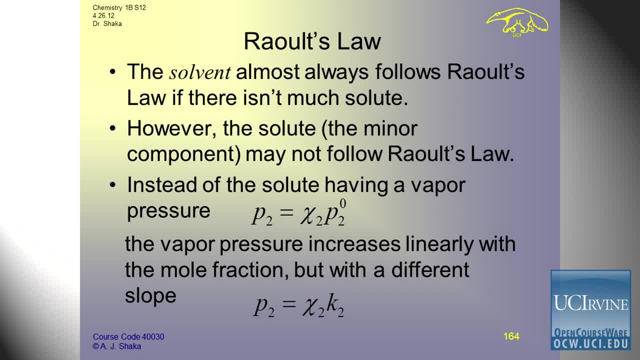 It won't follow Raoult's Law, but it does follow a line. The problem is, the line is different. So, instead of having a vapor pressure, the dilute one, instead of being proportional to its mole fraction, which is tiny, 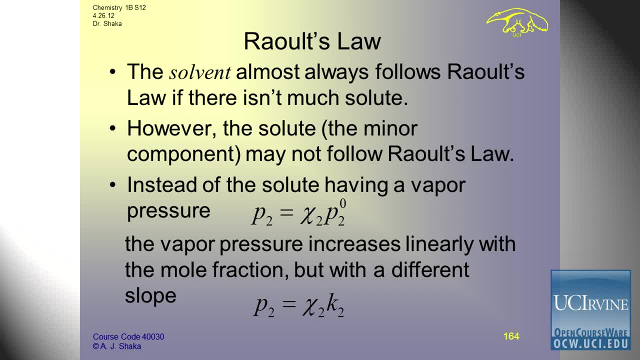 times the vapor pressure of the pure solute. it increases linearly. but it's not this value of pressure, It's this value, k2, which has the units of pressure, because mole fraction has no units at all. But the value of this pressure? 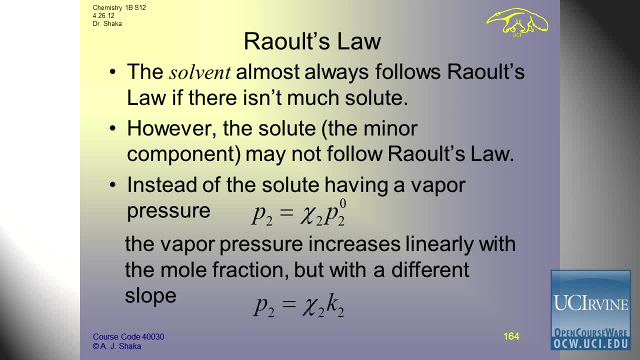 can be bigger or smaller, and sometimes by a lot compared to this one, And that's just because the solute may not be welcome The solvent. you throw the solute in. solute dissolves, but the solvent doesn't like it. 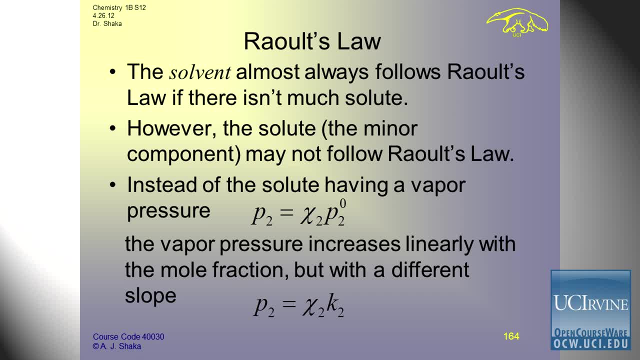 The solvent's saying: hey, why don't you just get out of here? It tends to push it up with a little bit higher force than if they were all solute. Then the value of k is higher. Or it could be that the solvent 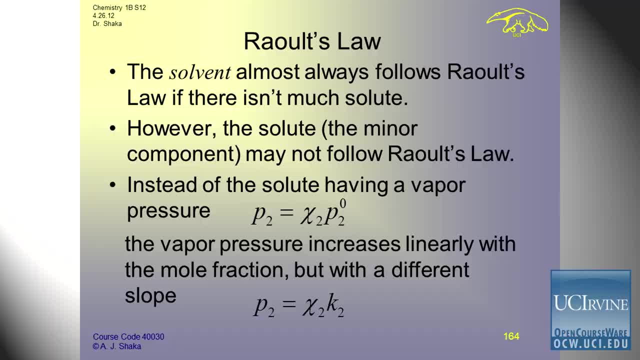 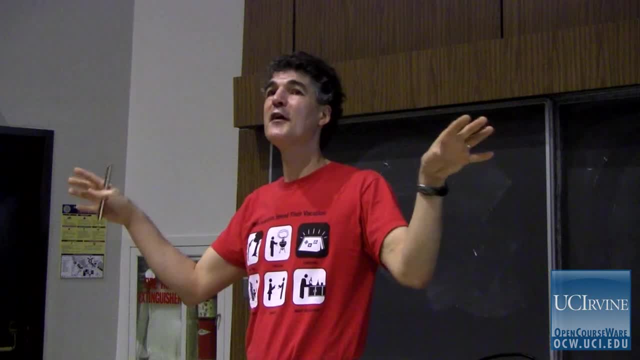 loves the solute, It says under no circumstances leave. I'm so tired of these other solvent guys here. Thanks, goodness, for a breath of fresh air. Stay down here, Okay, and interact with us, And then the vapor pressure is lower. 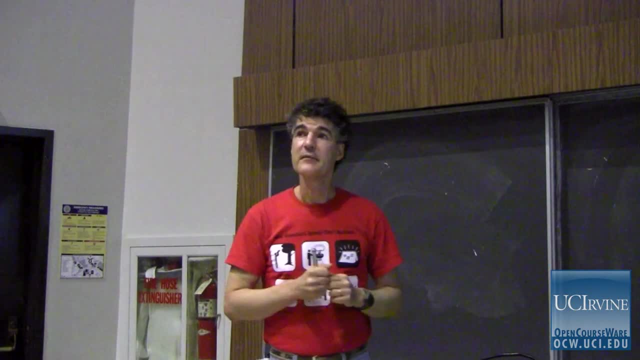 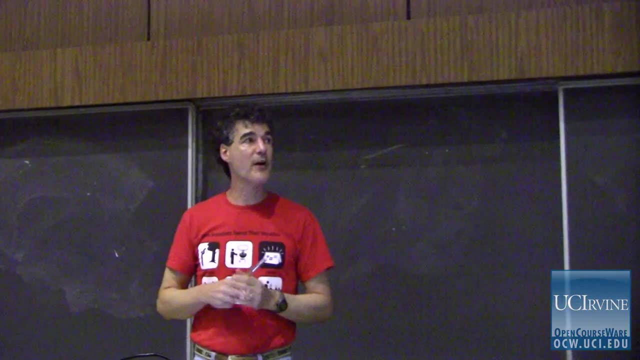 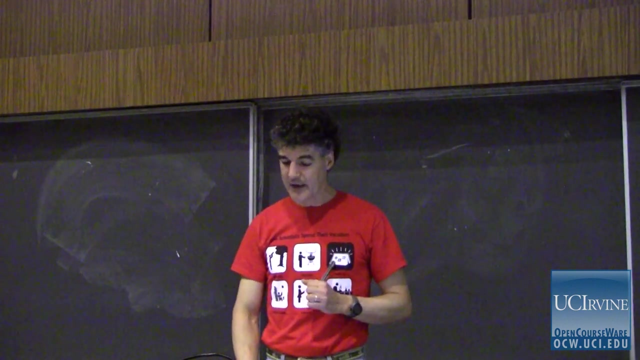 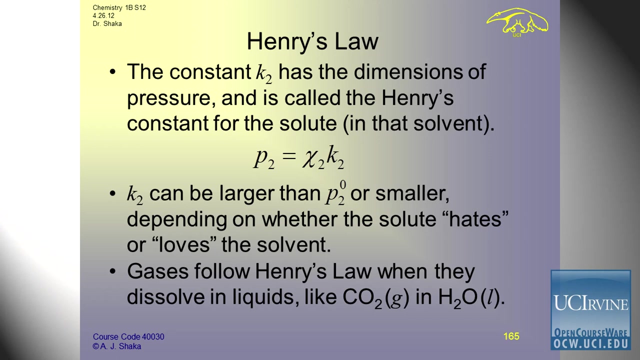 than what you would have predicted by an ideal solution. And then the value of k2 is again a pressure, but it's a lower pressure than the vapor pressure of the pure solute, And both cases occur And k2 is given a name. 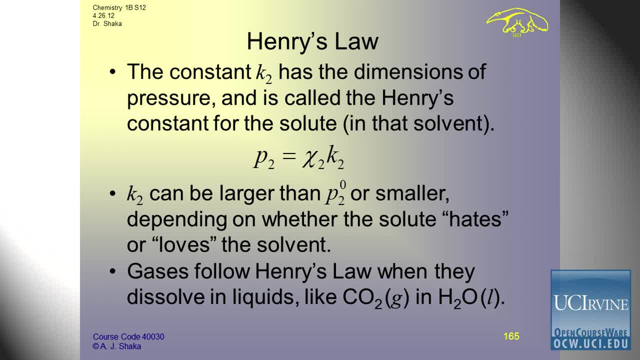 It's called the Henry's constant And this law that even for a minor component, that the pressure changes linearly with mole fraction, but just with the wrong slope. It's called Henry's law. And when two molecules are vastly different, one of them can hydrogen bond. 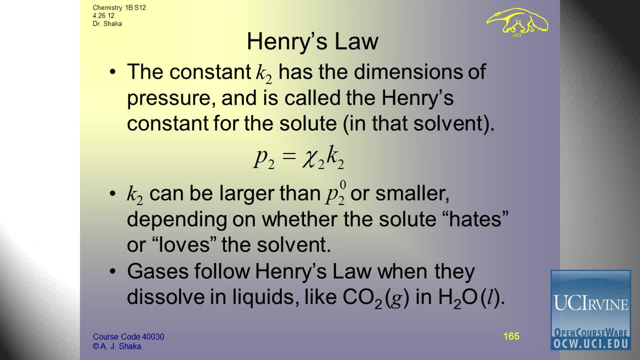 the other can't things like that. One of them has a lot of oily, greasy stuff and the other one doesn't- Then the solute will tend to follow Henry's law but not Raoult's law, And, as I just said earlier, 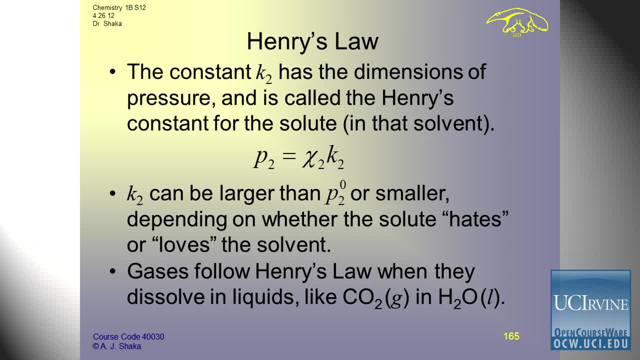 k2 can either be larger or smaller depending whether the solute hates or loves the solvent Gases follow Henry's law when they dissolve in liquids. For example, CO2 dissolves in water. That's how we can make carbonated water. 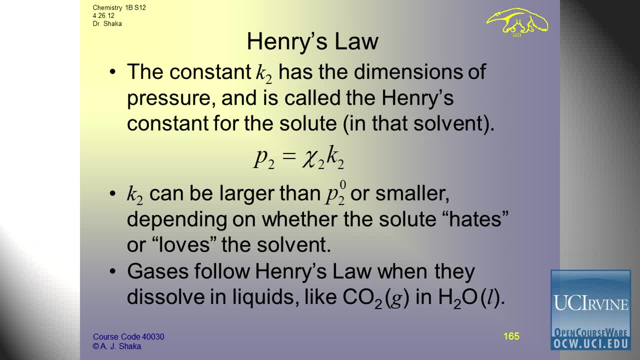 And of course, when you open a soda it's under pressure and it goes poof because some of the excess gas now sneaks out. And then you have dissolved CO2, which gives you the bubbles which people like And you can make your own. 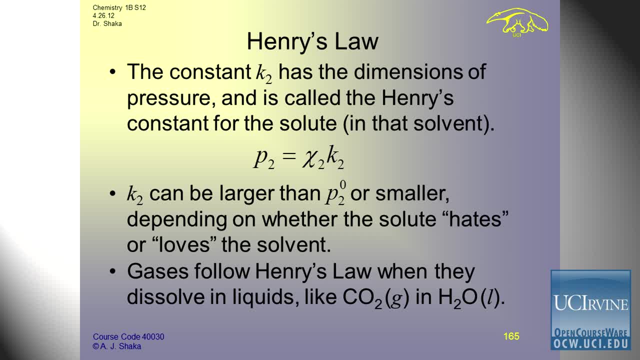 with CO2 and save a ton of money. But more to the point, this kind of calculation is ever so important if you start to argue about how much CO2 is going to dissolve in the ocean. The ocean is a lot of water, but we're putting in. 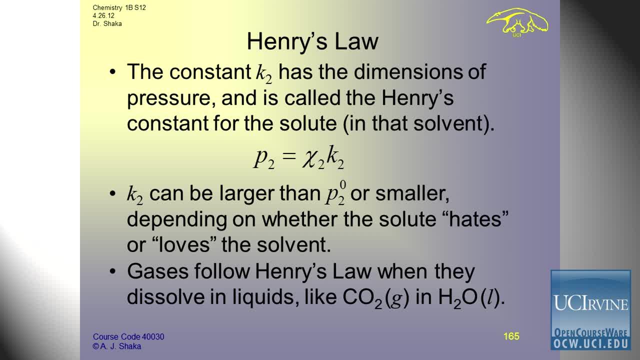 a lot of millions of tons of CO2.. You might say, well, maybe we could get out of the jam if a lot of the CO2 dissolves in the ocean, And some of it will. but if you want to figure out how much, 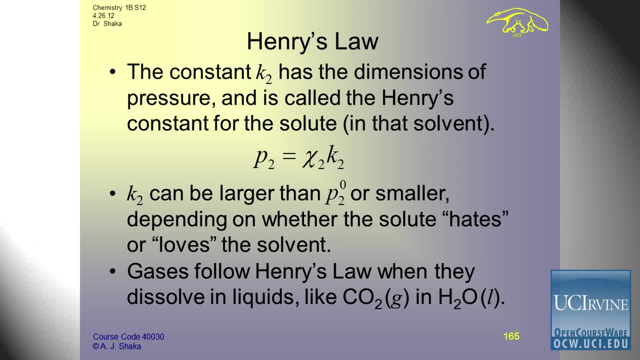 you have to know the temperature of the ocean. you have to know the Henry's law constant for CO2 and brine. you have to know the partial pressure of CO2 in the atmosphere. you have to know how much CO2 is already dissolved in the ocean. 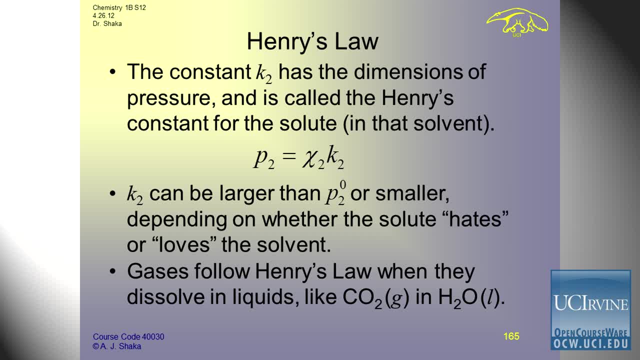 because if it's up to the top already, no more is going to go in and things like that And in fact we will dissolve more CO2 in the ocean, most likely- and that's already been picked up- because CO2 makes the water solution acidic. 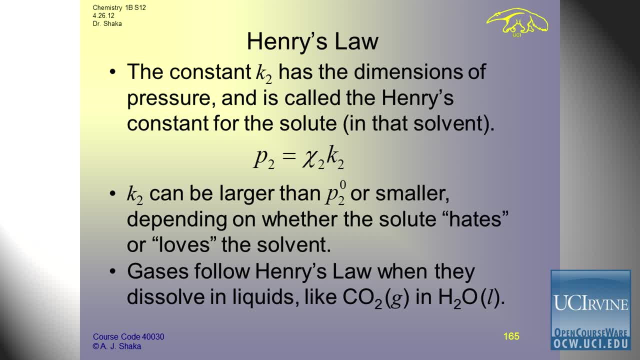 We get carbonic acid And in cases where the ocean becomes acidic, the calcium carbonate structures that many kinds of shells and coral reefs use to build up their structure dissolves. And when that dissolves, all the small guys who are hiding out there. 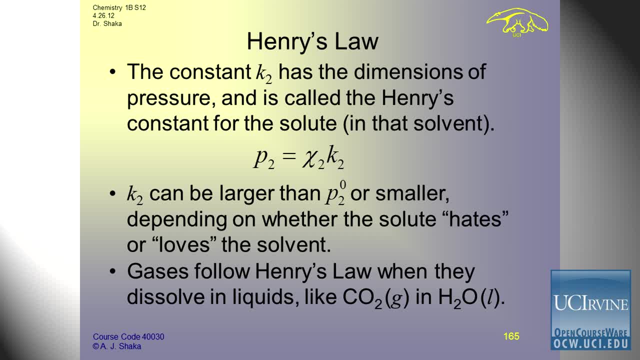 are out in the open, They're gone. And then, after they're gone, the big guys look around and say, hey, there's nothing to eat, And then they're gone And you can get a crash in the population When they first came to fish cod. 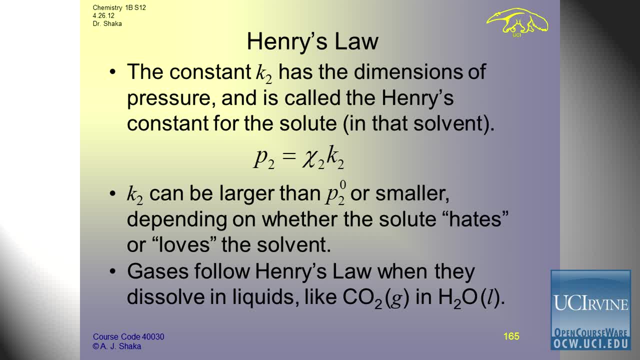 on the east coast in the Atlantic. there were so many cod in the ocean that they just said many times you could never possibly exhaust them. You just put a net in and you just get thousands of them. They're just everywhere And that's what they did. 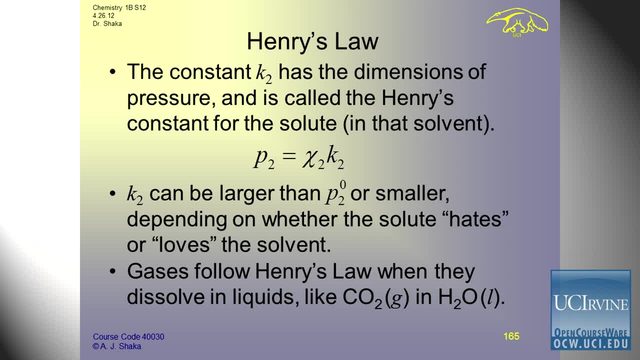 And now there's none there. There wasn't an infinite supply, It was quite finite. Lots of our food comes from the ocean, and so we don't want to one way or another, so we don't want to really pH the ocean. 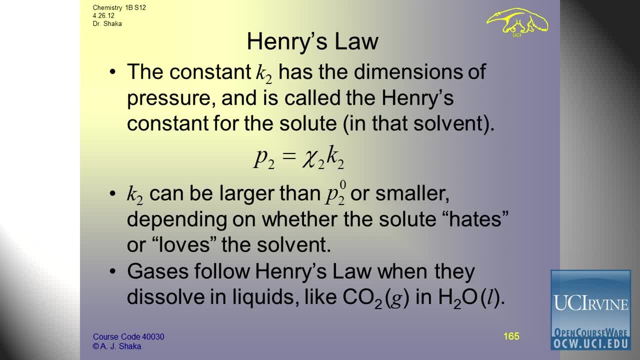 at some new value and try that experiment on a global scale and then find out we don't get the result we want, which could be far less food production. So, while you may think, well, that'll not be so bad for global warming. 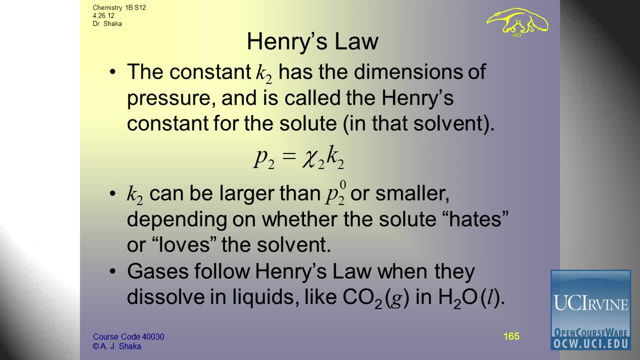 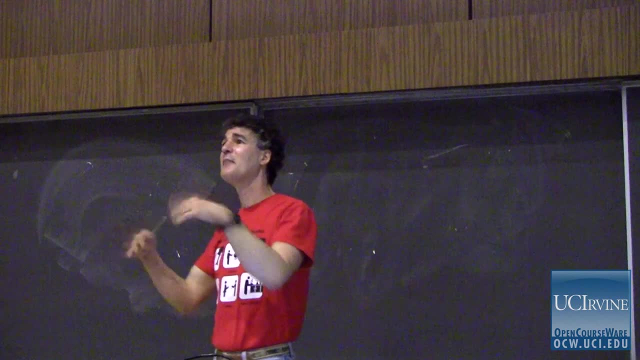 it could be very bad for global eating. And if you look at where people go fishing- now they're fishing the South Pole. They're pulling up all kinds of fish that you would never eat before and they grind them up and they call them- I don't know- crab. 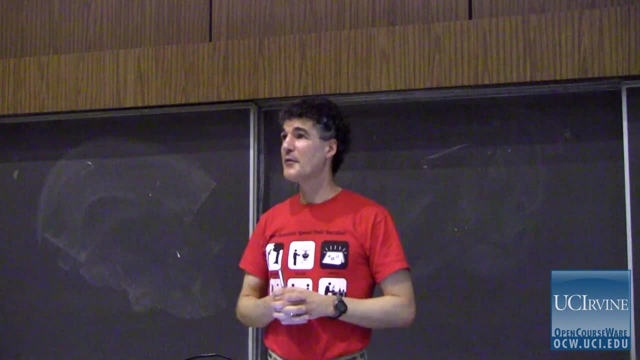 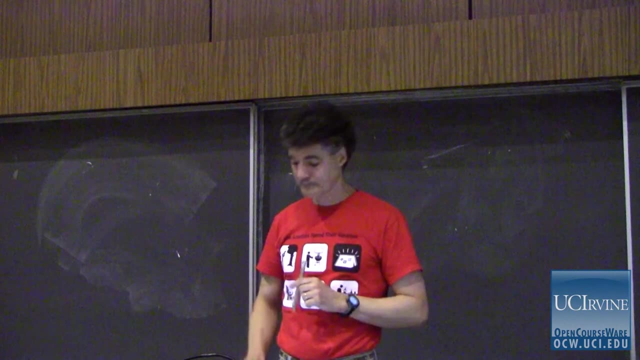 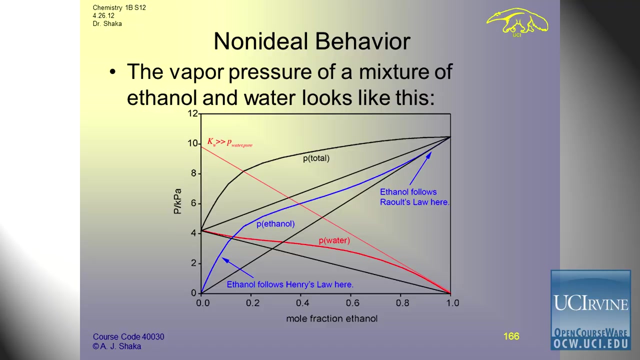 faux crab or something, and they serve them up to you, And they're now fishing those guys out too. So it may be that there won't be any fish at all, as is the case for some kinds of tuna. So here's a mixture of ethanol and water. 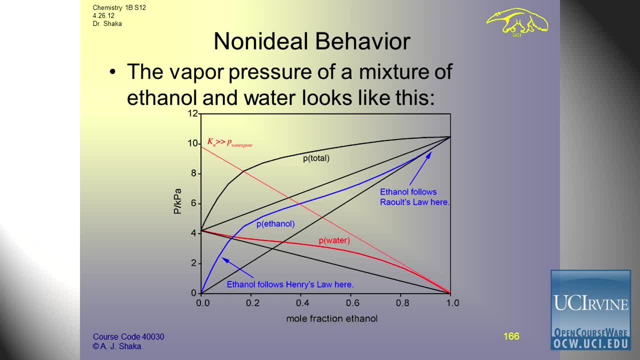 Chemists love mixtures of ethanol and water. Here is the mole fraction of ethanol. Here, when the mole fraction of ethanol is zero, it's all water. And as I increase the mole fraction of ethanol, the vapor pressure of ethanol goes on a straight line. 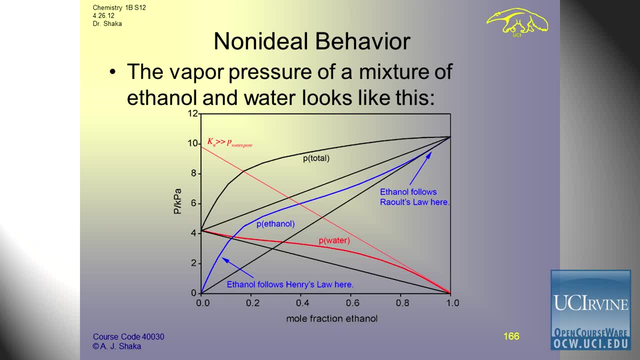 This is pretty straight, But the slope is not. This is the vapor pressure of pure ethanol. The slope is higher, In other words the water's pushing out the ethanol more than if it were just pure ethanol. And that's why, if somebody has a drink, 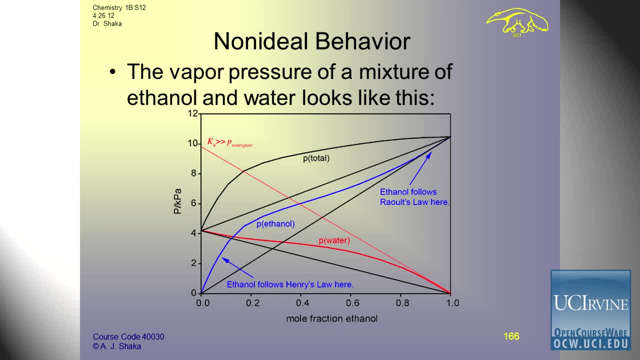 your mom can tell, because the alcohol comes out on your breath on a much higher level than you would expect And the human nose can pick that up immediately, especially parents. They have a nose. If you look at water in pure ethanol, it's the same thing. 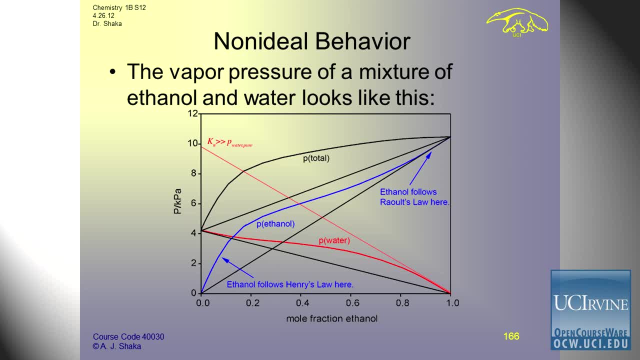 Pure ethanol says to water: get out, Go on. We're happy here. We don't want you cluttering around. We've got our interactions here with this hydrophobic methyl group. Get out. And so the water when it's in almost pure ethanol. 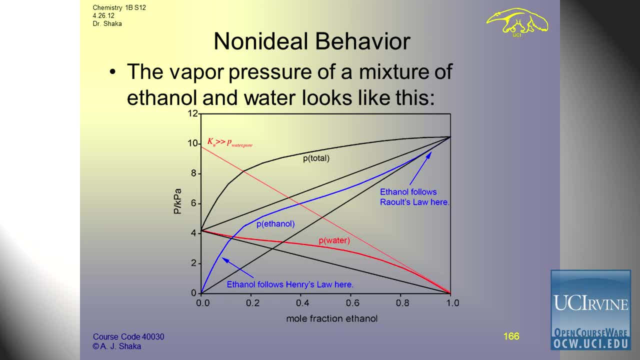 follows a law but the apparent vapor pressure. this is the Henry's constant. I've called it Kw here. The Henry's constant is the slope near here and it's way higher than the pressure of pure water which is on this. 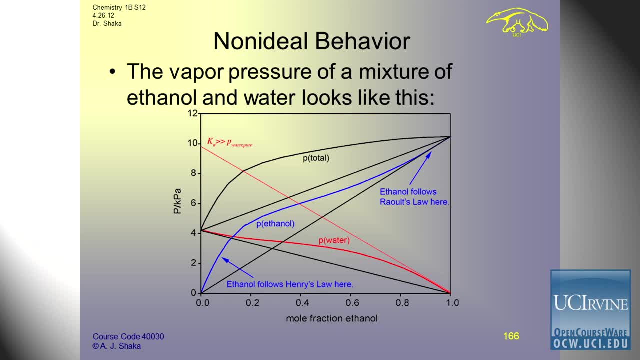 On the other hand, when we look at the pressure of water, when it's almost pure water, the mole fraction of ethanol is zero. it follows Raoult's law. It's linear up to pretty good concentration and it goes right down to zero. 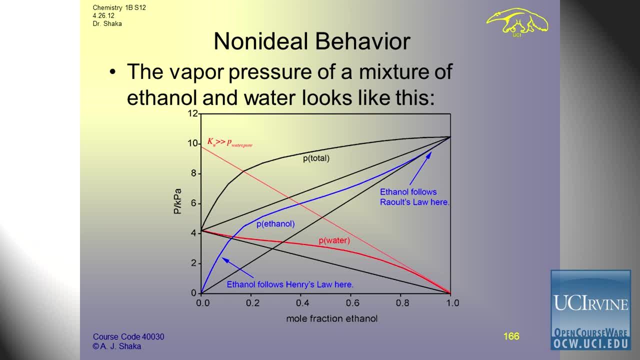 So it's following that line And likewise, when it's pure ethanol, it follows this line here. that goes down here and it has the right slope here. If the solution were ideal, we could add up these lines and we'd get this line. 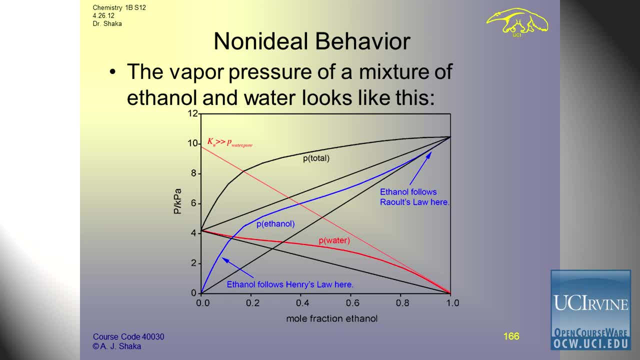 And this is Raoult's law. If ethanol and water followed Raoult's law exactly, they'd always be on that line. But it shows a higher, a higher amount of total vapor pressure. They dislike each other And so we get that funny curve. 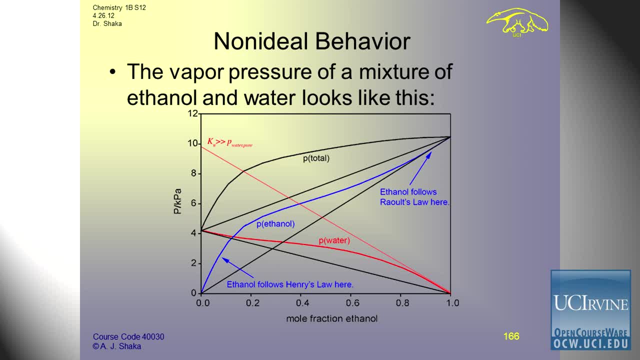 And that's the signature of a non-ideal solution. This solution is not very non-ideal, but it's kind of a good textbook example. You can mix them in any amount, but it starts deviating from the ideal behavior. Now we can use this. 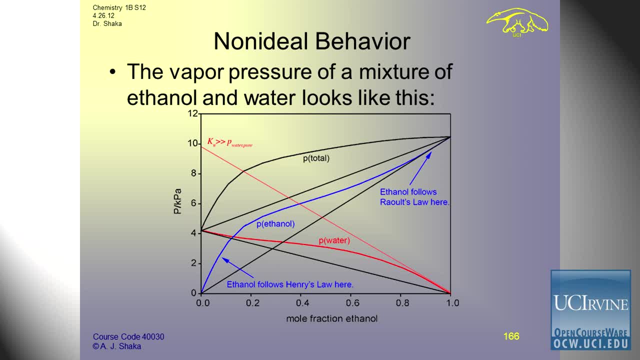 because ethanol has a higher vapor pressure than water. So if we take a mixture of ethanol and water and we heat it, the vapor is going to have more ethanol in it than water, And the Scots figured this out a long time ago, so they would take just stuff that they had fermented up. 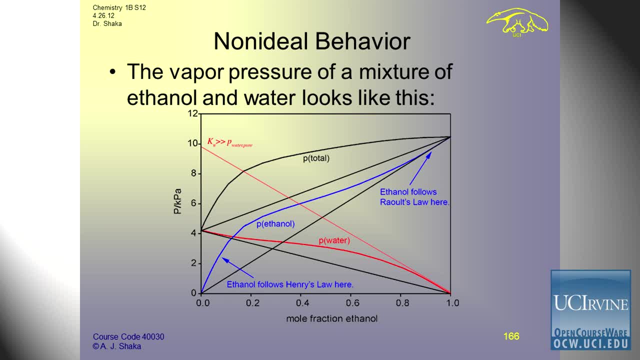 which tastes awful, and they would distill it, And they would make distilled spirits Which were much, much stronger than beer and very habit-forming, And they'd come out with this stuff. that's a clear stuff. that's the worst stuff you've ever tasted. 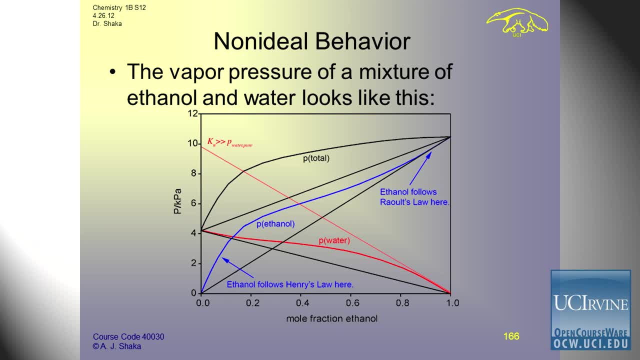 Unless you've tasted moonshine from Tennessee, or hand sanitizer or whatever the latest trend might be. If you want to look desperate, be caught distilled or distilling hand sanitizer, That'll do it, But then what they do is they take that distilled liquor. 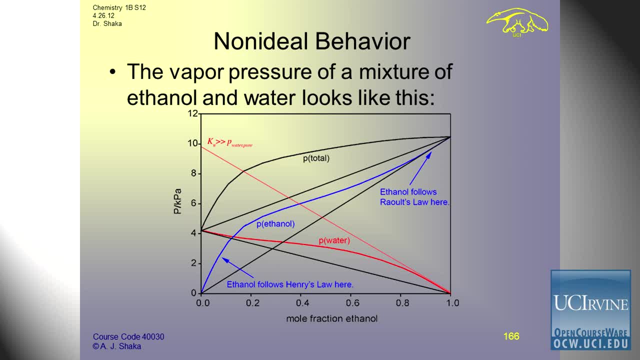 and they put it in some oak barrels And they just let it sit around 20 years And you get some very slow chemical reactions And all the bad stuff, the hard stuff, goes away And you also leach some very aromatic compounds out of the wood. 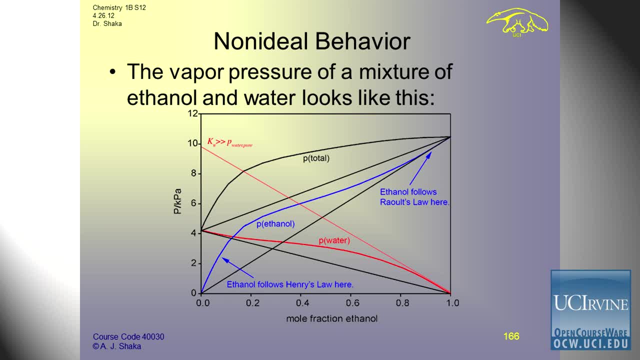 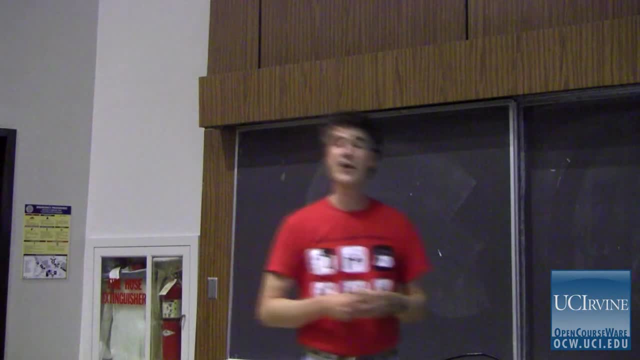 Usually you use an old sherry barrel So you get some of the sherry flavor That turns it a golden color And then it's quite delicious in small amounts. But since it takes 20 years to do that, scotch is expensive. Because how do you plan 20 years ahead what the demand will be? You just make some and then, if it turns out really good, it becomes very expensive Because everybody wants it and there's no more to be made. It's already been made. 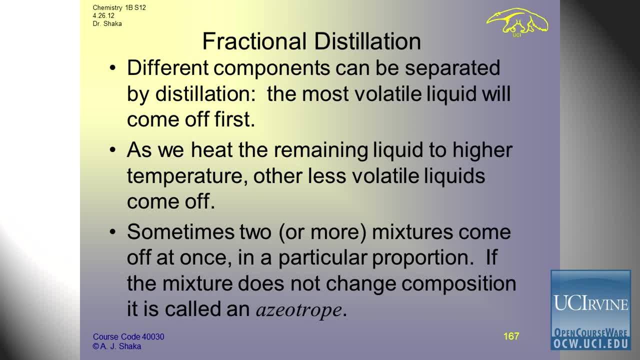 Well, we can separate by fractional distillation these components, And the ones with the highest vapor pressure will come off first. And when they're distilling, making distilled spirits, they have a thermometer there and they don't let the temperature get above a certain level. 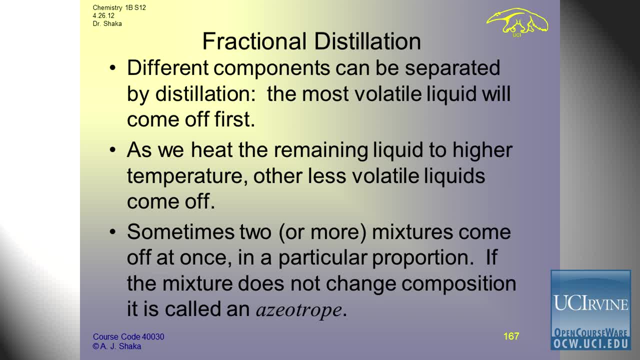 Because if you do, then you start boiling over all these awful things- Fusel oil and other things- which will give you a whopping headache because they're much, much more toxic than ethanol. But if you're just moonshining, you probably don't bother with a thermometer. 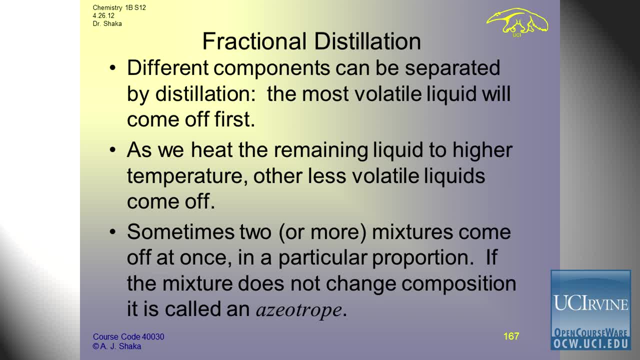 and you get what you get. And if we keep heating it, what'll happen is the temperature in the liquid will keep rising and we'll get- we'll get- less and less volatile things. So if we've got a mixture of a thousand things, 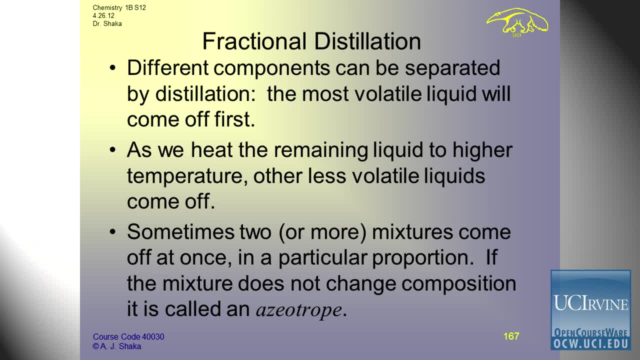 we can try to separate them by distilling them. We first make the temperature low and we collect something called a fraction. We collect five percent, And then the temperature goes higher. otherwise nothing else comes out. So we heat it up more. 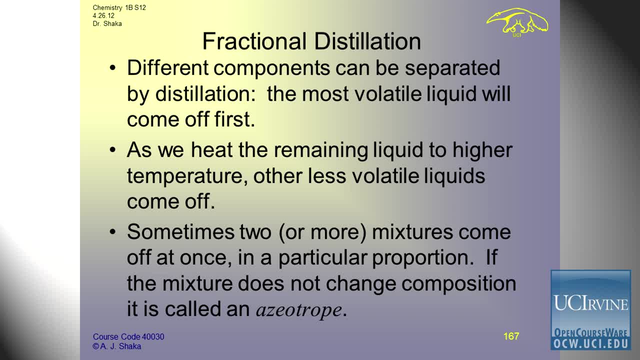 then we get the next fraction and so forth, And that's called fractional distillation. Occasionally two things come off together, And when that happens you've got something called an azeotrope, if it doesn't change composition. 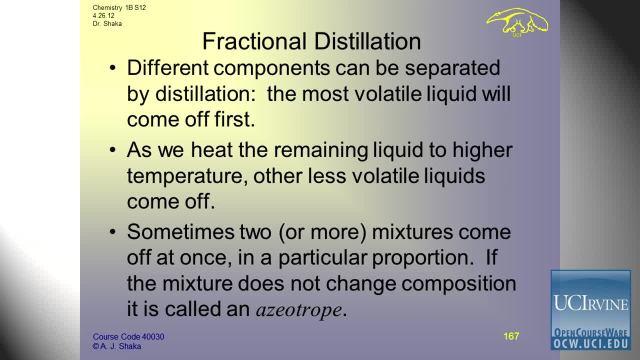 And that's how they denature alcohol. They add something to the ethanol so that if you try to distill it, the something they add comes off with it. And the something they add is usually poisonous gasoline or something small amounts. 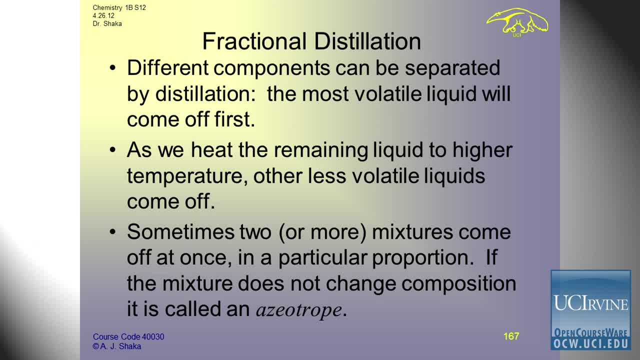 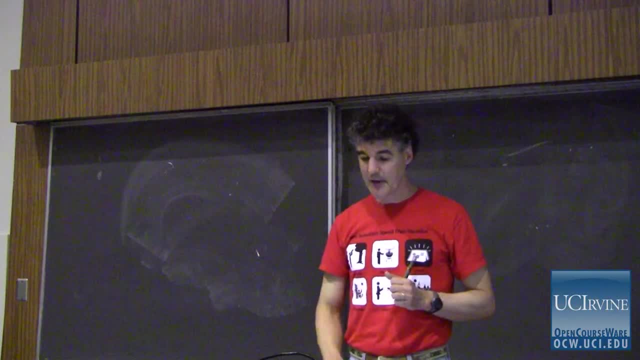 And then you don't have to pay the tax, but you have to pay on drink. Okay, Because you can't drink it. Same thing with Listerine: You put in a ton of thymol and eucalyptol. 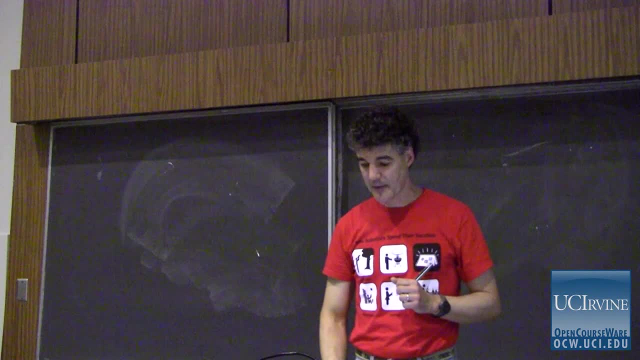 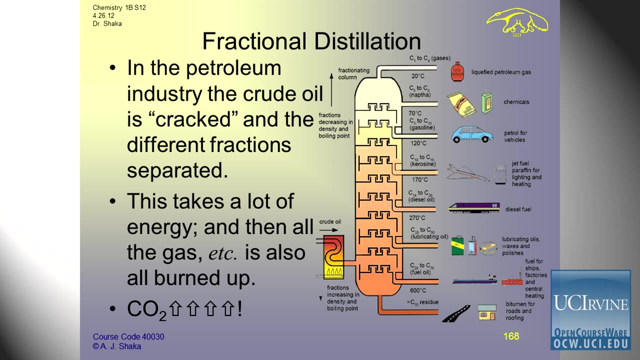 and you can't drink it. It'll be very unpleasant. In the petroleum industry. they do this thing on just a massive scale. These columns they have are gigantic And the amount of energy that they use to do the fractional distillation is just absolutely staggering. 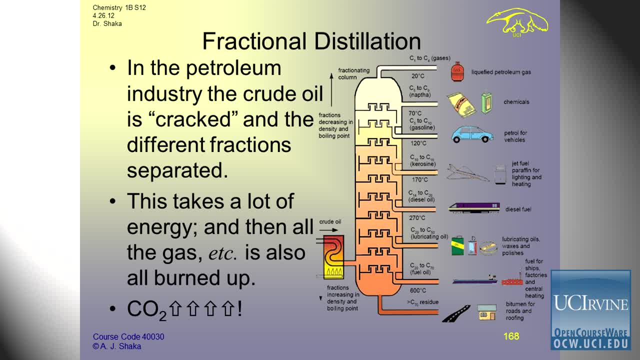 In comes the crude oil- 10 million barrels a day. All of it gets boiled up by some means. That is a lot of energy going into that. So we heat that stuff up and we get various fractions. Here we get diesel oil. 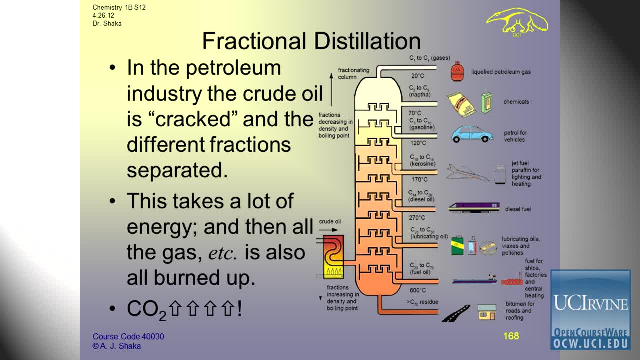 Here we get kerosene, That's jet fuel. Here we get gasoline for cars, Here we get naphtha, That's for the fine chemical industry. And then at the top we get gases which they tend not to like because they tend not to like to handle gases. 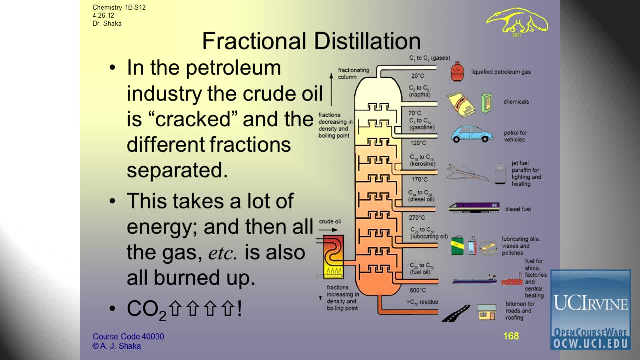 And so the gases. sometimes they just burn them off, Just flare them off. Total waste Not worth enough money to hassle keeping it, Which is astounding, but it's been true for a long time, If you go up to Montana, North Dakota now. 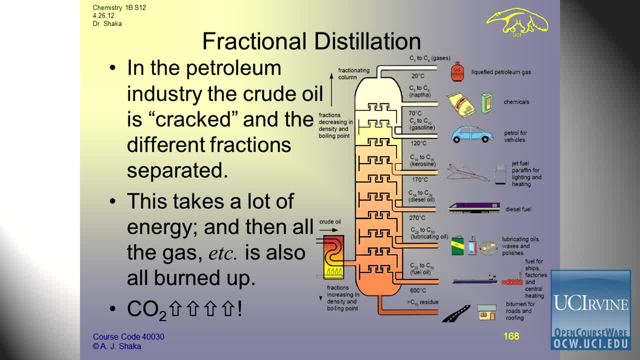 where they're drilling, drilling, drilling, drilling all these wells. they're just flaring off the natural gas, The methane, Just big flames sitting there doing nothing, Going up into the sky adding a fair amount of CO2.. And then you get some real bad actors down here. 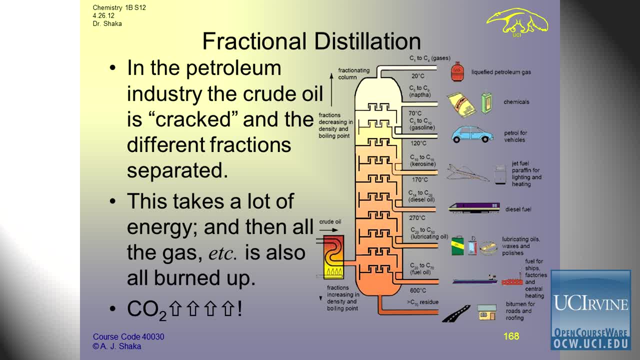 that are really heavy down here And this you use for ships- the so-called bunker fuel. And these really big ones asphaltane. those are like the bitumen in the pit: straw, black as pitch. That's what you use to pave the roads. 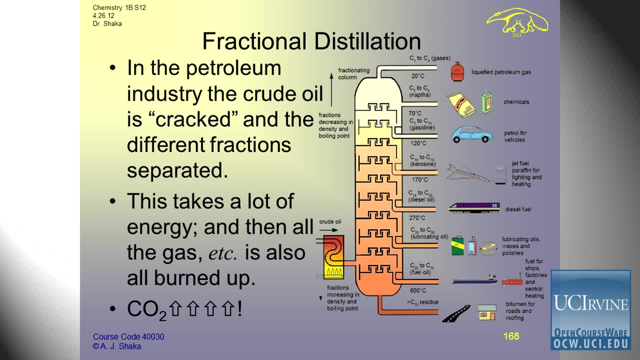 You separate all that out, But for every barrel of oil you boil up the whole thing. How do you do that? With another barrel of oil, or with this gasoline you've got, or whatever? Or these days you might use natural gas. 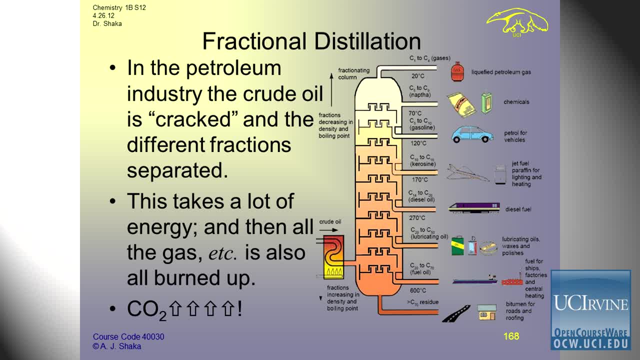 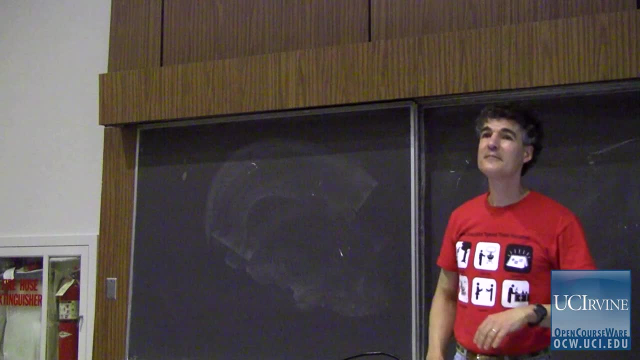 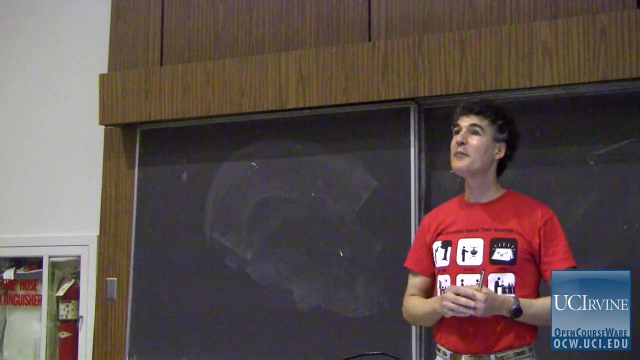 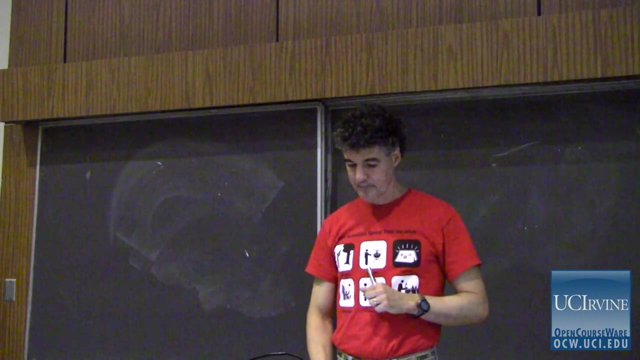 But still all that is producing a lot of CO2.. And then, after you take the oil and you fractionally distill it and you do all this stuff, you then burn all of it too, Or the vast majority, So the CO2 just goes up, up, up, up up. 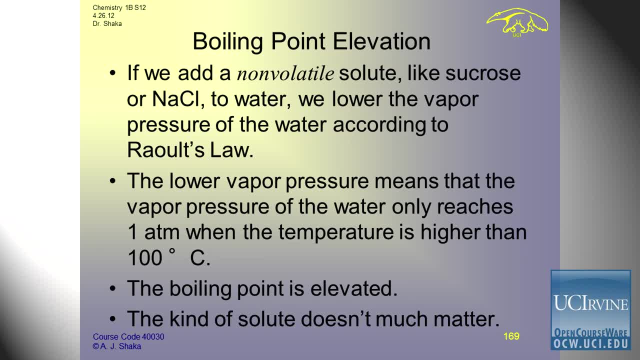 Okay. now if we add a non-volatile solute like sucrose or sodium chloride- by non-volatile I mean that at room temperature its vapor pressure is so low that you can't measure it- Then we lower the vapor pressure of the water. 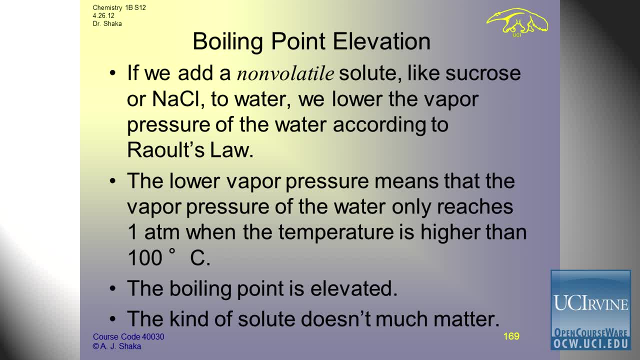 or the other solvent according to Raoult's Law And the lower vapor pressure of the solution. the other thing contributes no pressure, But when I put it in I lower the mole fraction of the solvent. so now the solvent has lower vapor pressure. 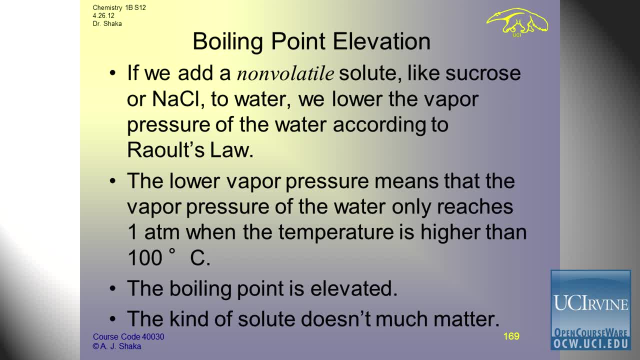 What that means is that to bring the vapor pressure up to one atmosphere, I've got to go to a higher temperature, Because where it was one atmosphere when I throw in this solute it's now lower And that means it boils at a higher temperature. 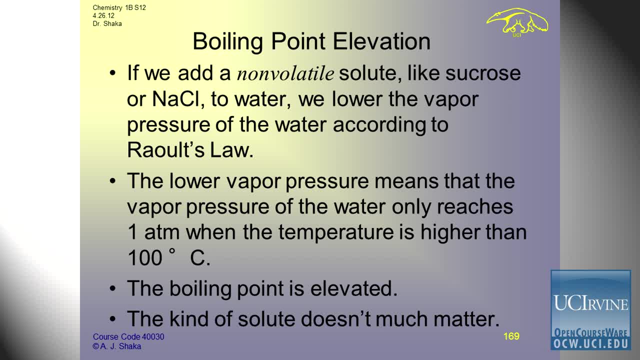 and that's called boiling point elevation. If I add salt to water or sugar to water, and I add quite a bit, it's going to boil at a higher temperature than just pure water. So the boiling point is elevated. It's always elevated. 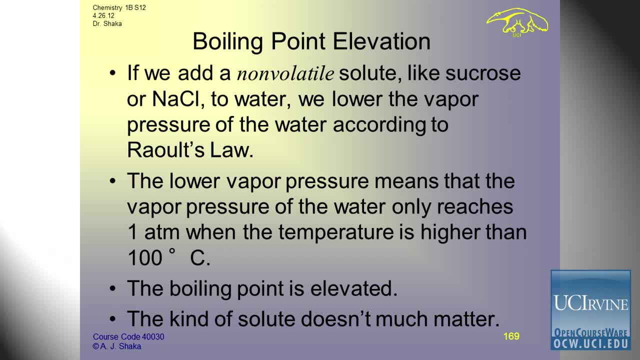 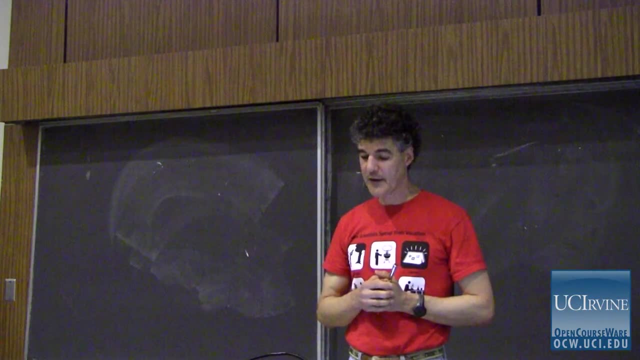 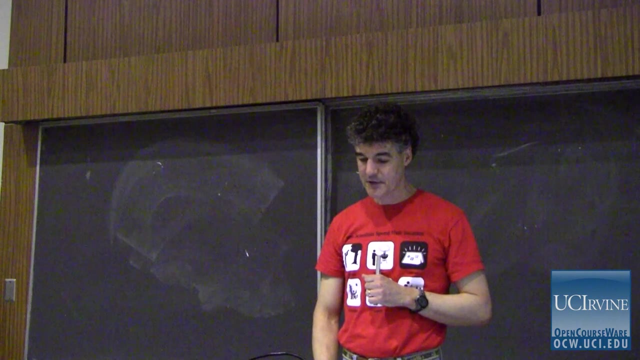 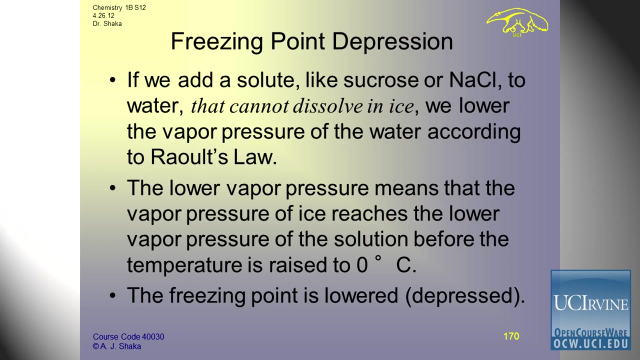 if the solute is non-volatile. The kind of solute doesn't matter much, It just has to do with lowering the temperature. We'll see that we can measure the molar mass this way by just changing the boiling point If we add a solute like sucrose. 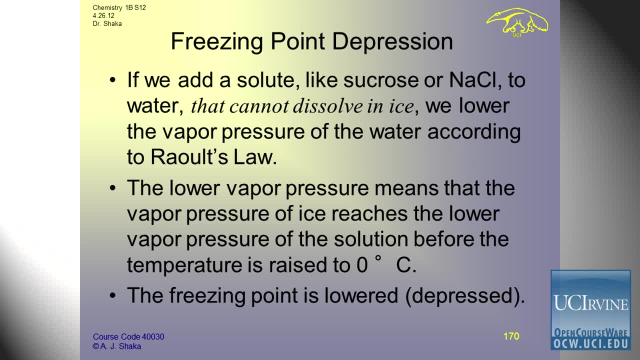 or sodium chloride to a solvent like water, and these guys, sucrose and sodium chloride, cannot dissolve in ice. That seems like kind of a funny thing to say, because these molecules dissolve in water. Water's disordered as a liquid and they just roam around. 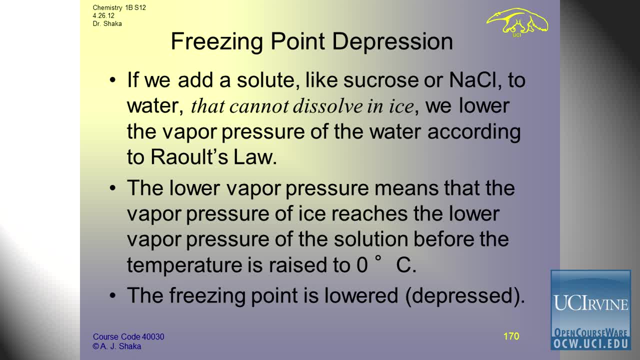 But when water starts forming a crystal ice and locking together, it keeps pushing the sucrose or the salt out into the solution. It locks together and the ice you get from salt water is still pure. Therefore, if you freeze ocean water slowly, 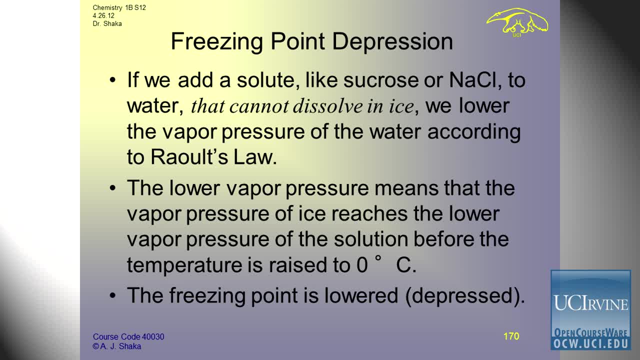 you can get fresh water from it, So the icebergs are all fresh water. They could be ocean water that froze slowly, but there's no salt in the iceberg. There's salt on the surface. So far it's not a commercially viable option. 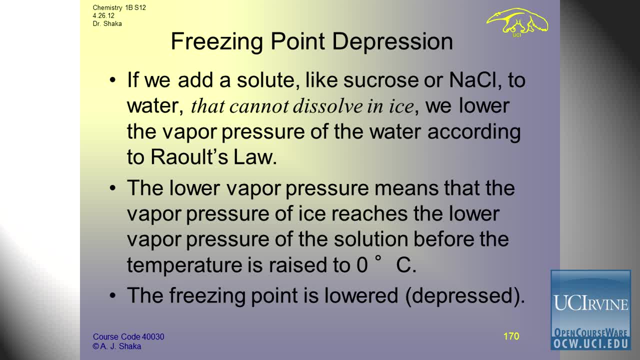 because the problem is washing all the salt off, all the ice cubes you get and hassling around with that. But it's theoretically interesting and if somebody works on it it could be useful. It's a lot easier to freeze water energy-wise if you're in a cold place. 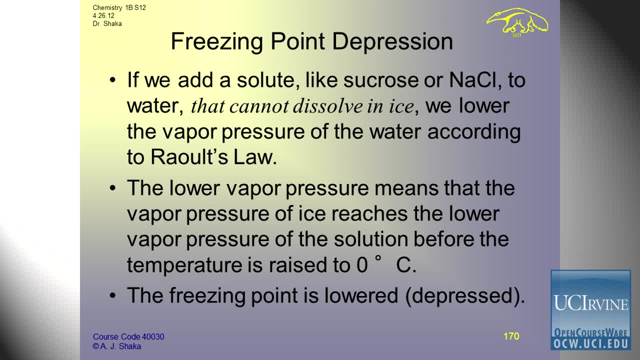 than it is to boil the water and then desalinate it by boiling all the water. So if you want an energy-intensive thing, get a couple of cubic miles of seawater and boil it all of it until you boil it all over. 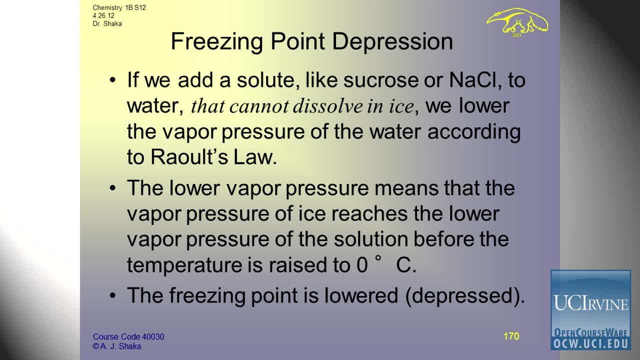 and you've got nothing left but salt. That's going to take a ton of energy to do that And the lower vapor pressure of the solution, because the ice is pure. the ice is the same vapor pressure And normally you don't think of 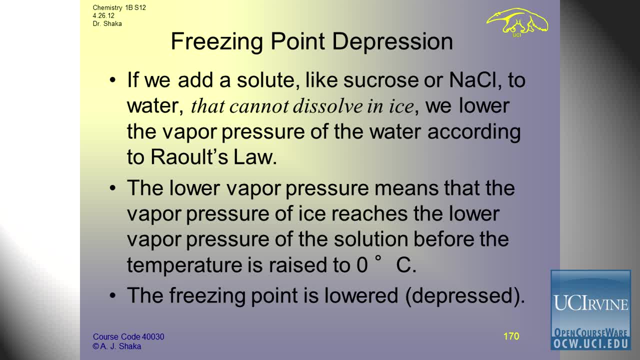 vapor pressure, ice water. what is he talking about? But consider it this way: Let's physically separate the solution of salt and the ice cubes that are floating in it And let's put them in two beakers and put them separate them. 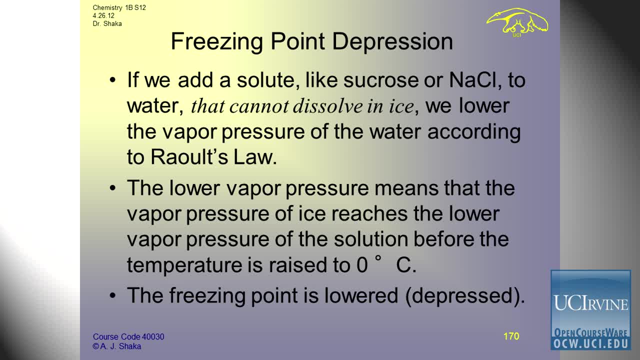 under an evacuated bell jar. They're separate anyway when they're in there because the ice is pure. But let's do it this way: The ice has a certain vapor pressure. It's equal to the vapor pressure of pure water right at zero. 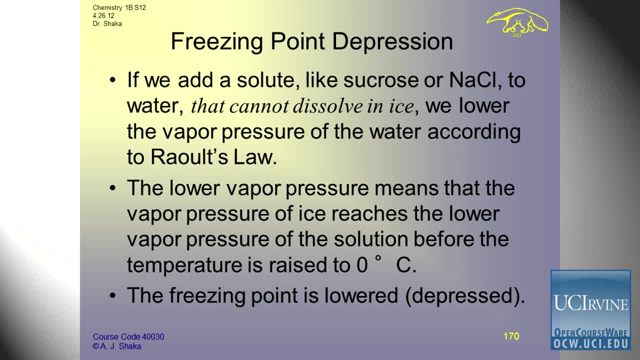 That's why, at zero, the ice doesn't melt or disappear over to the water and the water doesn't freeze, disappear over to the ice. The solution now has a lower vapor pressure, So that means that the ice actually is pushing out more water molecules. 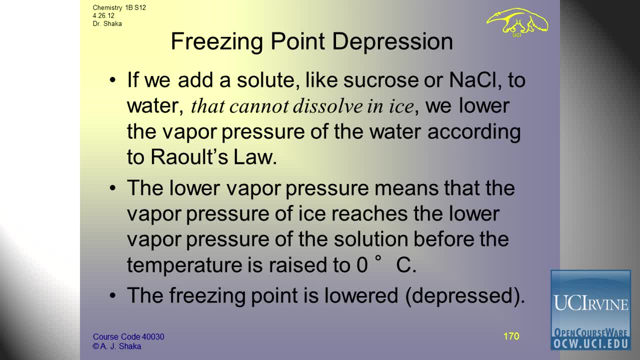 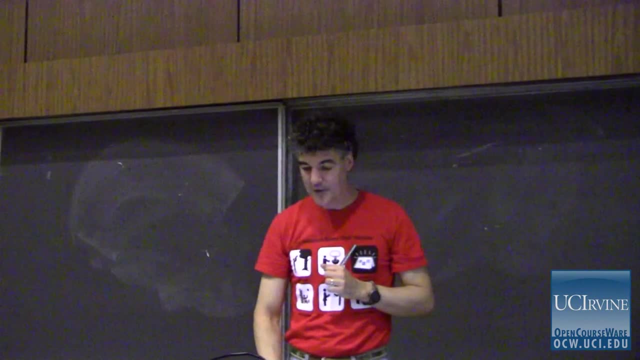 than the solution, And that means that the ice ends up going over here or it's got a lower melting point, So it's going to be lower than just the pure solution, So it's going to reach that point. It's called freezing point depression. 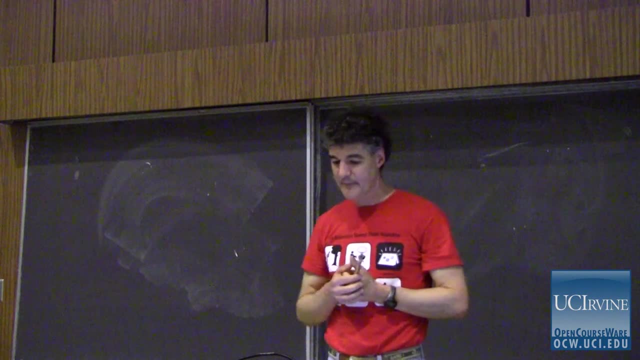 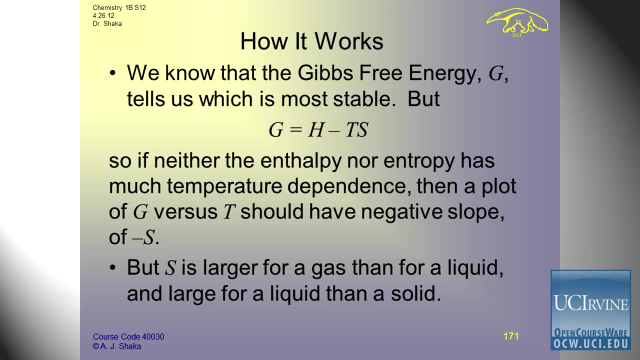 Now, how does it work? Well, I don't know if you've had this equation- I think you may have, but it's delta G, named after Gibbs. It's the Gibbs function that tells you what you're going to get at equilibrium. 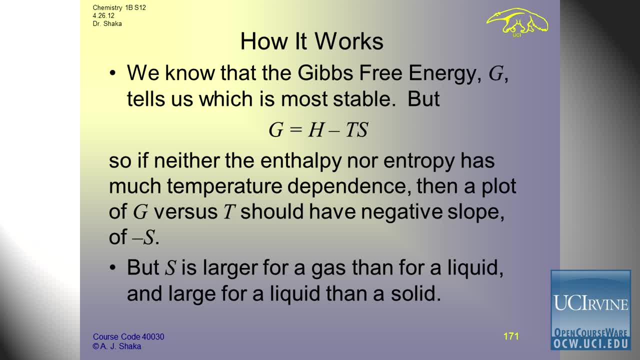 And if we say that the free energy is equal to the enthalpy minus the temperature times the entropy, then if we plot G versus T and H and S don't depend too much on temperature, which they often don't, then the plot of G versus T. 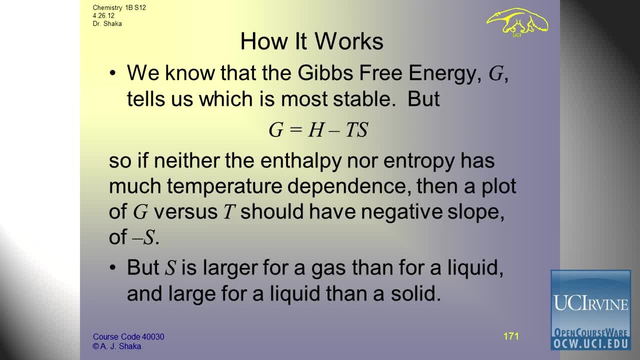 should be a straight line with slope of minus S. S is the entropy, That's the lowest for a solid, So the slope is the least negative for a solid. S is higher. for a liquid, The slope is more negative. S is very high for a gas. 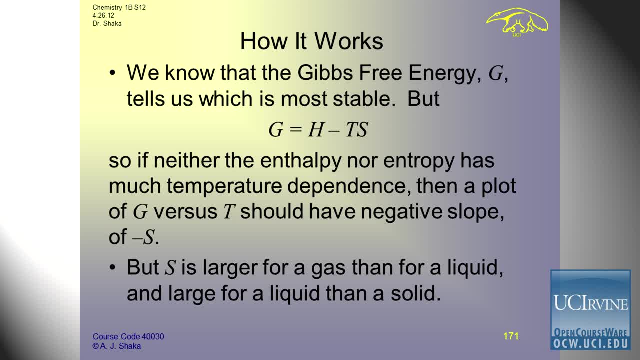 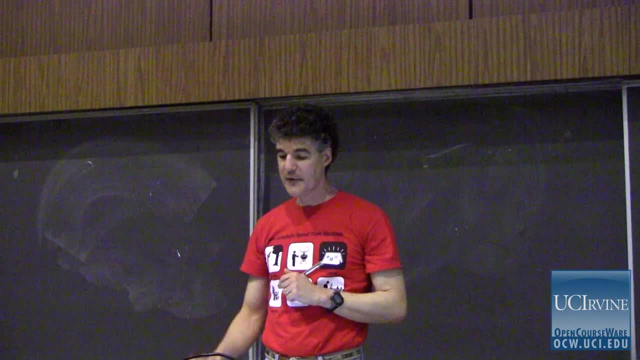 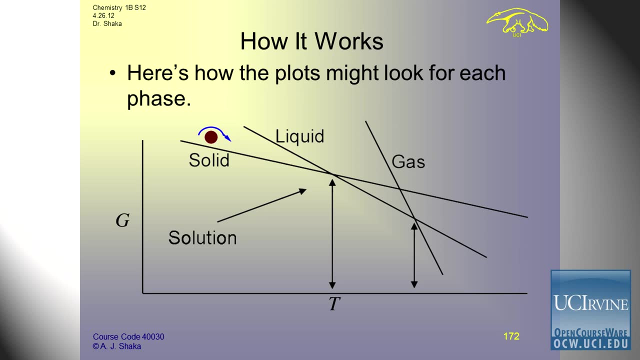 The slope is extremely negative. Well, suppose I plot the slopes for these three phases and have a look at what happens. Well, here it is. The system rolls downhill just like a ball. At very cold temperatures it's a solid. As I heat it up, 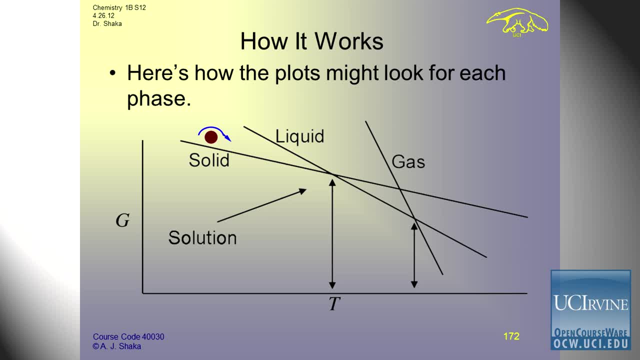 the Gibbs function of the solid goes down, down, down, down, down, down down. And because the Gibbs function of the solid is lower than the liquid or gas, it's solid because it already fell down to this level, But when it reaches this point here, 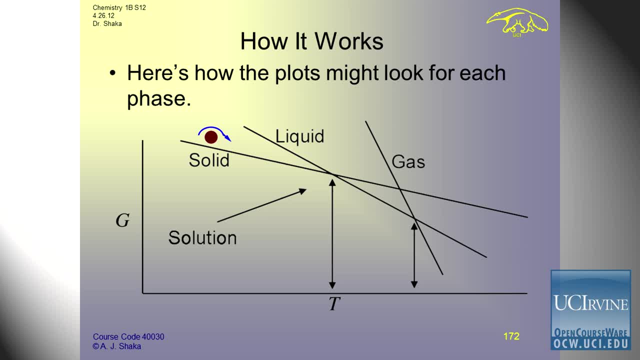 it's going to melt because now the solid's going this way and the material says: hey, I can lower my Gibbs function much faster by turning into a liquid, which it does until here, And then it intersects the gas, and then after that it says: 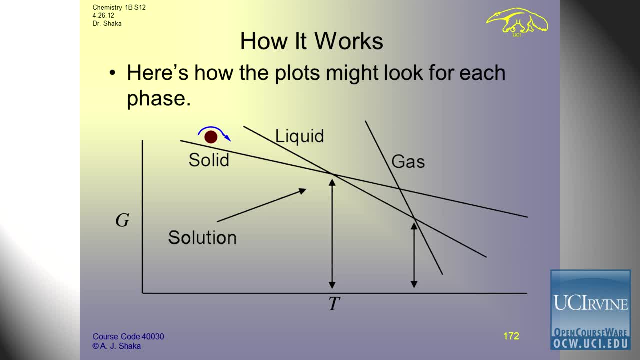 down I go. I'm a gas And these two points are when it freezes and when it boils, if I'm following it heating up. Now, if I have a non-volatile solute, it doesn't change the gas, and if it doesn't dissolve in the solid. 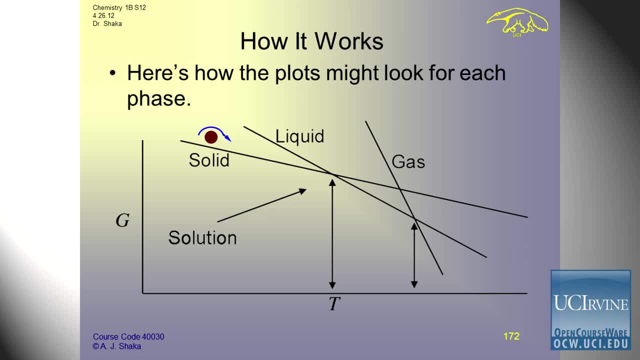 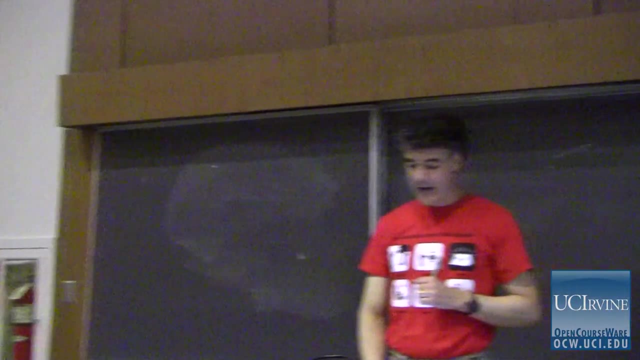 it doesn't change the solid, but it does lower the G of the liquid because the G is related to the pressure. Remember I told you pressure was energy per unit volume, so it has something to do with how much oomph it has, and it has less oomph when it's a solution. 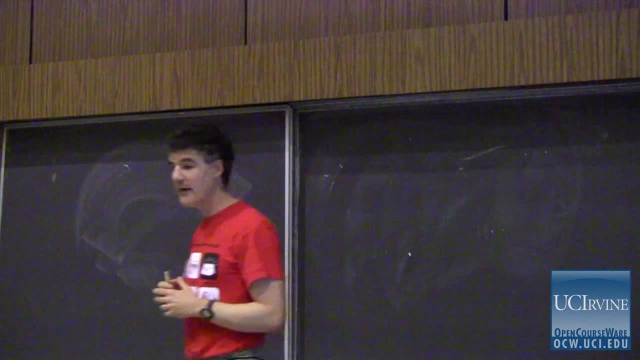 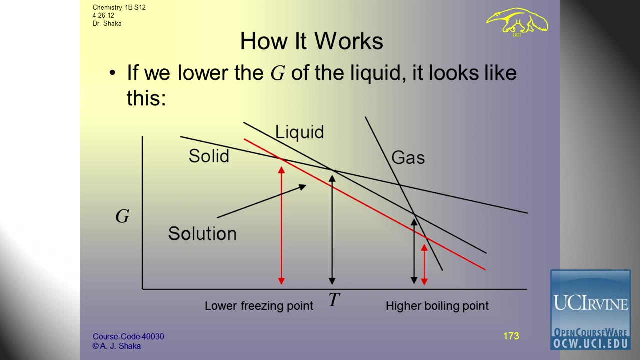 And so what happens then is the liquid moves down, and for simplicity, I've kept it the same slope. The solid doesn't change because the solute doesn't dissolve in the solid. If the solid moved down by the same amount, there wouldn't be any change. 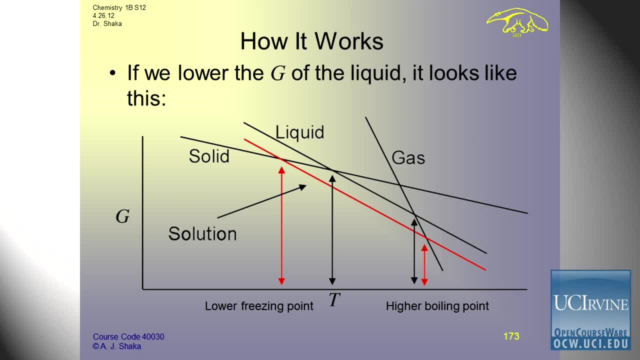 It would be here again, And the gas doesn't change because the solute doesn't go into the gas, It's non-volatile, And what we see then is now the solid to liquid. it hits this red line and then it says: 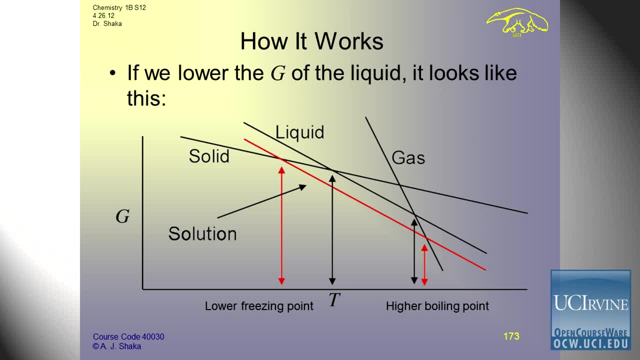 wow, I'm going to turn into a liquid. But it doesn't hit this black line until higher. So there's a lower freezing point and it's usually bigger because these are less of a slope And a higher boiling point, but it's only a little higher. 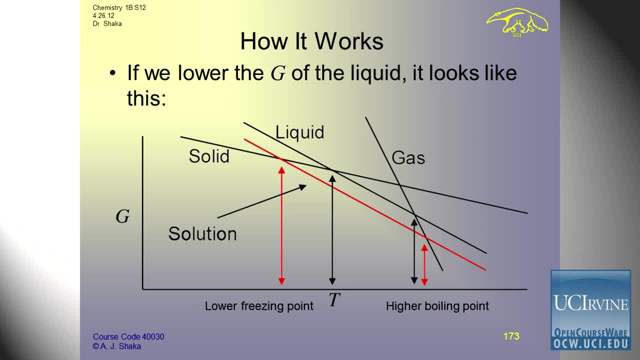 And therefore usually if you want to use this colligative property, you focus on the freezing point. You don't like putting your molecules in boiling solvent because your molecule may react, It may fall apart or something bad may happen to it. But usually if you're putting it in freezing, 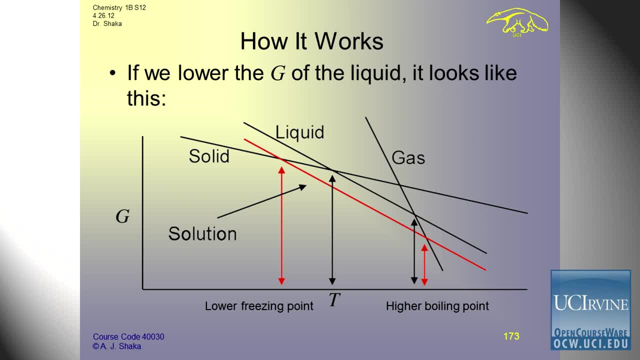 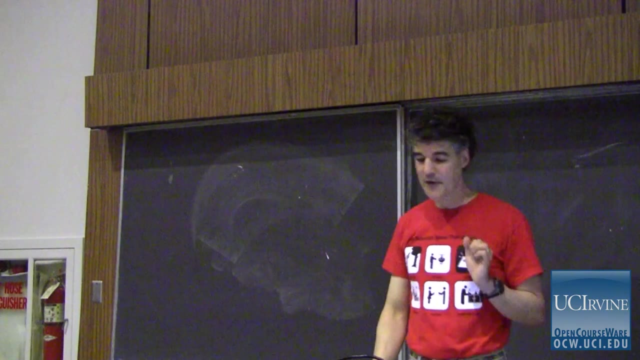 it's easier to see And you can measure the freezing point by cooling it and then seeing when it suddenly levels off, And you can get that quite accurately And then you can tell: gee, the freezing point was lowered by a certain amount. 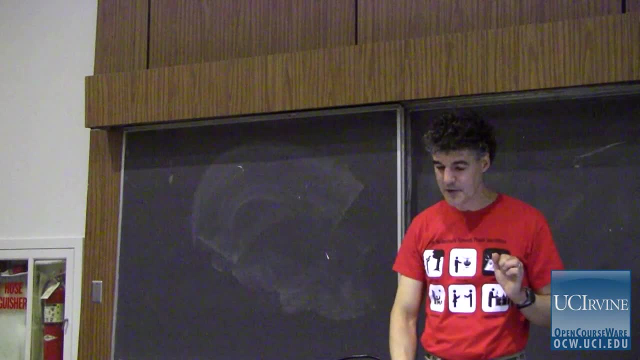 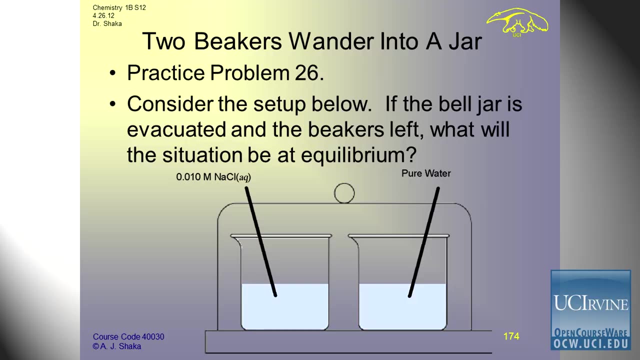 Now we can see this effect of the lower vapor pressure, of a solution in this practice problem. Well, let's consider this setup. We have a bell jar. There's a solution in it. It's vacuum, No air, And we have a solution. 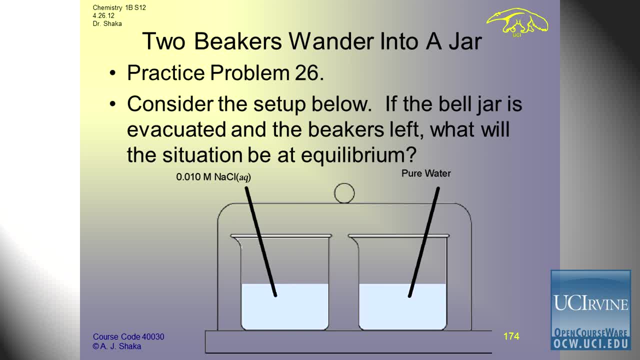 that's 10 millimolar sodium chloride here And we have a solution that's pure water here And we have them in a thermostat at constant temperature. Thermostat's important because we may need to supply some heat energy for things to happen. 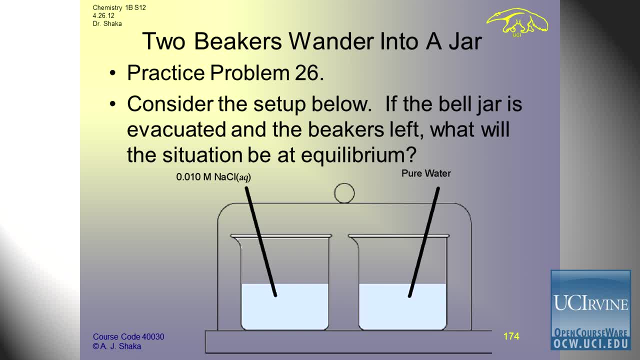 It's not insulated. The question is, what do we see at equilibrium? Who wants to take a guess? Yes, Exactly right. All the pure water will magically end up over here, And if it would happen quickly, this would be a great magic trick. 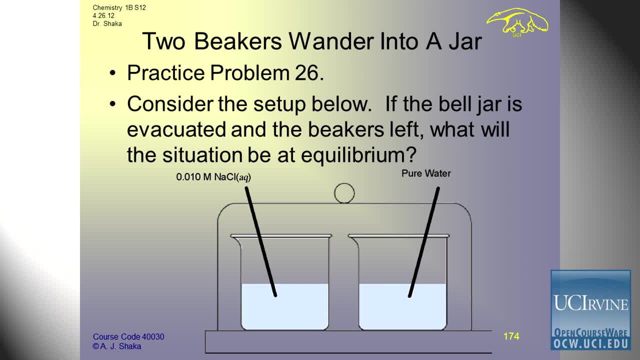 Since you can't see the salt. But unfortunately it happens quite, quite slowly Because we have to wait for the darn water molecules to come up here and fiddle around and come over here. But the pressure pushing up here is always slightly less. 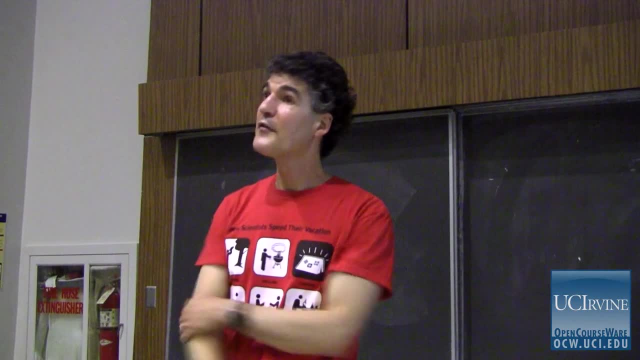 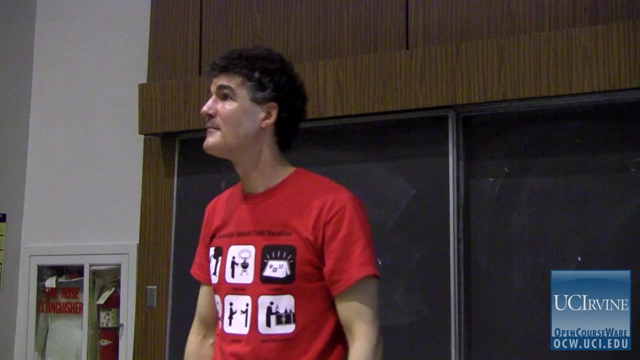 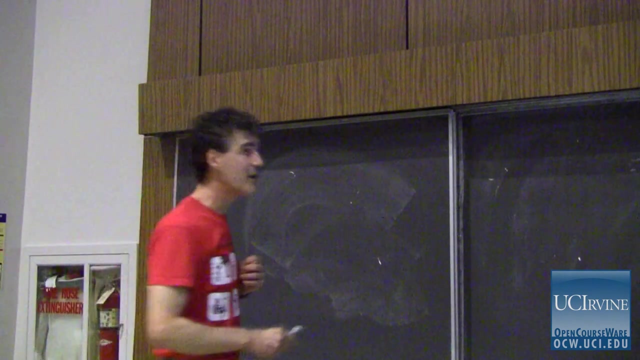 than the pressure pushing up here, And so if I'm pushing on something and you're pushing me, and I'm pushing you, and I'm pushing harder, you go backwards. That's what happens, And so all the water ends up over here And you end up then with 0.05 molar water. 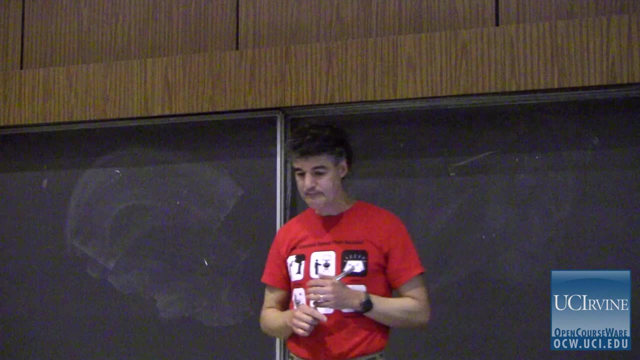 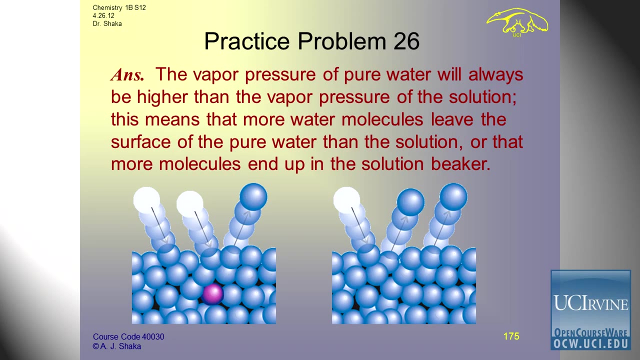 in the other beaker And you can see- I've tried to draw something here- where on this side there's an occasional guy here And what it means is there's less guys coming up off the surface. Maybe this guy attracts them at the last minute. 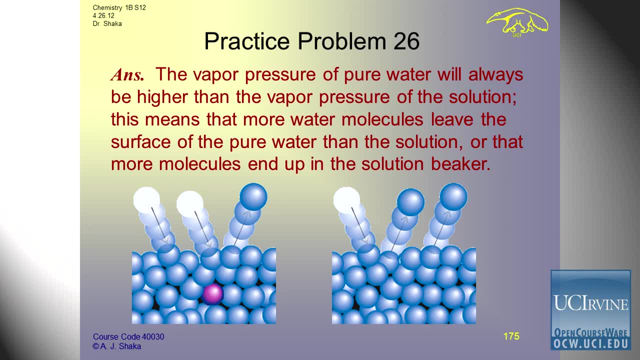 and says: don't go, don't go, I'll change my ways. It's like people: They wait until it's too late, Bye. And then these guys are giving more because there's nobody here saying anything. And so, over time, 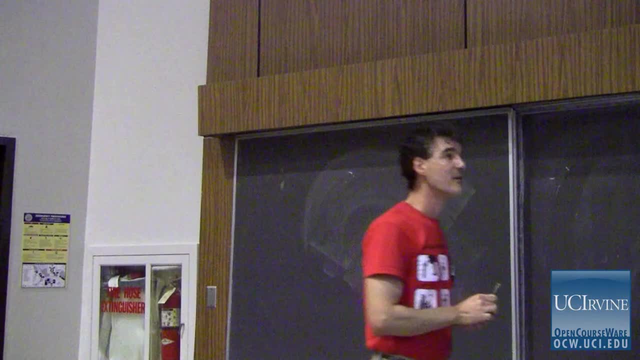 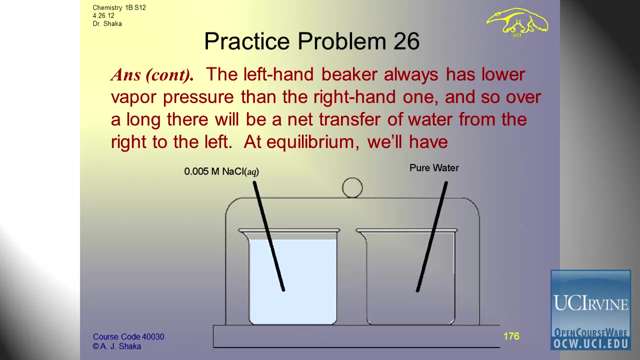 more comes out of the right and ends up on the left over there, And so here's what happens, And so here's what we get. I've never tried the experiment. This particular problem is at least 35 years old, because it was on an AT test. 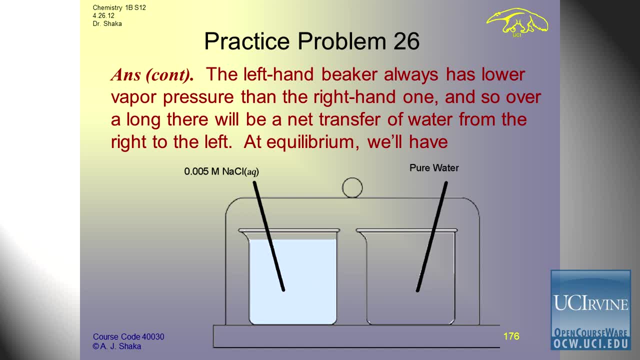 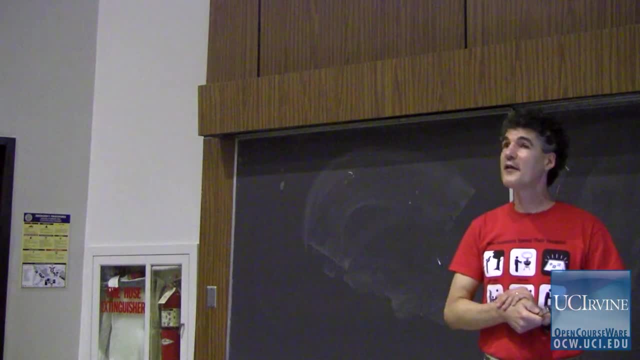 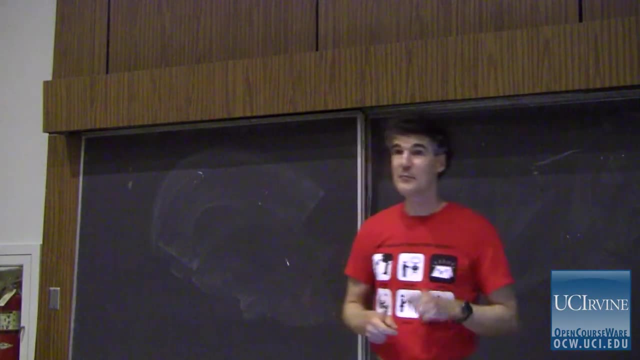 I took with a slide rule. It's that old, So this is an oldie but goodie. But I've never tried the experiment. I've always wanted to try it and just get two beakers and then sit there and also see how long it takes. 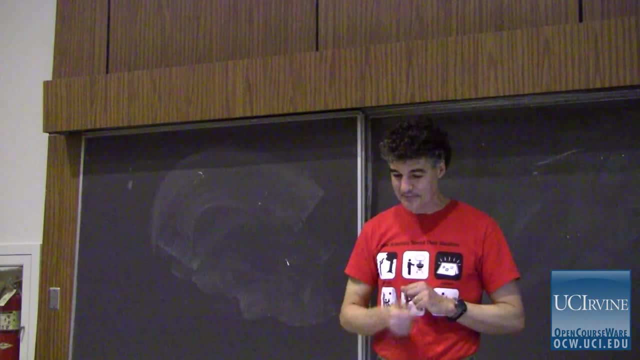 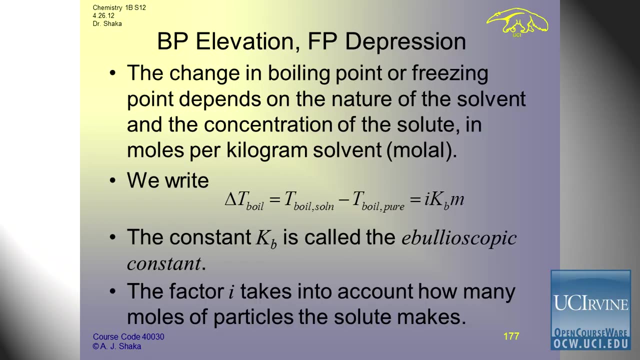 But I never had the time to do it. Okay, The change in boiling point or freezing point depends on the kind of solvent and the concentration of the solute in molal, But it doesn't depend on the kind of solute, at least not much. 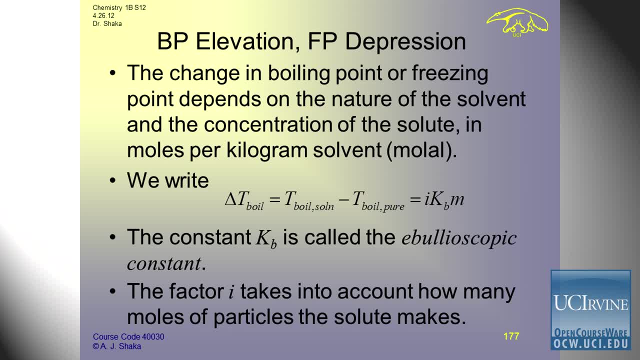 And so we write this equation: The change in boiling point is equal to this factor. I times the boiling point, what Chang calls the boiling point elevation. constant times the molality, And I is a factor. that means, if you've got sodium chloride, you make two particles instead of one. 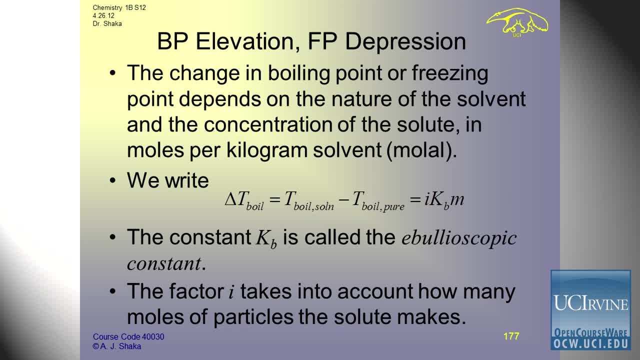 So for sodium chloride I is two, because you get twice as many particles And it has to do with the number of particles in the thing. The correct name for KB is the ebuloscopic constant, And after you say that a few times you'll see why they changed. 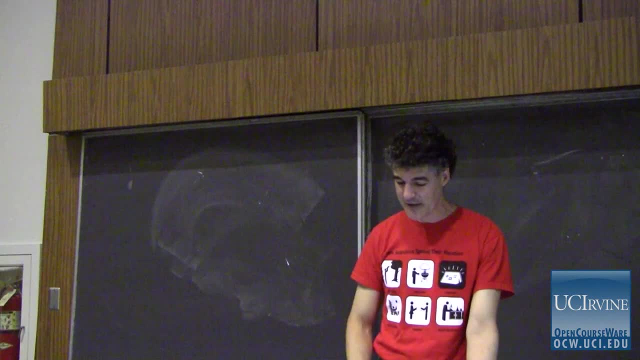 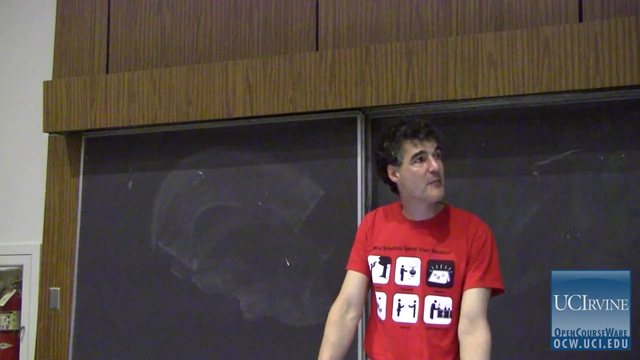 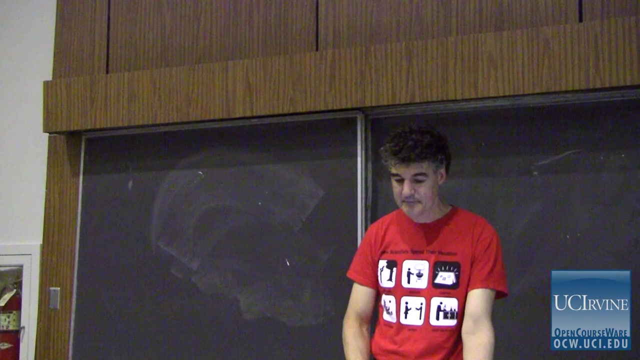 the name to the boiling point, elevation constant, But anyway that will clear your sinuses out. And the factor I takes into account how many moles of particles the solute makes, Not the same for every kind of material, obviously Freezing point depression. 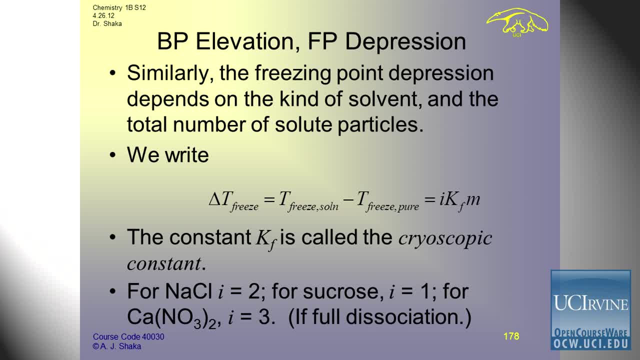 is the same thing. It depends on the kind of solvent and the total number of solute particles. And we write the same kind of equation, exactly the same, And this constant K only depends on the solvent. When you're looking up K for boiling or freezing, 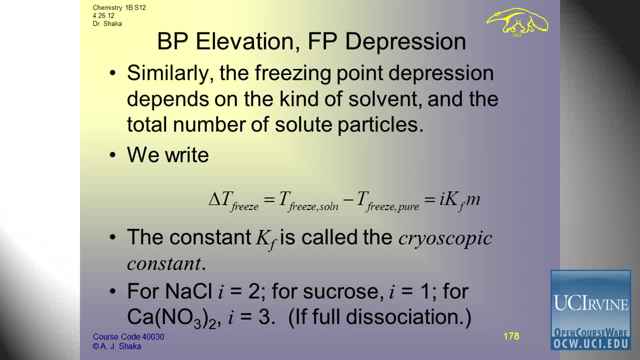 just think what's boiling or freezing- Mostly the solvent, And so that's all. it depends on You list it for that. And the constant KF is called the cryoscopic constant. You may have heard of cryopreservation If you get a fatal disease. 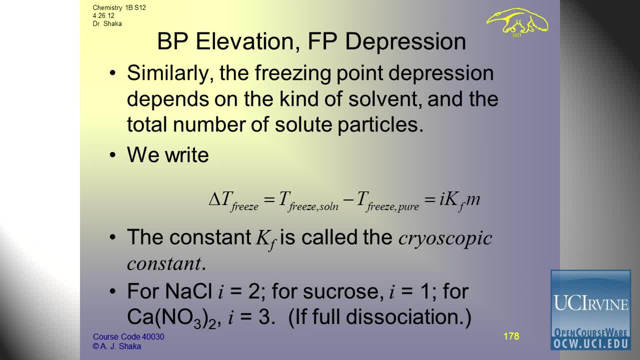 and some guy offers to freeze you in liquid nitrogen and then they're going to warm you back up when the disease is got a cure And that won't work, You just die. Yeah, And in fact a guy in Arizona was doing this in his garage. 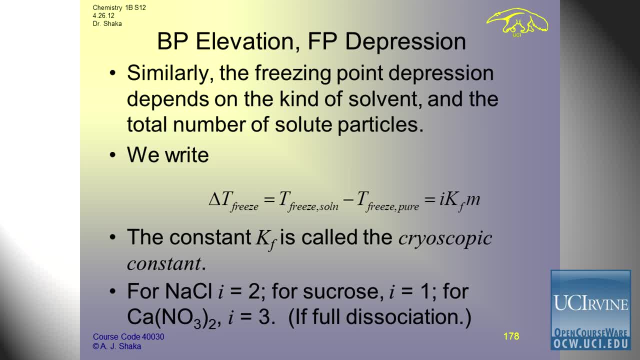 He had at least six or eight suckers whom he'd frozen and their relatives would come by and check out the giant thing full of liquid nitrogen. And one time he ran low on liquid nitrogen. They missed the delivery He was going. oh God. 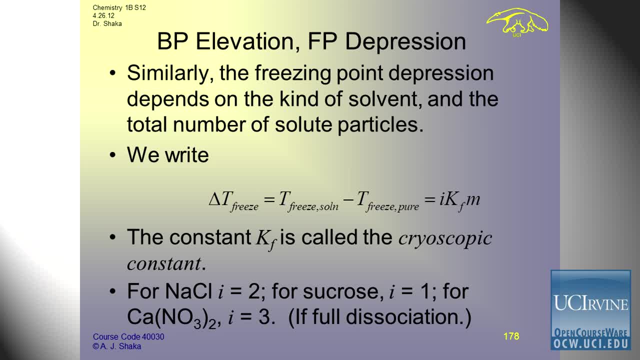 what am I going to do? What am I going to do? And so he just let one of the guys warm up And when the relatives weren't there, and then he puts in more liquid nitrogen later. Now you're really dead. if there weren't any questions. The other guys went to court- some of the relatives of the frozen man- and said: you know it's costing too much to keep feeding the old guy liquid nitrogen. Judge, can't you declare him dead, Legally dead, Which the judge did? 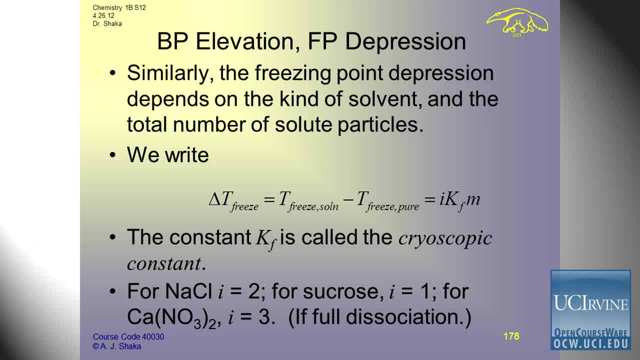 He said: look, it meets all the legal requirements, I'm a lawyer, The guy's dead, And so they turned him off, And so that it's not a good option to freeze yourself, unless you can somehow control what's going to happen after. 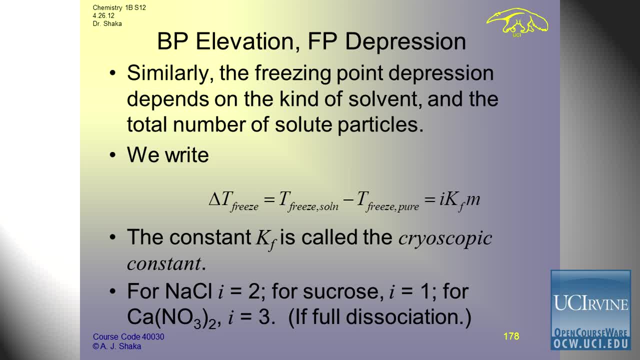 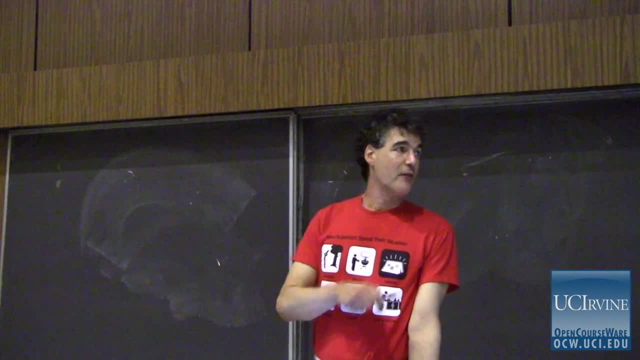 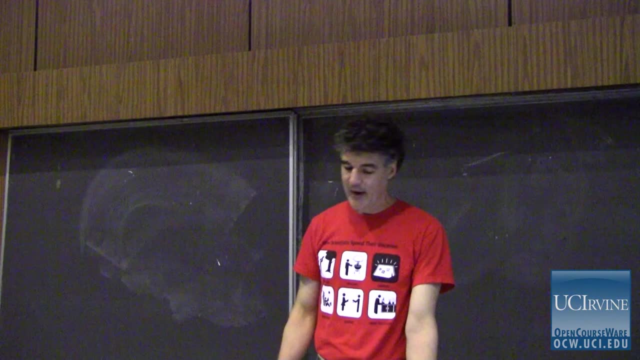 which pretty much you cannot. Okay, for sodium chloride, I is two. For sucrose, I is one, And for calcium nitrate, where we'd get three ions. if it all dissolves and dissociates, I would be three. Pretty simple. 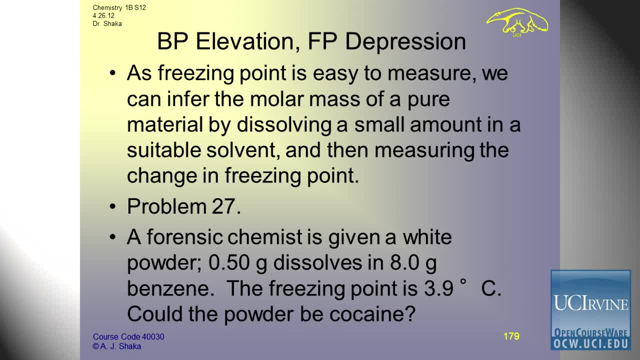 Freezing points pretty easy to measure And if we can measure the freezing point depression, we can tell what the molar mass of a pure material is. Now, if we can find something that dissolves in and measure the change in freezing point, 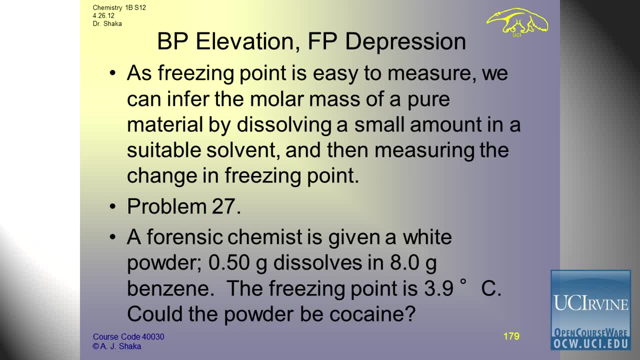 which is dead easy to do. we can figure out what it is, And so let's go to a crime scene. Well, not much of a crime scene. Forensic chemist is given a white powder. Half a gram of it dissolves. 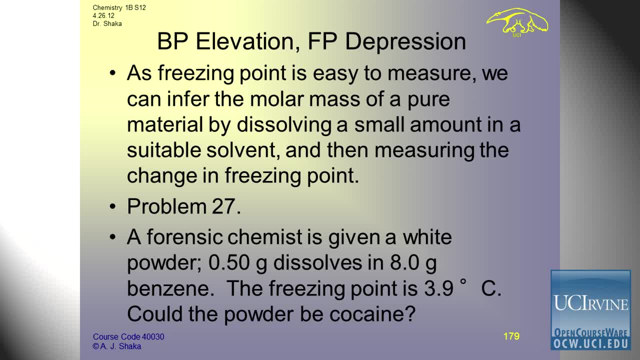 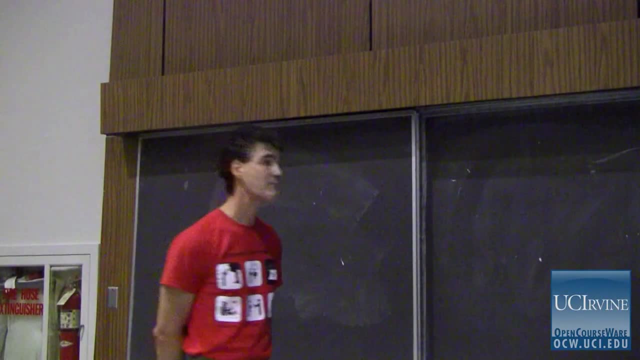 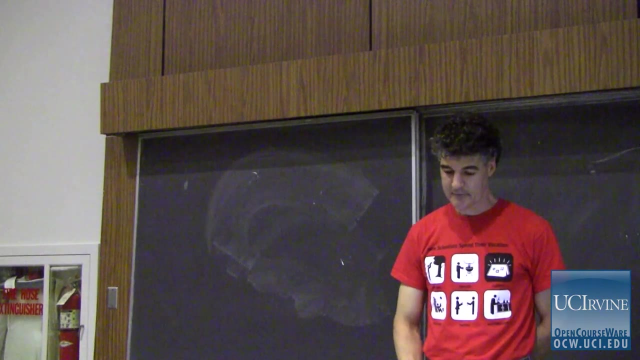 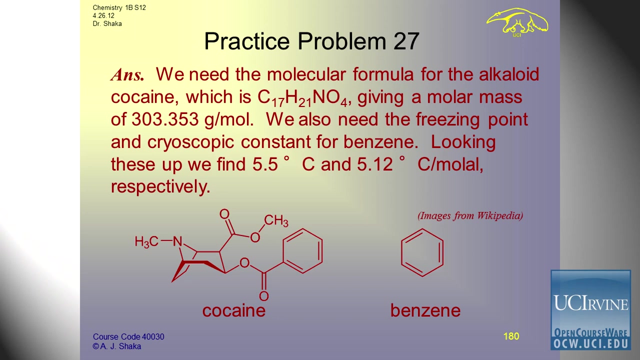 in eight grams of benzene, The freezing point is 3.9 degrees Celsius. Could the powder be cocaine? That's the question. Okay, Lots of things are white powders. Let's have a look. You can kind of see why cocaine. 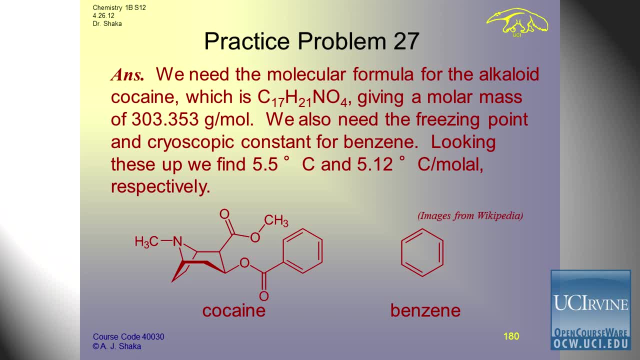 might dissolve in benzene, because they both have these benzene type structure here. And then cocaine has this very interesting structure here that the plant makes. Usually plants make these compounds not for fun. They say: why does the plant make all these things? 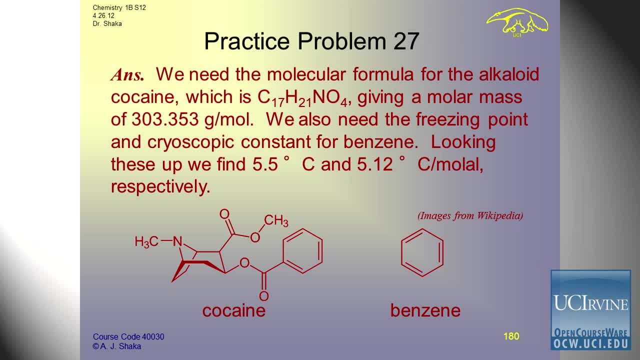 They make these things to keep the bugs off them, Because if you're a plant, you can't move And these bugs are crawling all over you and they're drilling in And if you're going to survive you have to use chemical warfare. 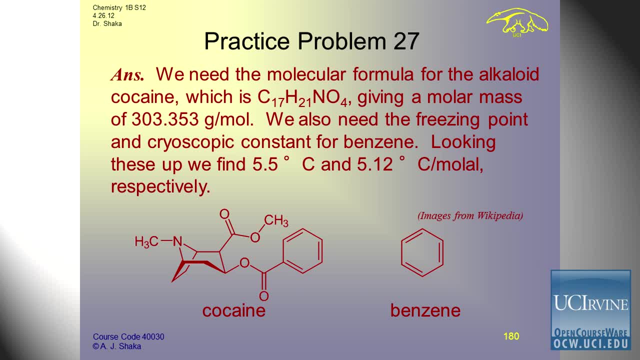 You look at eucalyptus, You start chewing the eucalyptus leaves. Ah, kind of burns my mouth. Well, it burns the insect's mouth too, And that means they stop eating, They don't go wild. You plant lettuce, they go wild, And so you have to do the chemical warfare, because otherwise they'll completely decimate your crop, Or you have to do something You can pick them off by hand. That gets old Because they're relentless and they come at night. 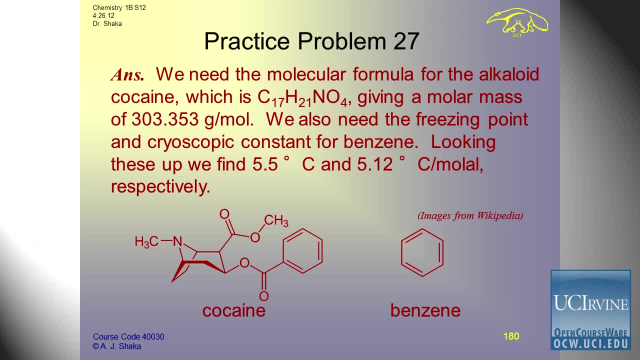 and slugs crawl over everything and wreck it Right. So usually you spray, And then the question is: that has an environmental impact. But presumably this has been made to keep off some bug, Maybe instead of burning the bug's mouth with eucalyptol. 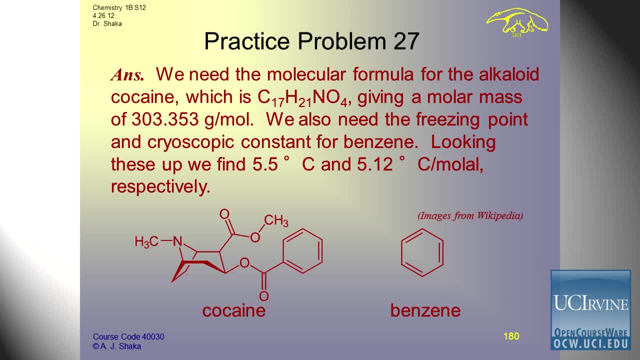 the bug eats some of the coca leaves and then it says: what was I doing, What was I trying to do here? And just kind of flies off, Doesn't eat anymore and the plant survives, Who knows. There are a lot of different strategies. 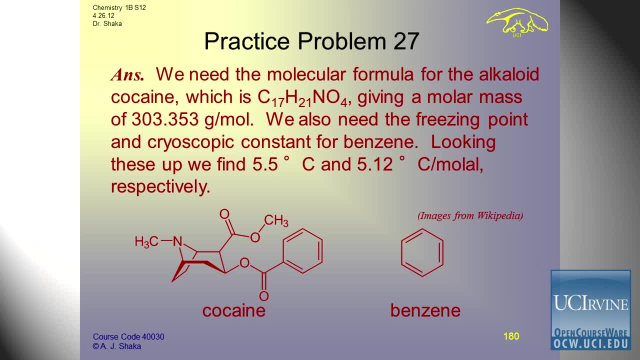 plants use. Well, if we look up the molar mass of this molecule, it's 303.353 grams per mole, And if we look up the freezing point of benzene, it's 5.5 degrees C, A little bit higher than water. 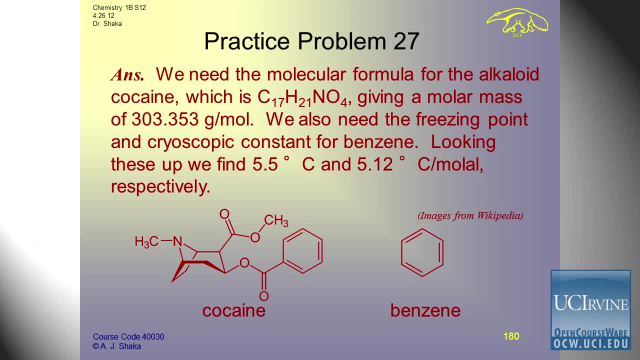 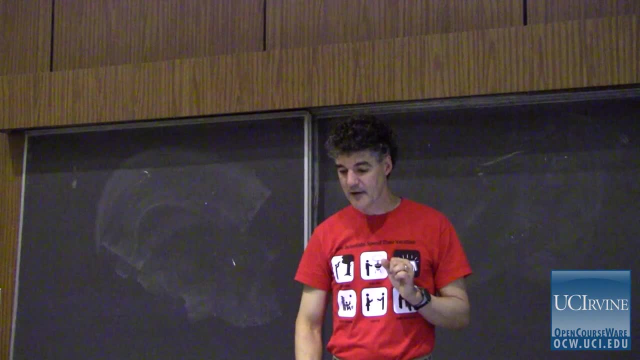 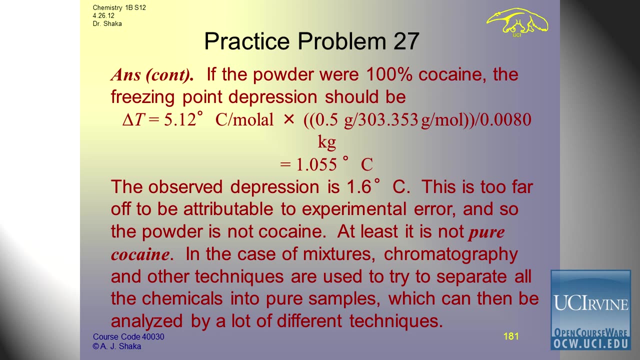 And the cryoscopic constant is 5.12 degrees C per mole out. That's how the units have to work out. But let's have a look then at whether it can work If the powder were 100% cocaine, which is the real problem here. 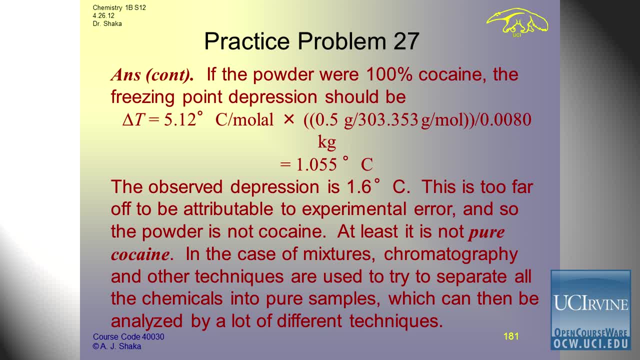 then the freezing point should be the cryoscopic constant times. the 0.5 grams convert to moles and then divide by 0.008 kilograms, which is 8 grams, And the freezing point depression should be 1.55 degrees C. 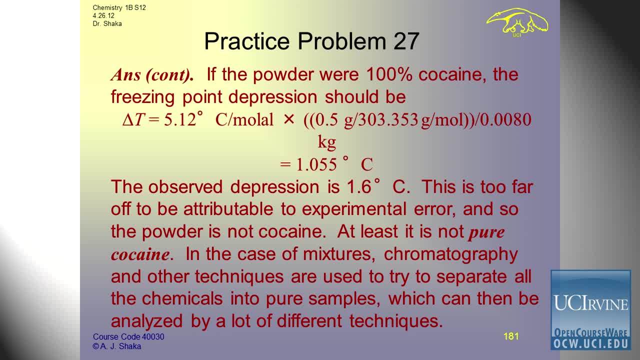 The observed freezing point depression is 1.55.. The observed freezing point depression is 1.6.. Way off. So our conclusion is: it's impossible that that's 100% cocaine. But sadly, hardly anything is going to be 100% of the most valuable compound. 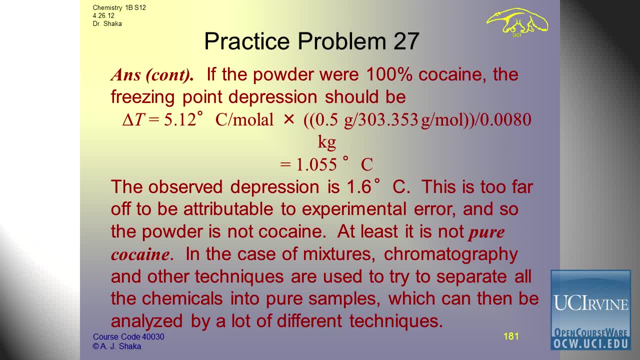 Usually some other things have been added And you don't know then if the other things are lowering the freezing point by a different amount. In fact, what you have to do with the sample first is separate it using chromatography or other means until you get things that you see are pure. 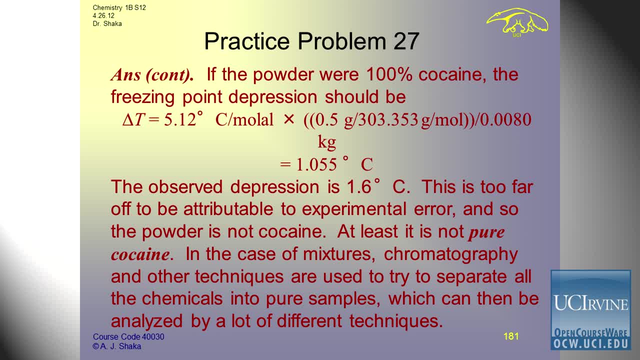 You can just take a tiny spot of the material, You can put it on a silica sheet and you can put solvent. The solvent percolates through and if it's one material, you have one spot that moves. If it's more than one material, 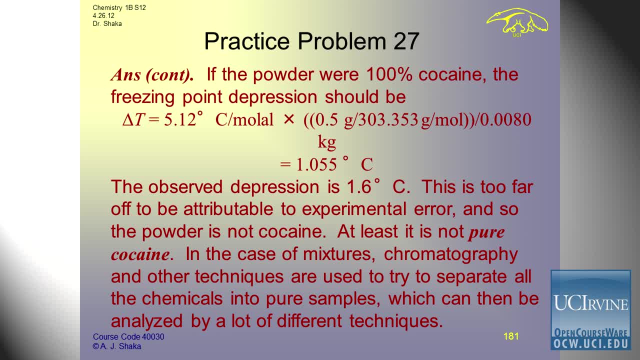 you get different spots. That's called thin layer chromatography. You only need a tiny amount to see that it's not pure. Yes, I'm a little confused about how to observe the depression in the 1.6 degrees Celsius, while the change in temperature. 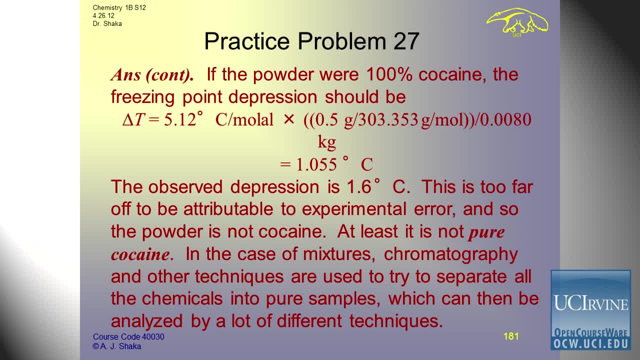 says 1.05 degrees, Because benzene freezes at 5.5 and what the forensic chemists found is, when they put this stuff in, it froze at 3.9, and that's 1.6 degrees difference. So what I'm saying is: 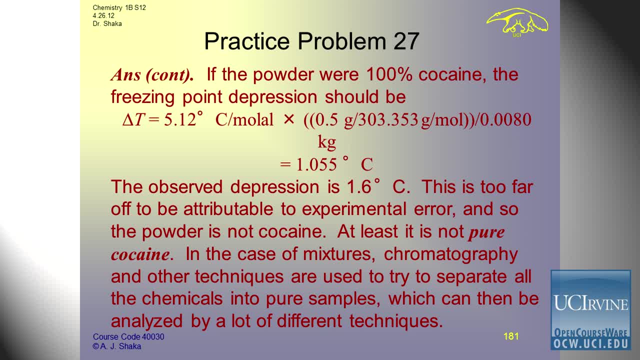 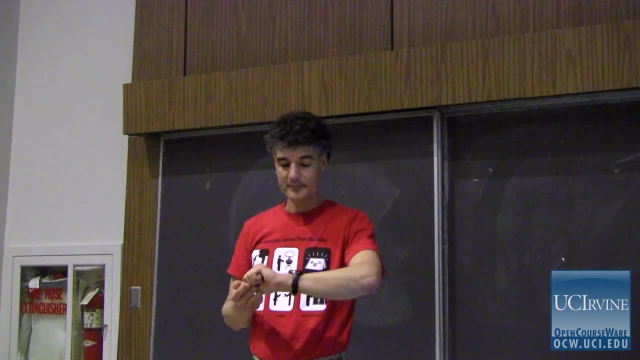 it can't be that molar mass. All you know is it's not that molar mass. You don't know. it's not some other drug, Okay, But it's not that drug, You would then try some other ones, Okay. 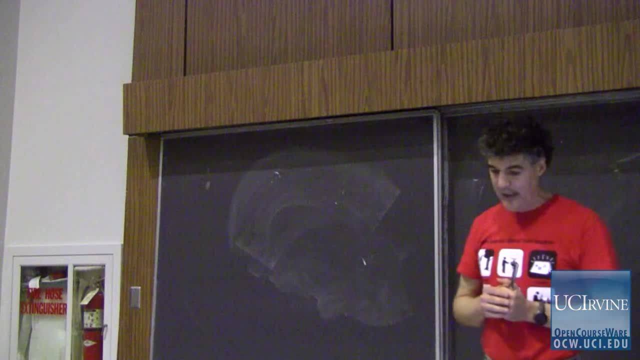 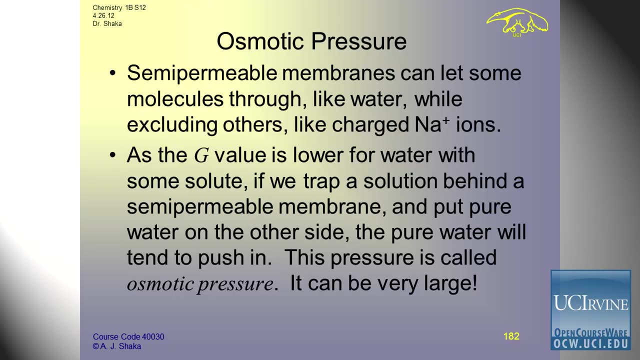 All right, Let's do one more thing and then we'll quit. By the way, you'd never do it this way If you go to a crime lab, they don't. They have mass spectrometers and they'll tell you. 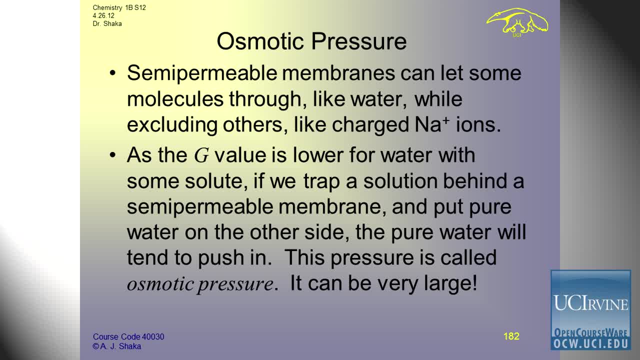 you know. or the Olympic testing when they find one extra molecule of testosterone. I mean, that's really interesting chemistry, the sort of cloak and dagger to find out who's cheating. The short answer is: everybody's cheating in certain sports. They just haven't been caught. 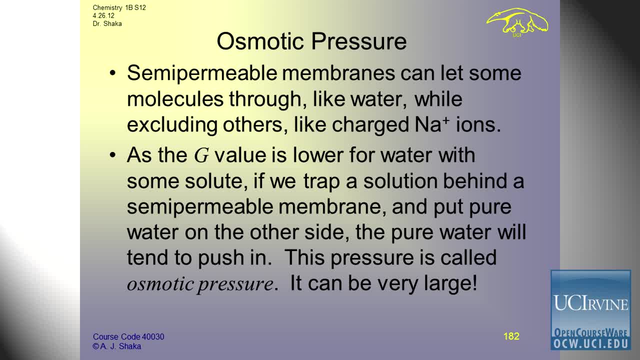 Okay, If we have a semi-permeable membrane and we can let through some molecules like water, while excluding other ones like charged ions. you might think how do you do that? But in fact that's what our cells do all the time. 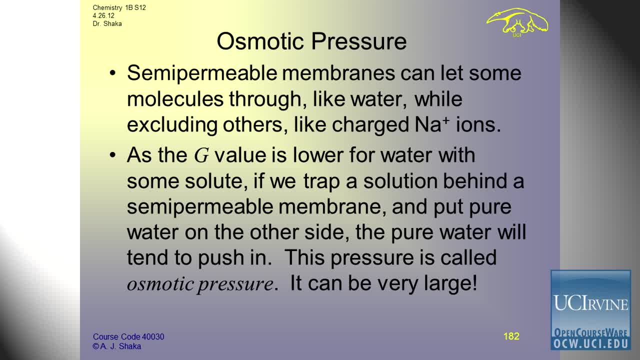 They let through potassium into the interior of the cell and the sodium stays in the plasma of your blood. So there are membranes that do that. Well, if we have an artificial membrane like that, the G value is lower for water with some solute. 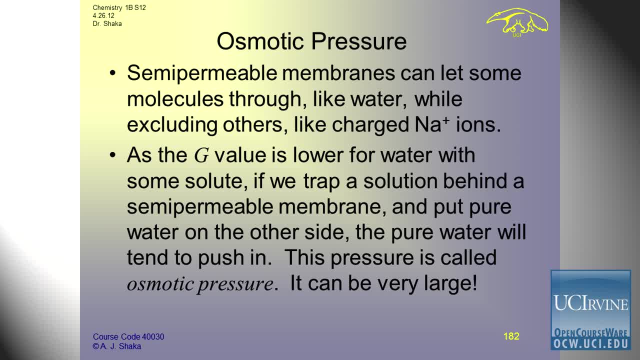 because, we saw, its vapor pressure is lower. Therefore, if we trap a solution behind a membrane and put pure water on the other side, then the pressure can be huge And the water will tend to rush in and swell the stuff up And you can see this effect. sometimes people who eat too much salt look very puffy for a while and their kidneys work overtime. Get rid of all that stuff Back to normal, And then another bag of Doritos or something and you're back to where you started. Don't eat salt. It's not a good idea. Try to steer clear of it and you'll get just the right amount. It's like smoking: You don't need to worry about having a minimum amount to be healthy, And this pressure then will pick up this next time. 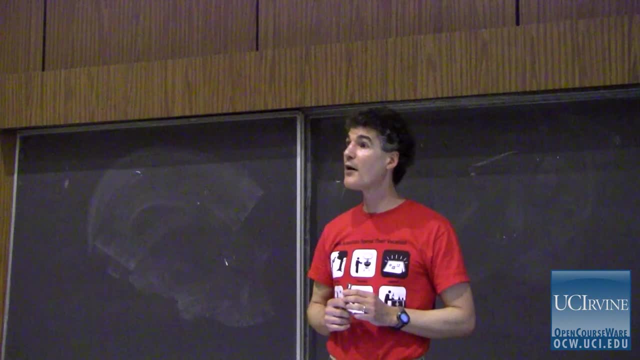 when we talk about desalinization of water by reverse osmosis. 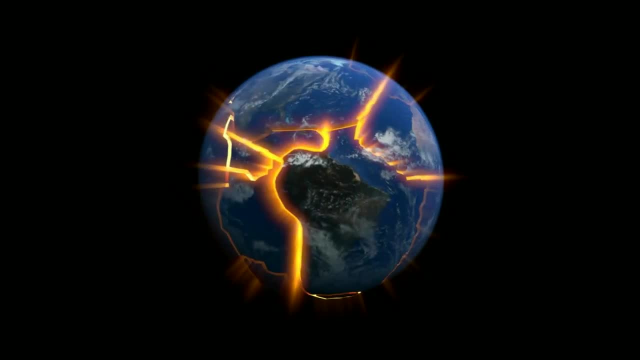 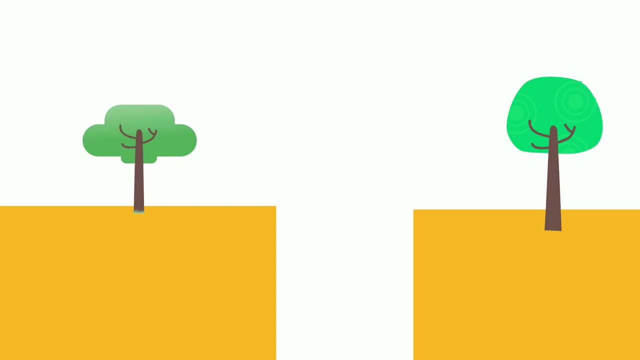 Welcome to MooMooMath and Science and different types of convergent boundaries. Convergent boundaries occur when tectonic plates move towards each other and strike one another. If you look at this map of the major plates, you can notice several that are convergent boundaries.